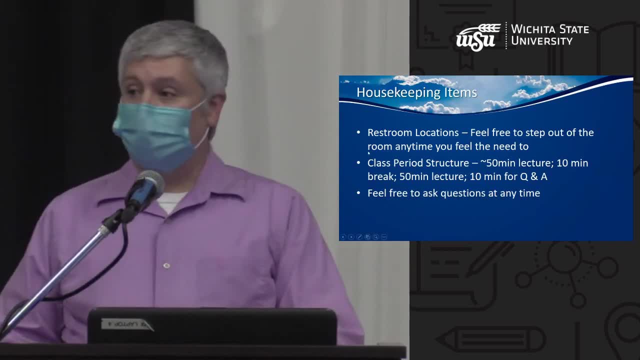 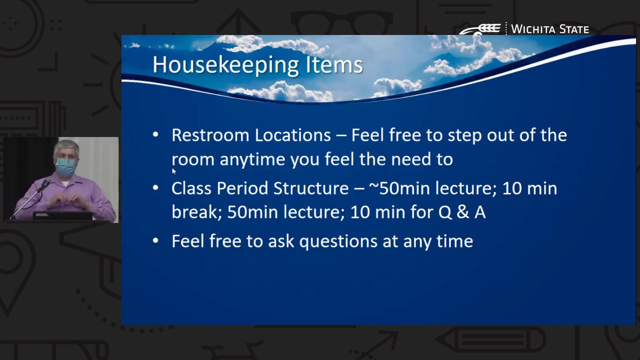 Number four of Intro to Meteorology: I presume that by this point everybody has at least gone to one of the two sessions before. so hang on for just a second while I go through them all while touching my face over and over again. Number five of Intro to Meteorology: I presume that by this point everybody has at least gone to one of the two sessions before. so hang on for just a second while I go through them all while touching my face over and over again. 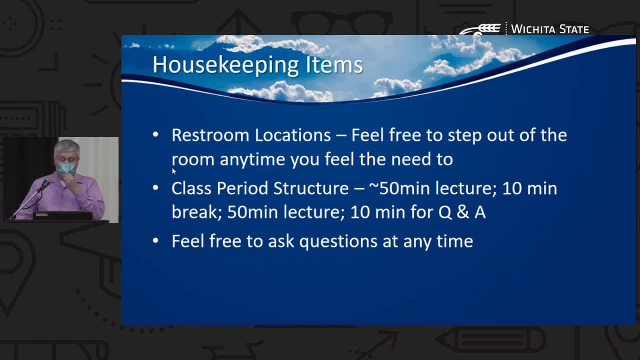 Number six of Intro to Meteorology. I presume that by this point everybody has at least gone to one of the two sessions before. so hang on for just a second while I go through them all while touching my face over and over again. Number seven of Intro to Meteorology: I presume that by this point everybody has at least gone to one of the two sessions before. so hang on for just a second while I go through them all while touching my face over and over again. 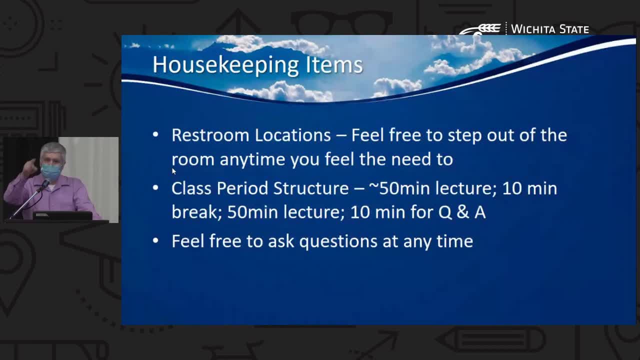 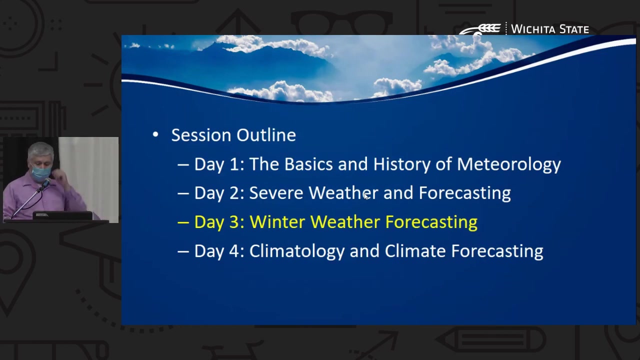 Number eight of Intro to Meteorology: I presume that by this point everybody has at least gone to one of the two sessions before. so hang on for just a second while I go through them all while touching my face over and over again. Number nine of Intro to Meteorology: I presume that by this point everybody has at least gone to one of the two sessions before. so hang on for just a second while I go through them all while touching my face over and over again. 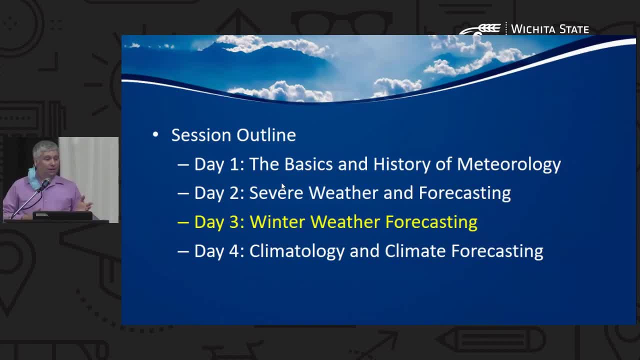 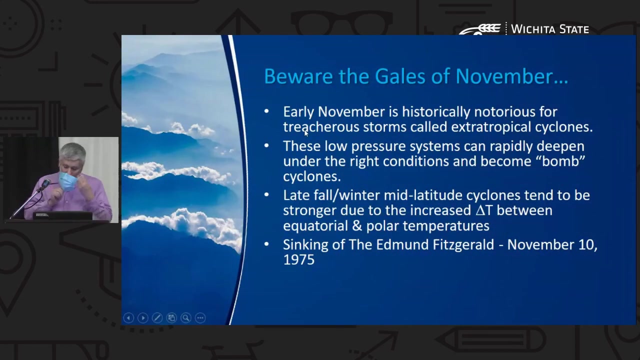 Number ten of Intro to Meteorology: I presume that by this point everybody has at least gone to one of the two sessions before. so hang on for just a second while I go through them all while touching my face over and over again. Number eleven of Intro to Meteorology: I presume that by this point everybody has at least gone to one of the two sessions before. so hang on for just a second while I go through them all while touching my face over and over again. 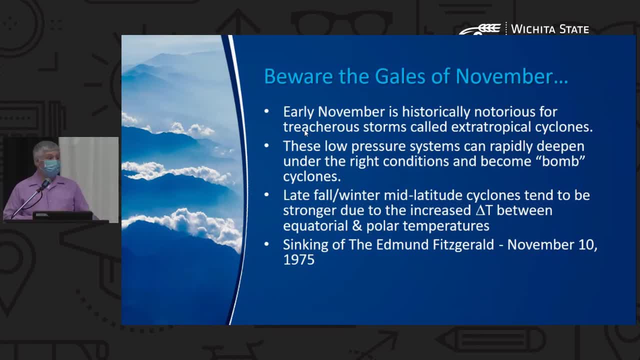 Number twelve of Intro to Meteorology. I presume that by this point everybody has at least gone to one of the two sessions before. so hang on for just a second while I go through them all while touching my face over and over again. Number thirteen of Intro to Meteorology: I presume that by this point everybody has at least gone to one of the two sessions before. so hang on for just a second while I go through them all while touching my face over and over again. 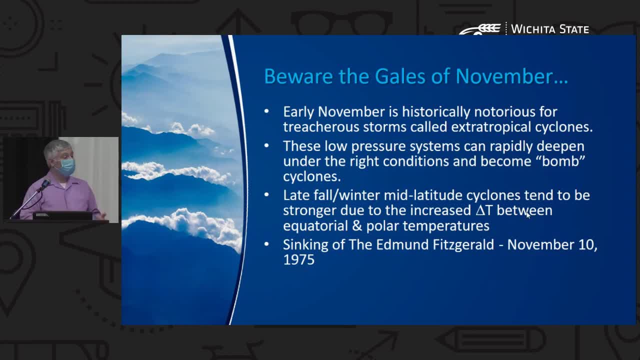 Number fourteen of Intro to Meteorology: I presume that by this point everybody has at least gone to one of the two sessions before. so hang on for just a second while I go through them all while touching my face over and over again. Number fifteen of Intro to Meteorology: I presume that by this point everybody has at least gone to one of the two sessions before. so hang on for just a second while I go through them all while touching my face over and over again. 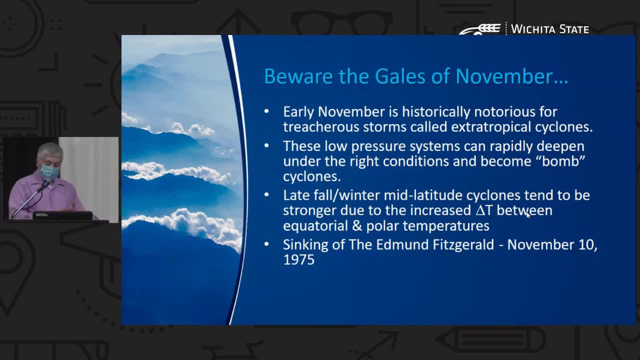 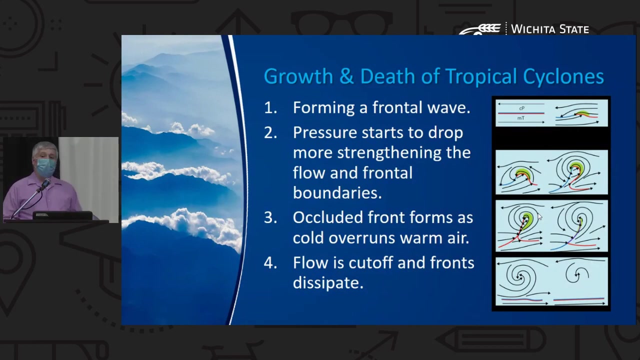 Number sixteen of Intro to Meteorology. I presume that by this point everybody has at least gone to one of the two sessions before. so hang on for just a second while I go through them all while touching my face over and over again. Number sixteen of Intro to Meteorology: I presume that by this point everybody has at least gone to one of the two sessions before. so hang on for just a second while I go through them all while touching my face over and over again. 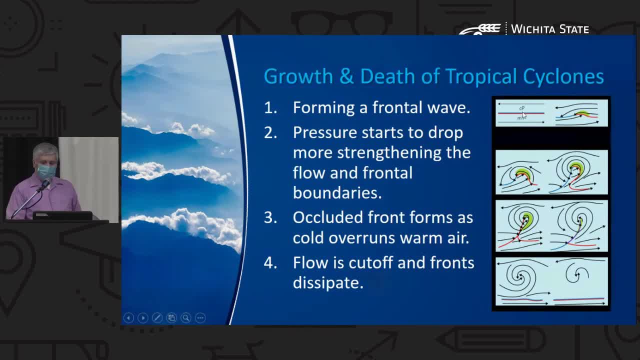 Number sixteen of Intro to Meteorology. I presume that by this point everybody has at least gone to one of the two sessions before. so hang on for just a second while I go through them all while touching my face over and over again. Number sixteen of Intro to Meteorology: I presume that by this point everybody has at least gone to one of the two sessions before. so hang on for just a second while I go through them all while touching my face over and over again. 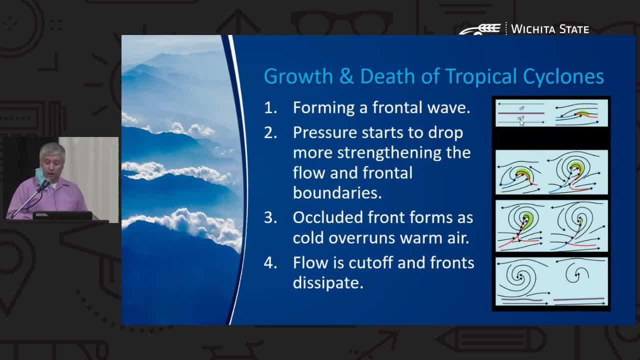 Number sixteen of Intro to Meteorology. I presume that by this point everybody has at least gone to one of the two sessions before. so hang on for just a second while I go through them all while touching my face over and over again. Number sixteen of Intro to Meteorology: I presume that by this point everybody has at least gone to one of the two sessions before. so hang on for just a second while I go through them all while touching my face over and over again. 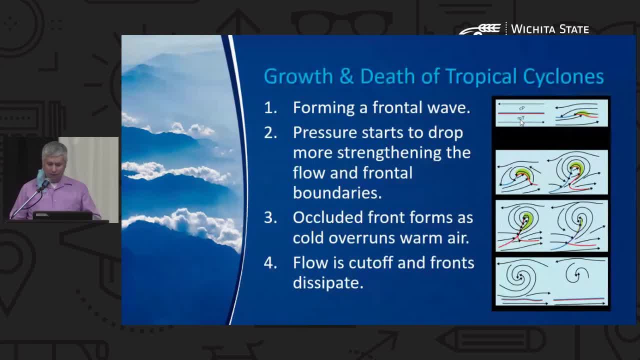 Number sixteen of Intro to Meteorology. I presume that by this point everybody has at least gone to one of the two sessions before. so hang on for just a second while I go through them all while touching my face over and over again. Number sixteen of Intro to Meteorology: I presume that by this point everybody has at least gone to one of the two sessions before. so hang on for just a second while I go through them all while touching my face over and over again. 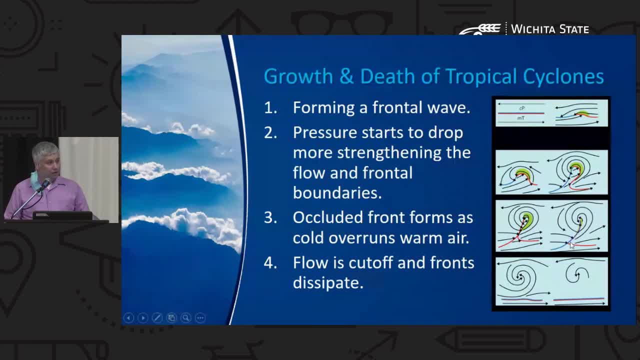 Number sixteen of Intro to Meteorology. I presume that by this point everybody has at least gone to one of the two sessions before. so hang on for just a second while I go through them all while touching my face over and over again. Number sixteen of Intro to Meteorology: I presume that by this point everybody has at least gone to one of the two sessions before. so hang on for just a second while I go through them all while touching my face over and over again. 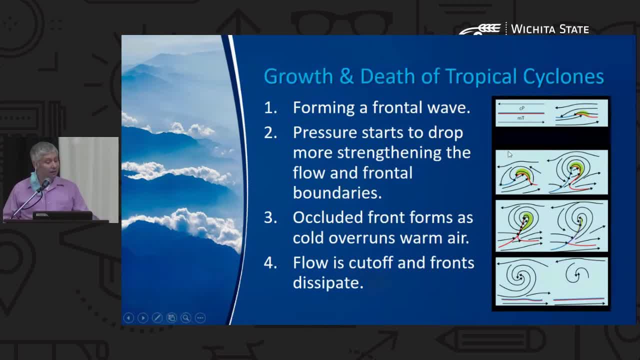 Number sixteen of Intro to Meteorology. I presume that by this point everybody has at least gone to one of the two sessions before. so hang on for just a second while I go through them all while touching my face over and over again. Number sixteen of Intro to Meteorology: I presume that by this point everybody has at least gone to one of the two sessions before. so hang on for just a second while I go through them all while touching my face over and over again. 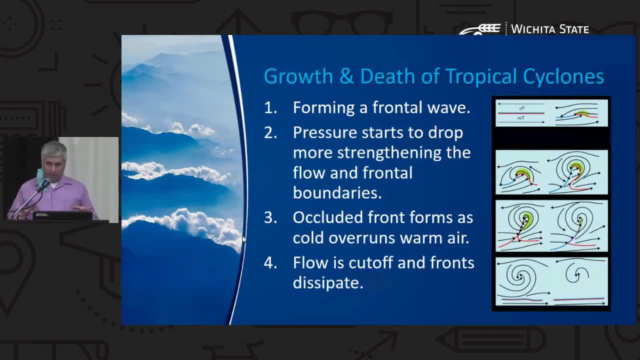 Number sixteen of Intro to Meteorology. I presume that by this point everybody has at least gone to one of the two sessions before. so hang on for just a second while I go through them all while touching my face over and over again. Number sixteen of Intro to Meteorology: I presume that by this point everybody has at least gone to one of the two sessions before. so hang on for just a second while I go through them all while touching my face over and over again. 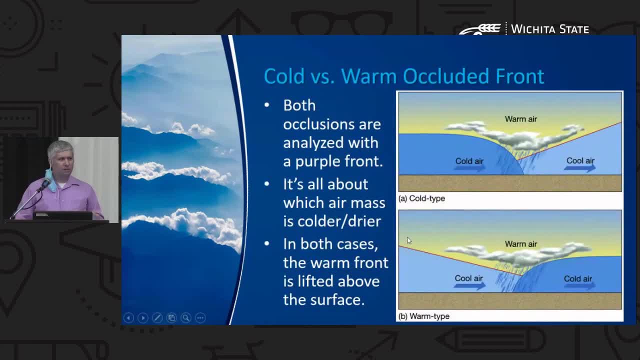 Number sixteen of Intro to Meteorology. I presume that by this point everybody has at least gone to one of the two sessions before. so hang on for just a second while I go through them all while touching my face over and over again. Number sixteen of Intro to Meteorology: I presume that by this point everybody has at least gone to one of the two sessions before. so hang on for just a second while I go through them all while touching my face over and over again. 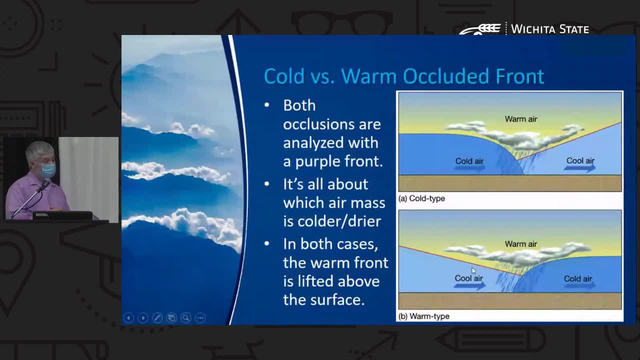 Number sixteen of Intro to Meteorology. I presume that by this point everybody has at least gone to one of the two sessions before. so hang on for just a second while I go through them all while touching my face over and over again. Number sixteen of Intro to Meteorology: I presume that by this point everybody has at least gone to one of the two sessions before. so hang on for just a second while I go through them all while touching my face over and over again. 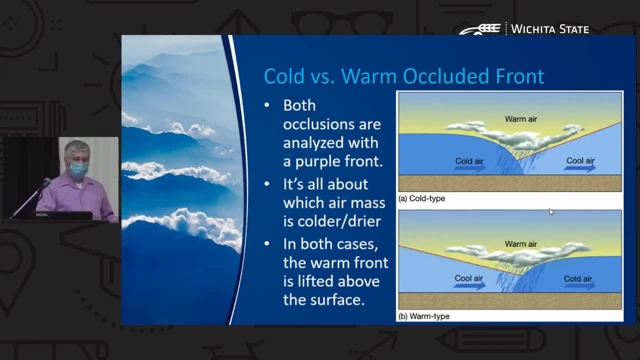 Number sixteen of Intro to Meteorology. I presume that by this point everybody has at least gone to one of the two sessions before. so hang on for just a second while I go through them all while touching my face over and over again. Number sixteen of Intro to Meteorology: I presume that by this point everybody has at least gone to one of the two sessions before. so hang on for just a second while I go through them all while touching my face over and over again. 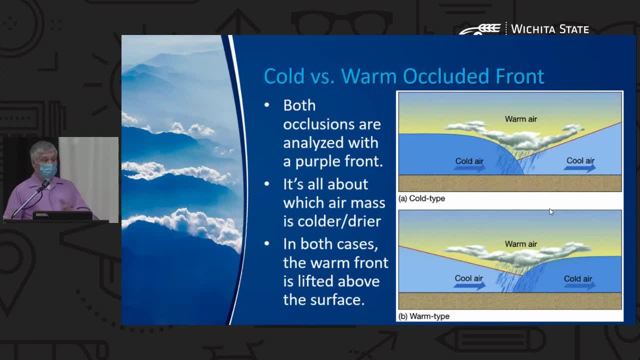 Number sixteen of Intro to Meteorology. I presume that by this point everybody has at least gone to one of the two sessions before. so hang on for just a second while I go through them all while touching my face over and over again. Number sixteen of Intro to Meteorology: I presume that by this point everybody has at least gone to one of the two sessions before. so hang on for just a second while I go through them all while touching my face over and over again. 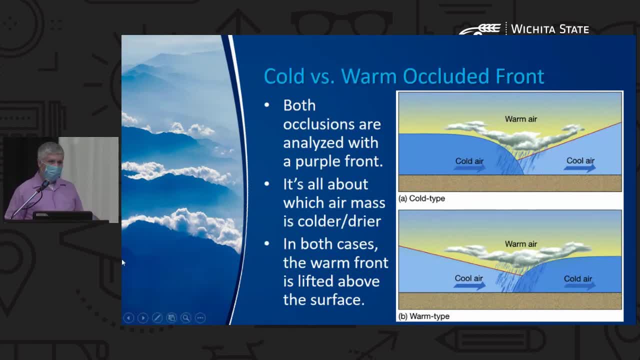 front. that's passing. that kind of defines it Incidentally with an occluded front, and this is actually true of all of our fronts. if you ever want to know what direction the front is moving, all you have to do is look at which side of the frontal boundary. I'm just going to 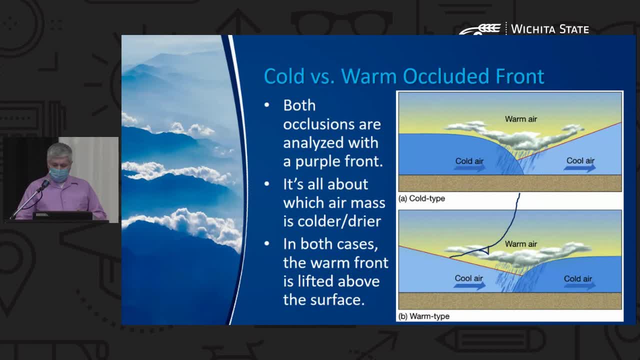 randomly draw one here. what side of that frontal boundary has the barbs on it, And that's always telling you what direction the front is moving. So if you had a warm front drawn like that, there's sort of a my drawing's terrible. but 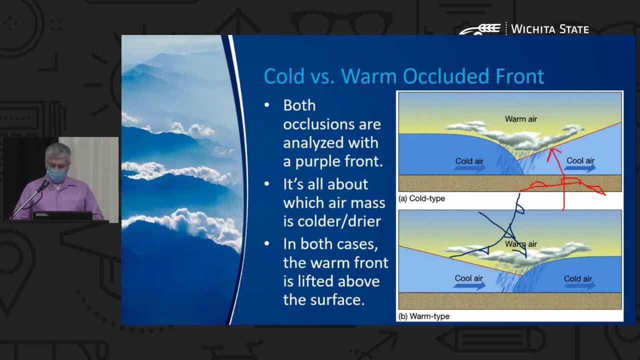 the way the barbs look. that's the way the front is moving at the time, And then you wind up with a stationary front where you see the red and the blue. There's the red. Last week I cut out of drawing that stationary front and instead drew a. 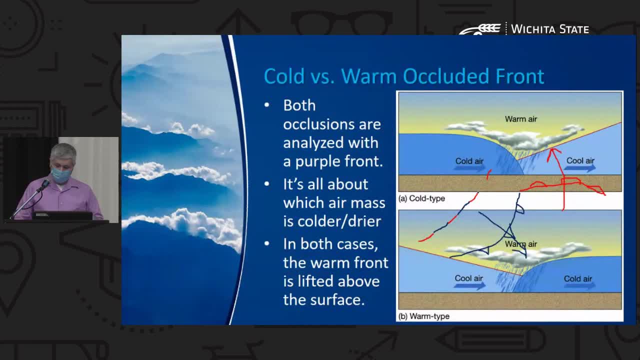 trough line, a low-pressure trough line instead, because drawing the stationary front is a little harder for me to do on the computer. So I'm going to draw a stationary front and I'm going to draw a trough line. and I'm going to draw a trough line instead, because drawing the stationary front is a little harder for me to do on the computer. 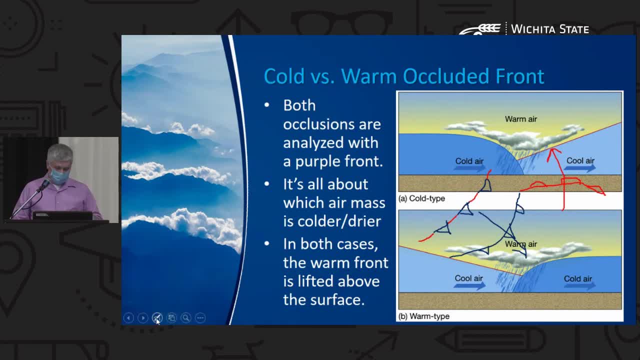 But you wind up with- I'm kind of taking a sidebar here of where I was going with the lecture, but you'll see that as a stationary front And what that means is, yeah, the warm air is trying to push that way, the cold air is trying to push that way, but it's not going either direction. So that's a. 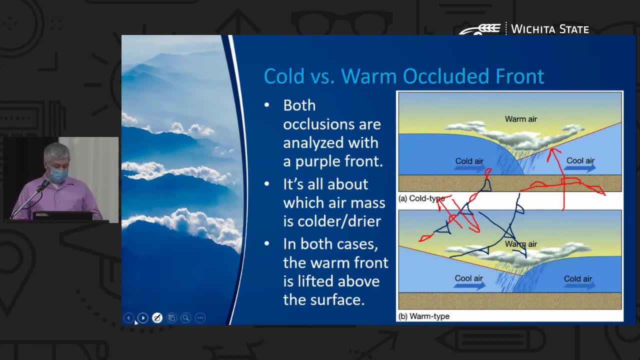 stationary front And then the occluded front looks like this On a map. it's drawn in purple And you'll see that's kind of the triangle, that's sort of the half circle and it's triangle, half circle and that's your occlusion. So that's a little sidebar off of talking about warm and occluded. 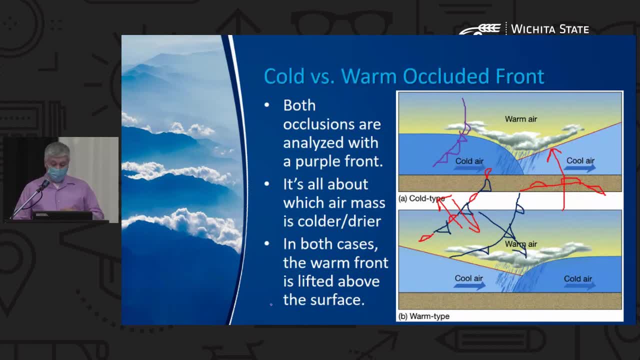 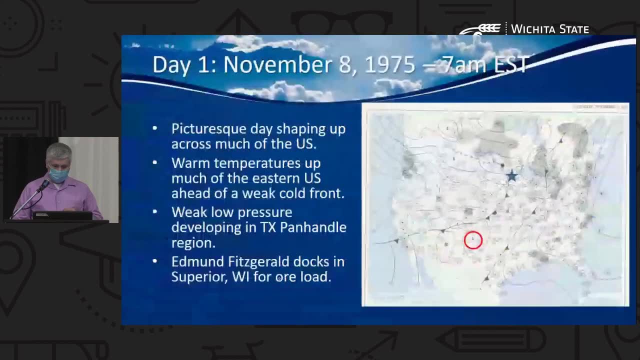 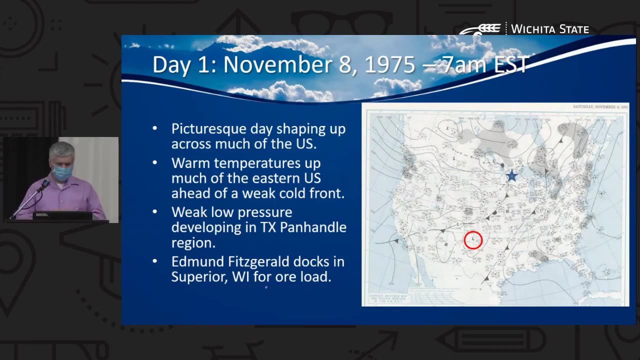 fronts as you're looking at them on the weather map and also knowing what direction those fronts are actually moving at the time. That's how it's drawn up. So back to focusing on the storm that sunk the Edmund Fitzgerald, And this is back in November 8th 1975.. 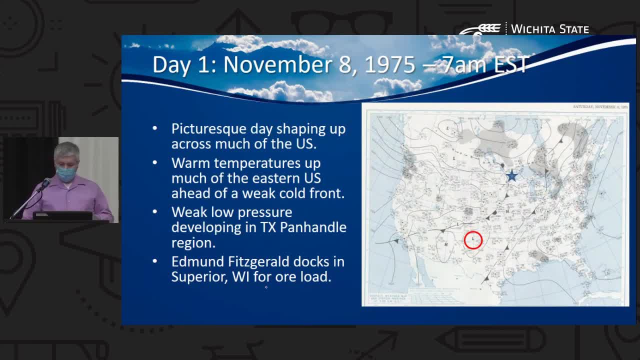 A storm is just starting to form. We can see it down here. You got a low here, low here. This is actually. well. I circled the low that I probably that's more the low that's influencing this event. But anyway, we've got the picturesque day kind of across. 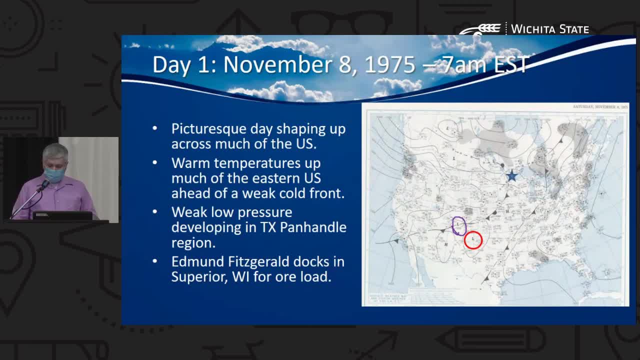 most of the US Got a little bit of overcast, a little bit of rain, snow, moving out of the upper Great Lakes region into Canada. The star here, that is right now where our Edmund Fitzgerald ship is. For those of you who are, 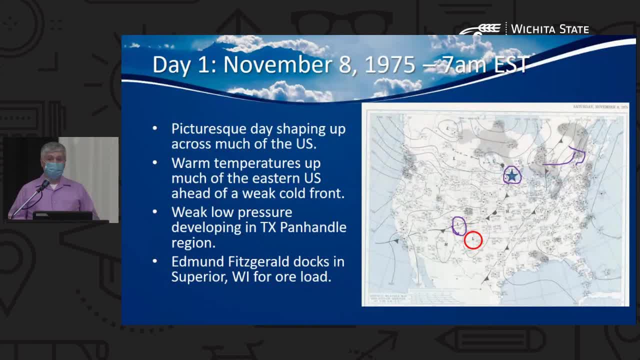 less aware of the Edmund Fitzgerald. it was at the time the largest shipping vessel on the Great Lakes Had been in service for- about trying to do my mental math- about 20 years at this point And it was sort of the pride of the Great Lakes. 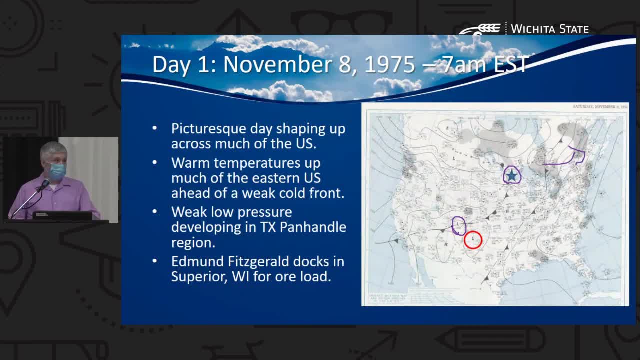 It had been worked really hard and had performed really well in terms of shipping goods across the Great Lakes, in particular the Lake Superior. So Edmund Fitzgerald's docked in Wisconsin, Superior Wisconsin to be exact- And it's awaiting its next shipment of iron ore, which it's going to take across the Great Lakes or across Lake Superior. 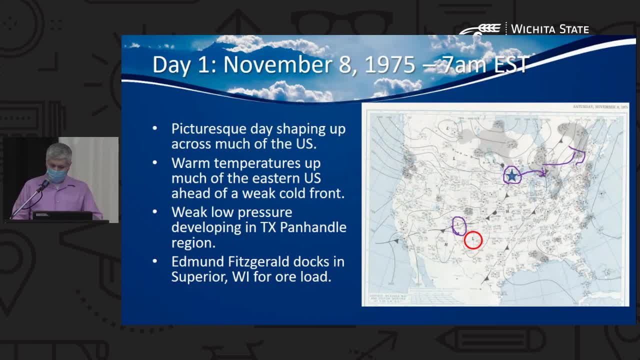 in a path right about like that And we're looking at all of North America, so it's a little hard to see on this, but that's going to be the rough path that actually, if I'm really being accurate, it's a little bit north of that- that the Edmund Fitzgerald's going to take. 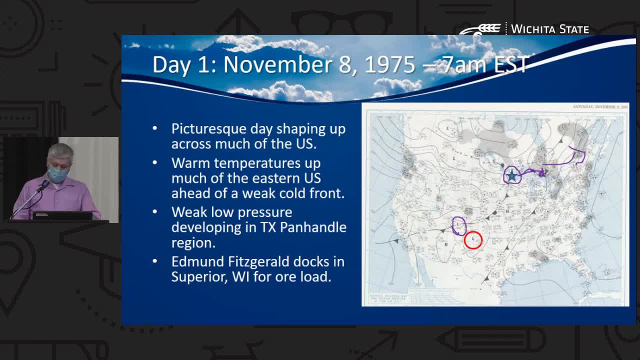 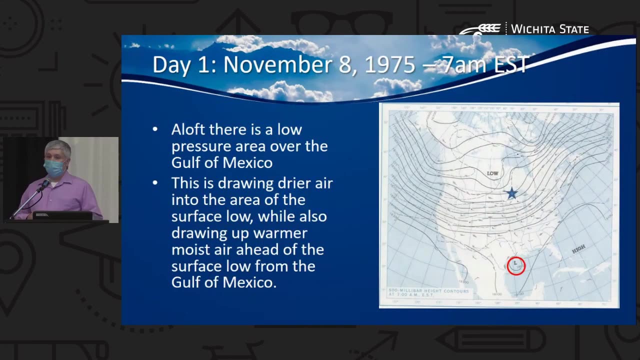 So we've got some got this weak low pressure system here, an even weaker low right there as well, So we have some low pressure developing If we look aloft, and this is actually in this class. this is the first time we've taken a look at a weather map above the surface. 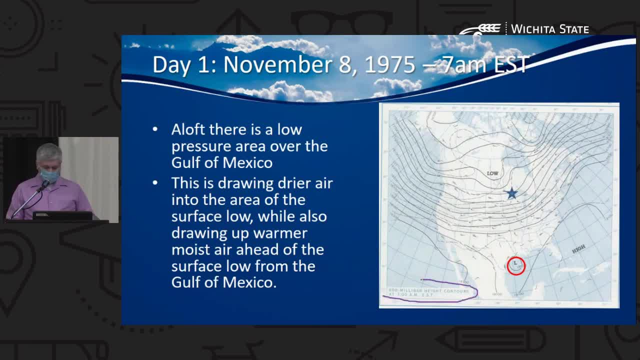 This is at what we call the 500 millibar height, And so when you get above the surface of the Earth, we no longer are talking about sea level pressure. We're talking about- we're not mapping across, pulling everything down to a sea level pressure. 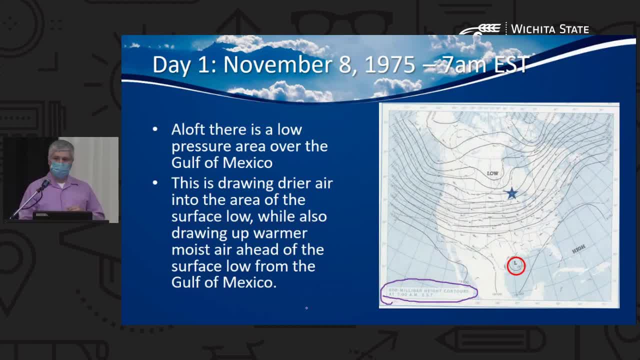 We're mapping the height of what the 500 millibar height is, the location feet above surface That we hit 500 millibars. And so one of the things that's notable when we look at upper air maps versus the surface is you notice there really aren't any closed highs or closed lows. 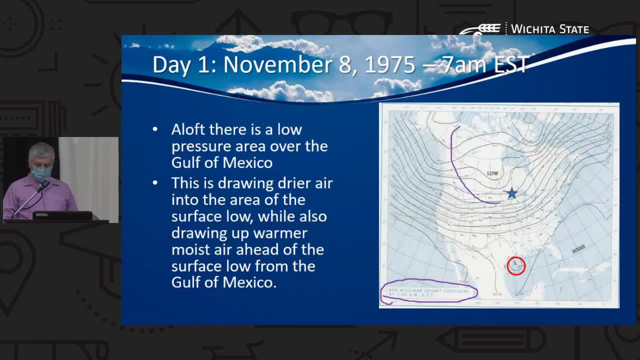 I mean you've got this. they're very large areas, generally speaking, most of the time of your low pressure, your high pressure, and they're not what you typically call closed off, which means you have a real concentrated sort of center of high pressure. You just have these what are called. you know really more of waves across the planet at those upper atmospheric locations, And the reason for that, in large measure, is you don't have the topography Near the bottom kilometer of the atmosphere is where the most mixing is occurring, because we have everything from mountains to buildings to everything going on. In this lower atmosphere, The lower, lowest part of the atmosphere. But when you get above all of that the westerlies, our general flow across, our general flow across the planet basically takes most of the air from west and moves it to east in this part of the world. 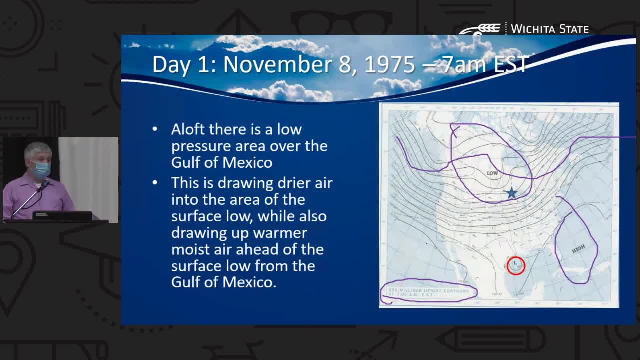 And that's what you see here. Now what we do as meteorologists is we are trying to identify some of those places like right here We're aloft. We do definitely have a closed off low pressure system, because we know that that is going to enhance the surface low, actually more like that, the surface low that we have, because aloft, this low is going to start pulling in moisture out ahead of the surface low. 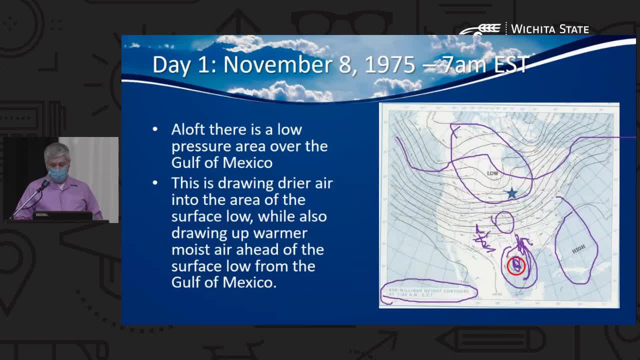 And so we know the general flow is going to pull this low. And so we know the general flow is going to pull this low into an area that's going to enhance the low pressure at the surface more. Does that make sense? Any questions on that? 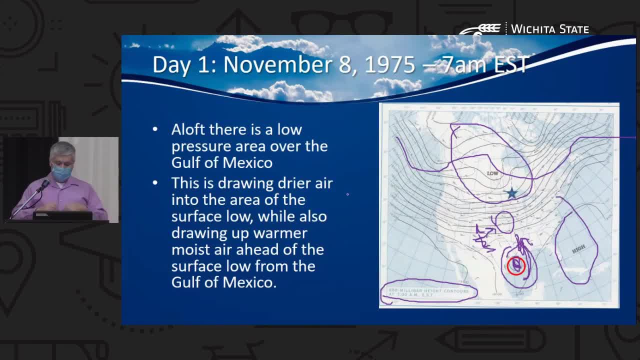 I hope I'm not talking too above. This is kind of a: what happens at the surface is enhanced by what happens above, And so that's what's going on. That's how meteorologists knew that there was going to be some enhancing of this low. 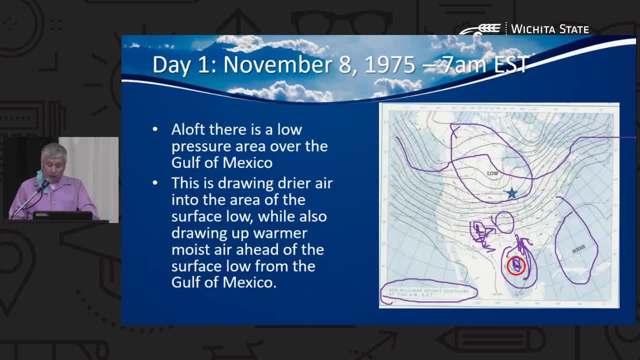 uh, in colorado, low frankly. uh, that was going to start moving through the general flow up toward the great lakes region. it was going to encounter this moisture drawing in ahead of it and the drawing out of the um of some moisture behind it was going to propagate that. 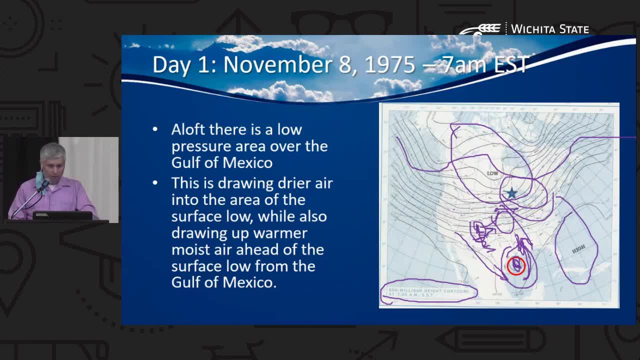 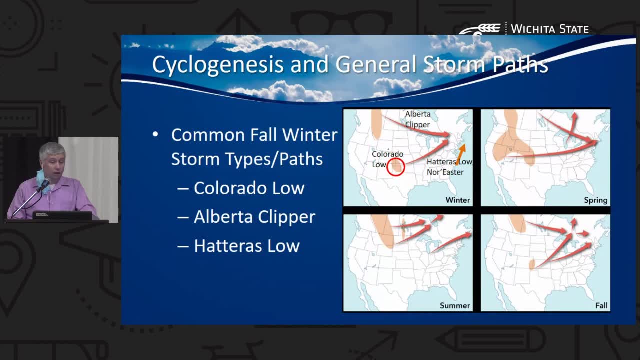 strengthening over the next 24 hours. so i had mentioned that that was a colorado low that was forming, uh and that's uh. what this is just showing is our general locations over the course of the year, which do change a little bit season to season, um of where our mid-latitude cyclones form. uh, our intent, you've probably 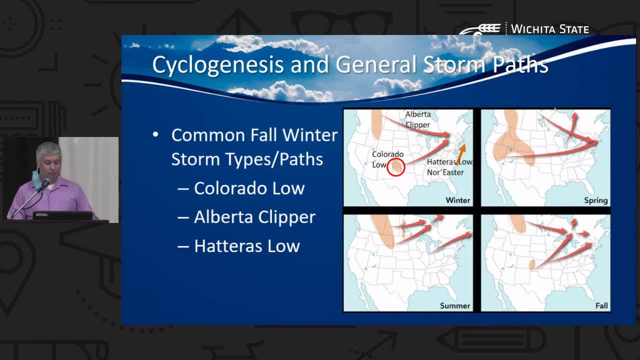 heard of alberta clippers. those are literally formed in alberta and they kind of. they don't generally have too much impact on us here in kansas, uh, but they have big impacts on the- uh upper midwest region. uh, back where i grew up and everything. 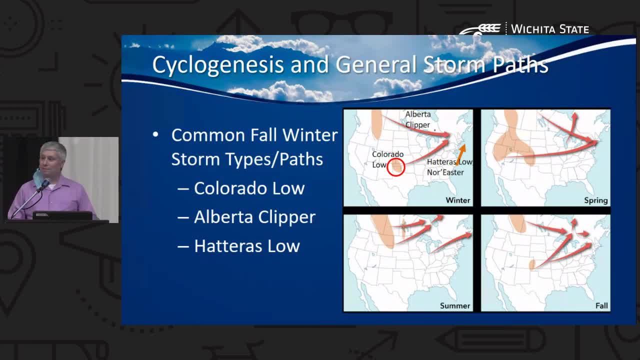 like that. um, you'd hear about alberta clippers all the time, uh, and those were the times where, as a kid, we would be rooting for snow days, because they tend to drop a lot of snow that is light, fluffy, uh, and deep. uh, there's also the colorado low. that's going to be a little bit more of a 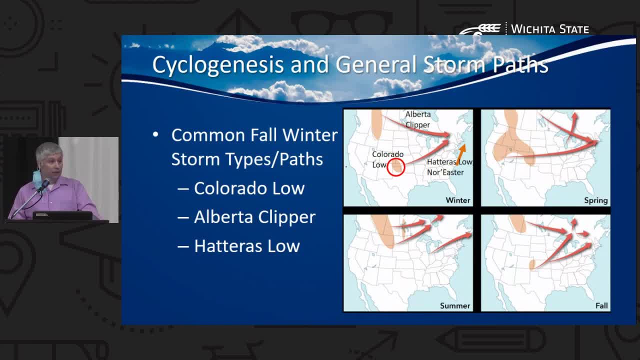 low. that's what impacts us across the central plains most often. that's true both during the winter and the summer months. um, and that's that's what it was uh occurring for this uh storm that sunk the edmund fitzgerald. um, there's another low that we focus on, which is- uh- i drew this one in- 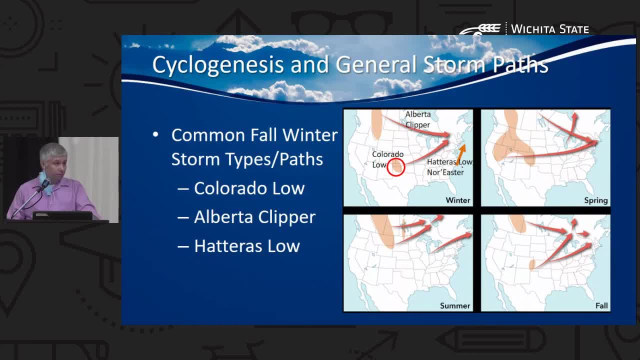 since it wasn't on this map. uh called a hatteras low and the hatteras low is is the uh low formation, doesn't always, but uh frequently will become a nor'easter, if you hear that term thrown around. uh, which uh nor'easter can be a real. another one of those really tightly wrapped low pressure. 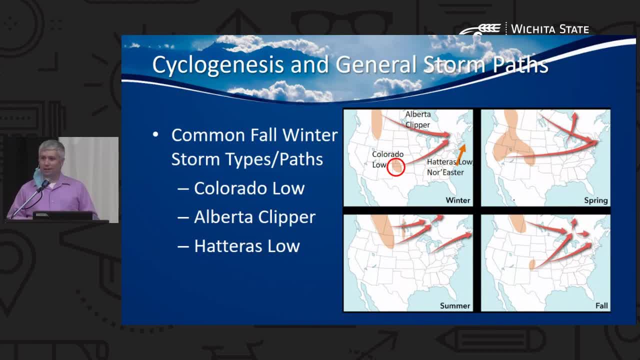 systems that that sometimes get referred to as, like a winter hurricane, um, because of how deep that that system can get and how, uh high the winds within that system can get. and, as you see, uh, you know, looking across some of the other um seasons, we don't have quite the same level of intensity across this part of the country. you get some, some 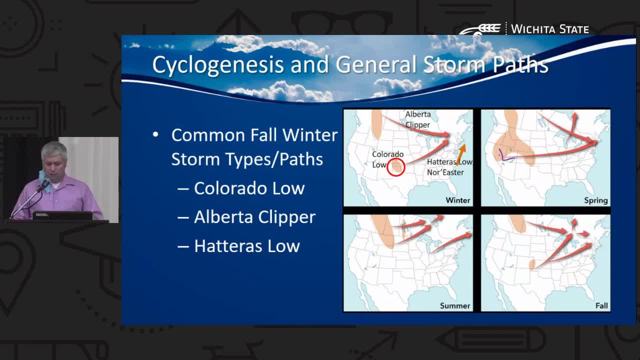 of this springtime- and i'm not going to cover this too much- some of this springtime uh storm paths will create some of the severe weather we wind up having across the uh uh central plains, tornado, tornado, tornado, alley region, um, and so we watched that during those months. but today we're going to 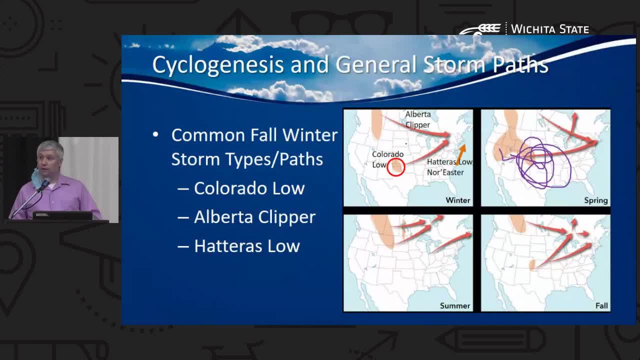 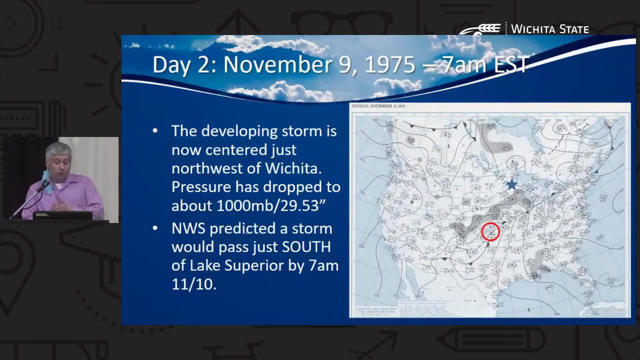 talk about some of the more major financial changes in the winter, and those are our main regions for where we're going to see cyclogenesis occur. oh, went too far. so we're now on november 9th 1975 and our developing storm has kicked out a little bit. that low pressure aloft has pushed it. 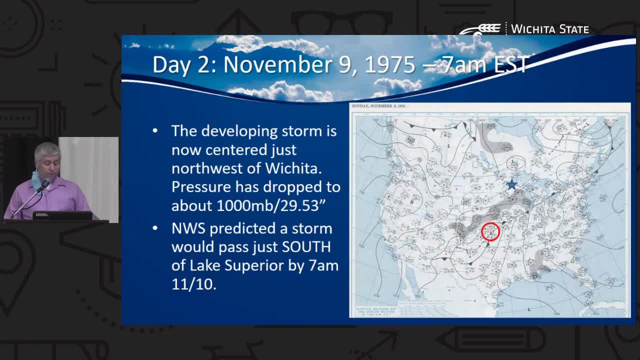 a little bit further to the north and to the east. Remember we had talked about our average sea level pressure being about 10, 13.25 millibars and 29.92 inches of mercury, So we're definitely now below that. 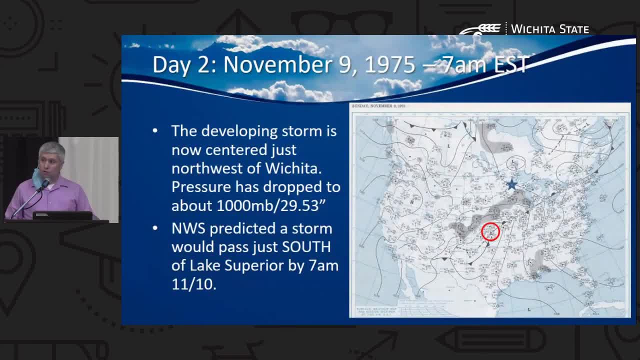 We're having a fairly rapidly intensifying storm at this point that is starting to wrap itself up. National Weather Service at this point has also predicted that a storm would pass just south of Lake Superior by 7 am on 11-10, on November 10th. 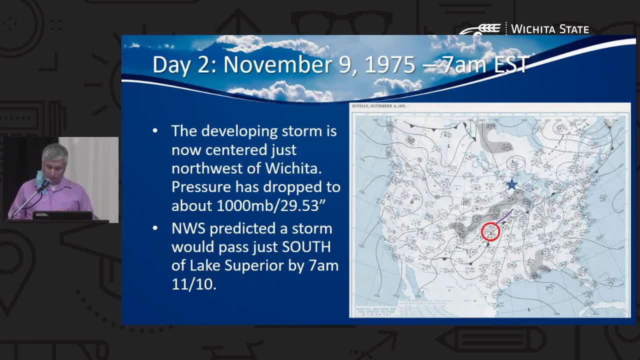 So the forecast, the going forecast, was pulling the storm about like that And we're going to see what the path actually was. So in November, the shipping lanes across Lake Superior, the boat captains, many of whom were very experienced, including the captain of the Edmund Fitzgerald, had 30, 40 years of experience. 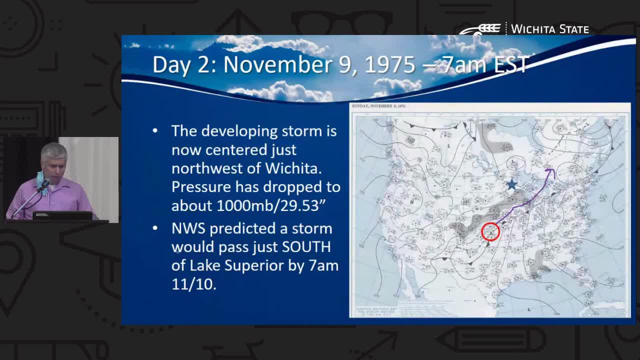 Actually, he was getting very near retirement, And so they all were used to these kind of things, These kind of situations, these kind of setups. If they were, you know, getting ready to ship across the Lake Superior, they'd be concerned. 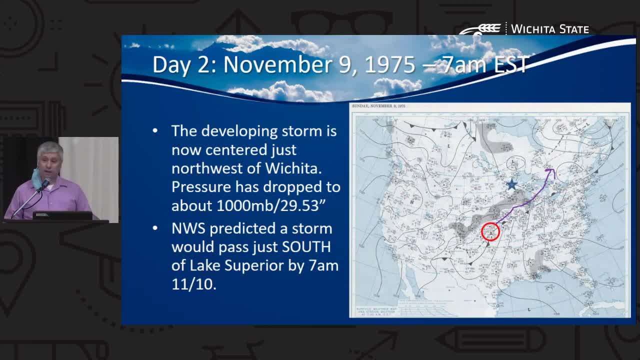 But there's two routes across Lake Superior that they could take. One that is the northern route as they would call it- And I believe that might be on another slide as I go in here- And then their regular route. Their northern route, took them into Canada and kind of closer to the land mass. 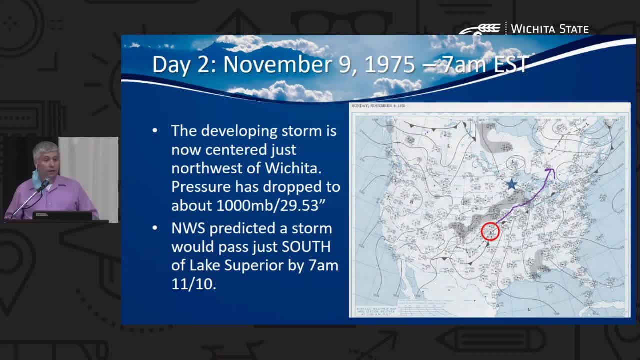 Which probably Protected them a little bit more from the extreme winds that could happen in these storms. And then their southern route, which they would take during the summer months and when there wasn't nearly as the concern about weather, kind of cut straight through Lake Superior and sort of an arc path across the lake. 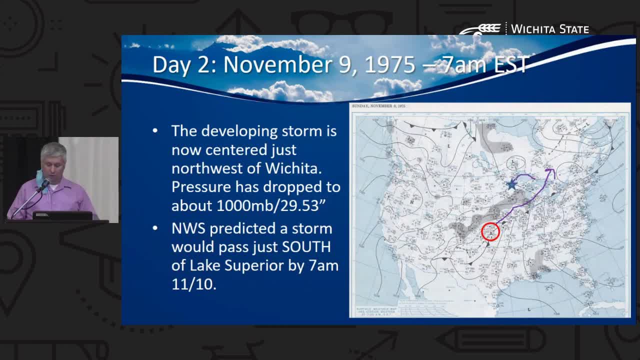 Kind of more like that. Well, I kind of drew that more along the northern route versus southern route Kind of went like that. So McSorley and the other captains on Lake Superior that are departing about this time, they're watching the weather pretty closely. 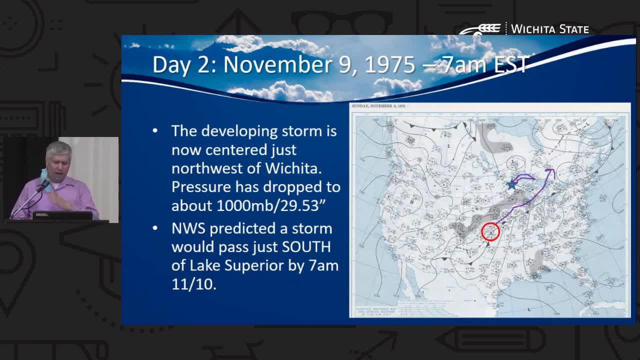 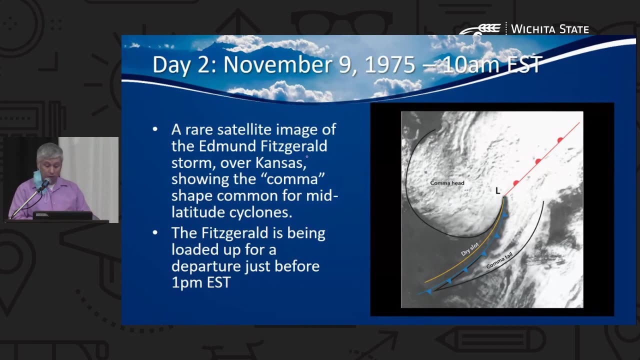 But weather service is saying it's probably going to pass a little bit south. You'll get some high winds, But nothing horribly out of the ordinary for November. So this is a satellite image taken at 10 am. So this is a satellite image taken at 10 am. 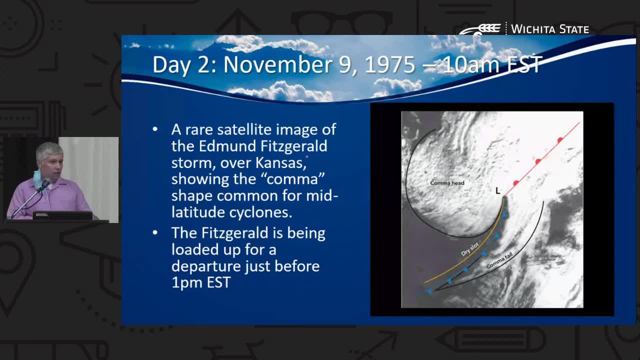 thing that's uh important to note is that, you know, we're back in 1975. there. yes, we do have satellites up there, uh, but our, you know, we're barely into the space age at this point, um, and so our satellite images aren't pretty much constantly taking pictures. um, this is one of the few um clear. 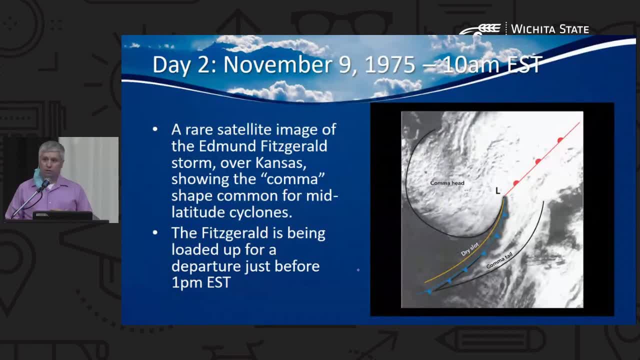 photographs that that even exist, of the storm that sunk the edmund fitzgerald um, and this is at 10 o'clock on uh, 10 o'clock eastern standard on november 9th, and drawn on here are the frontal boundaries as well. uh, you're kind of getting a picture as well of the? uh, kind of the general look. 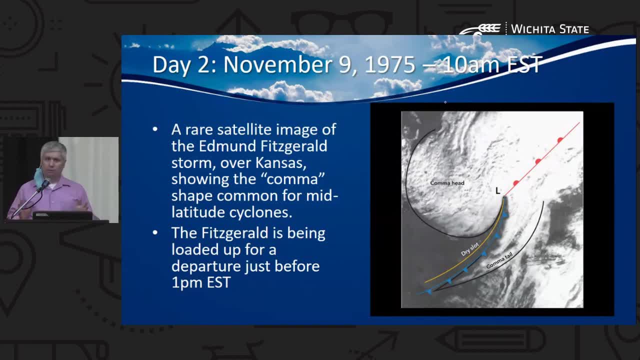 of these mid-latitude cyclones. you've all probably seen this on weather maps before- um, the you- you kind of have this comma. look, if you look at the satellite um, and this is a visual satellite image. there are multiple different types of satellite images you can look at. 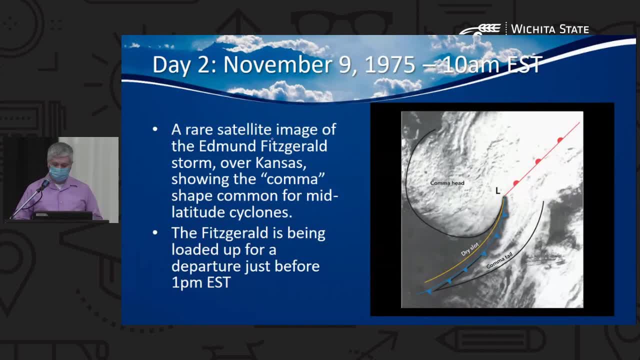 but this is literally a camera picture of the surface. uh, right now. now. the problem with visual uh satellite images is they don't look good when there is no sun, which is why that you'll also hear of infrared satellite. an infrared satellite can take pictures 24 hours a day, whereas visual or visible uh satellite imagery is not as uh. 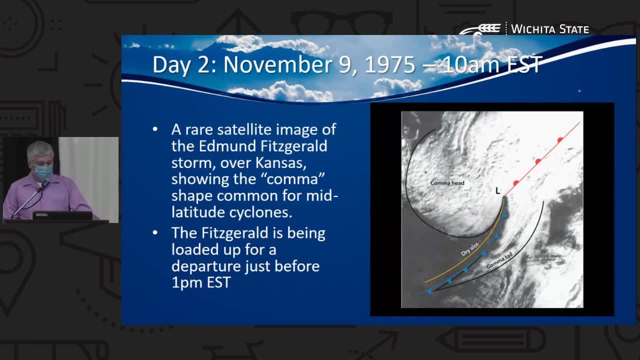 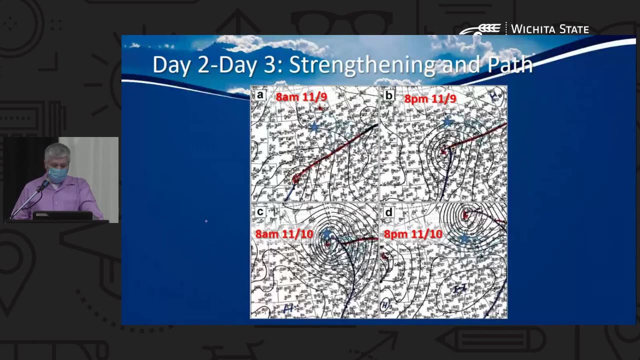 you can only do that over about 12 hours of the day, uh you know, one o'clock in the afternoon the uh fitz is being uh finished off on getting loaded up and getting ready for its departure across lake superior. so now we're looking at the strengthening uh and path of this storm. 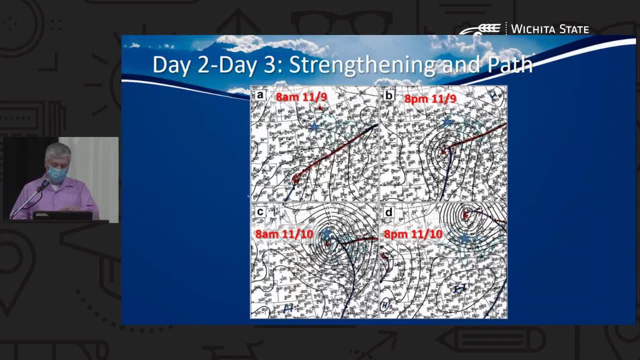 how it tracked versus how it was forecast. well, how it was forecast is not on here, but how it was tracked. so we looked a little bit at um the eighth. now we're looking at the ninth and the tenth, ultimately, uh, we see at 8 am on the 9th. 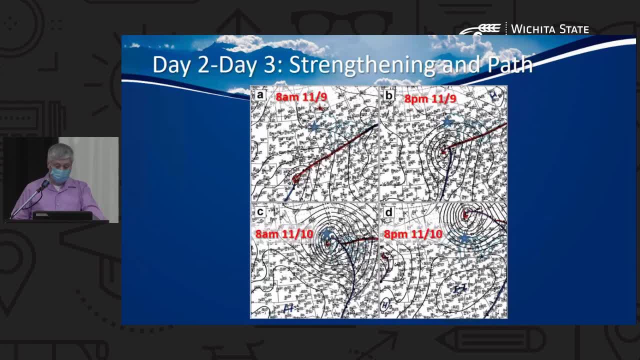 we have that low basically on top of wichita kansas, uh, at this time, as it's starting to build 12 hours later, at 8 pm, and these are eastern standard times, uh, as opposed to the central standard, uh, this low is definitely deepened more. it's uh, more tightly closed off and you're seeing. 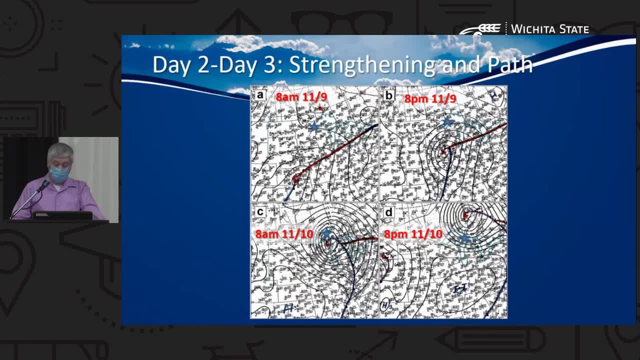 the, you know the, your black lines, just like we talked about last week, those are your lines of equal pressure. now, if you're ever finding yourself looking at a weather map and determining, uh, the weather map, and determining, uh, the weather map, and determining, uh, okay, where are my high, highest winds? always look for where are these isobars the tightest. 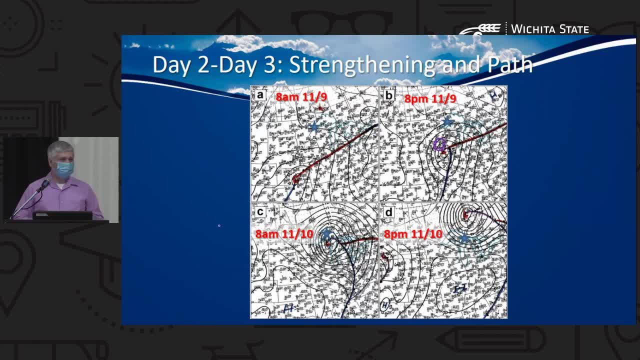 your winds are always going to kind of correlate with those really tight isobars where the pressure drops really rapidly. you can sort of think of it like a funnel, like if you go to like a science museum or or the zoo or any place. that's kind of collecting donations that maybe kids go to with their parents. 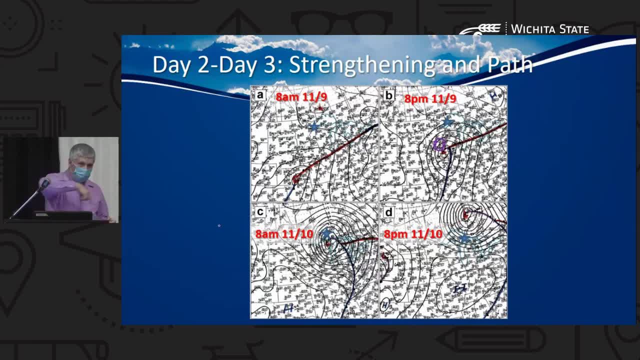 You have these big funnels that you can kind of drop a coin and the coin spins And you notice it spins slower at the top and then gets faster and faster and faster and faster as it goes down the middle. A low-pressure system is very much the same way. So the closer you get to the low, the tighter things get and the faster the winds get. So now we're at 8 am, on the day that the Edmund Fitzgerald sunk Again. the star location is kind of where the Fitzgerald is at the time. 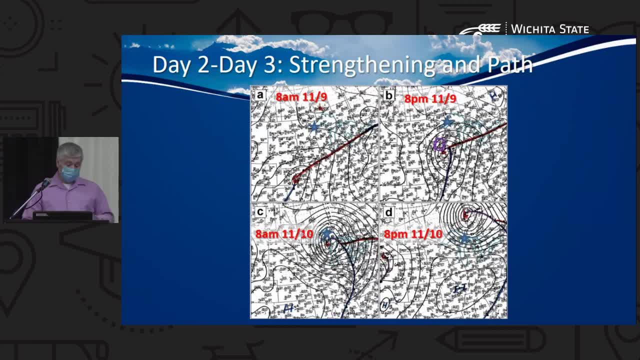 By 8 am on November 10th the Fitz is about halfway across its journey across Lake Superior. It's taking the northern route, which takes it kind of close to the, the landmass in Canada. So it's on sort of the Canadian side of the border, following as closely as possible along the. 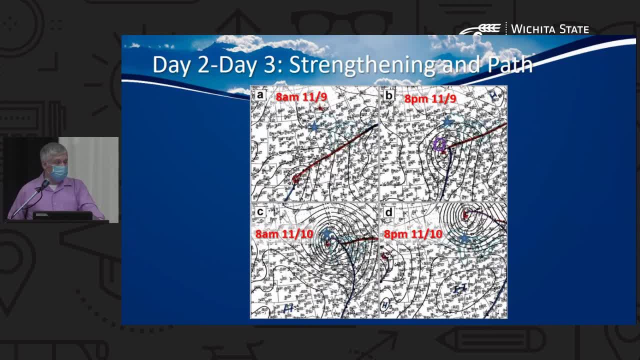 as close as safely possible, I should say along the northern side of Lake Superior, Again trying to avoid the highest winds. And you know, you see, right here I mean they are getting buffeted by high north easterly winds. 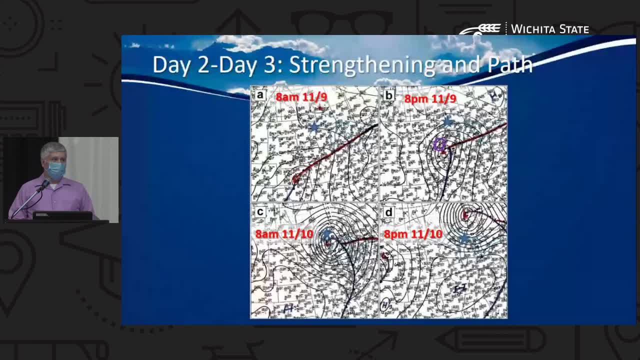 We're going to get into why the wind from the northeast- at high winds- is not as bad as what we're going to wind up running into at 8 pm on November 10th, Where, by this point, it's believed that the Edmund Fitzgerald has been sunk. 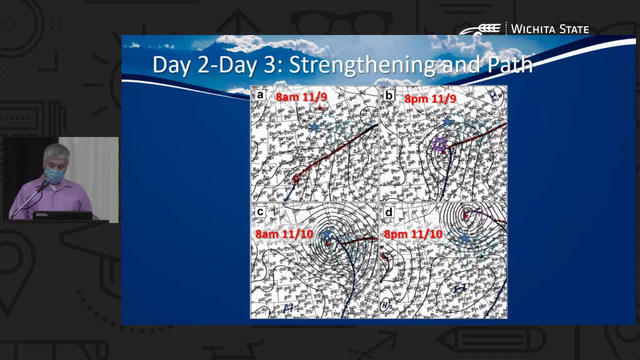 And, And And. the low-pressure system definitely did not go south of Lake Superior, It went right through Lake Superior. So the forecast prior was a little bit off And while it wasn't off drastically, a little bit of being off can make a very big difference if you are on a shipping freighter going across Lake Superior during the month of November. 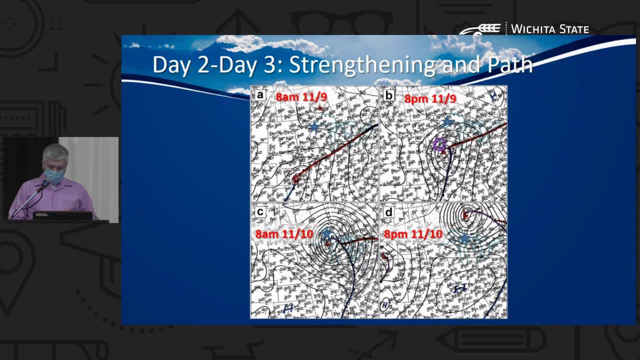 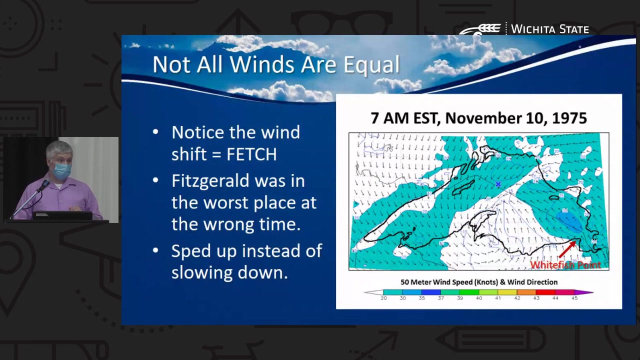 At this point we've got winds coming in pretty intense From the north to northwest across Lake Superior And we're going to get into in a moment why that's so critical. Not all winds are equal, Especially when you're talking about maritime forecasting. 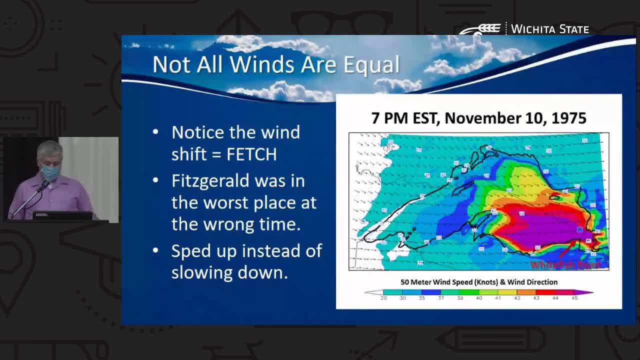 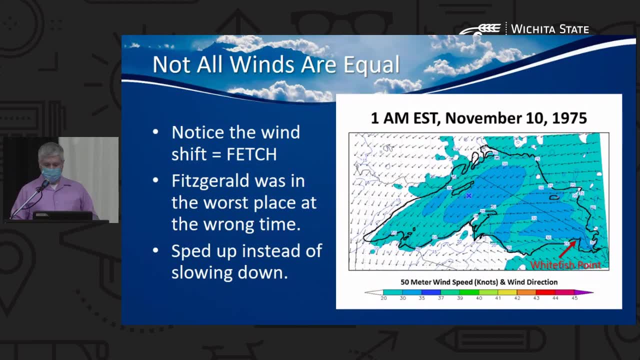 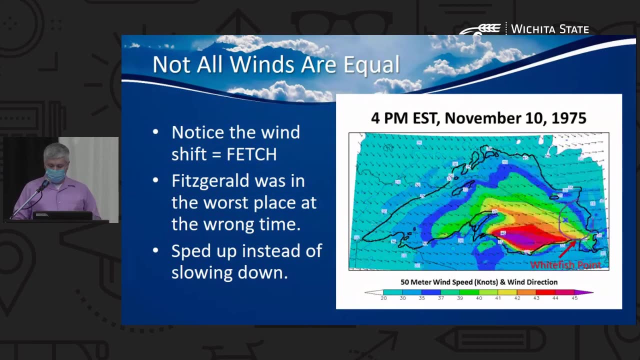 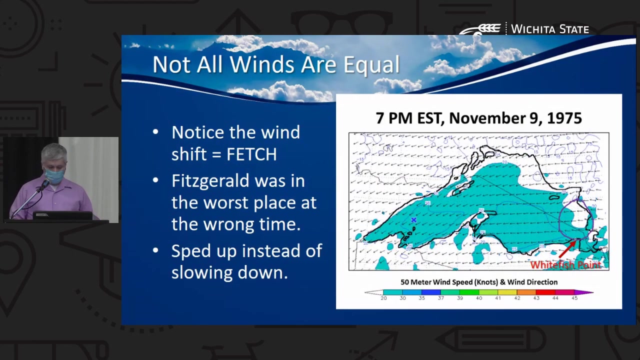 This is sort of a time, A time Going through over time what the winds wind up being at Certain times during this event. It is well known to shippers that the most dangerous part of this journey is right here near Whitefish Point. 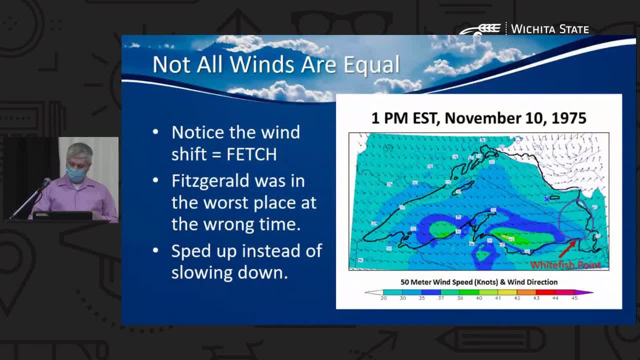 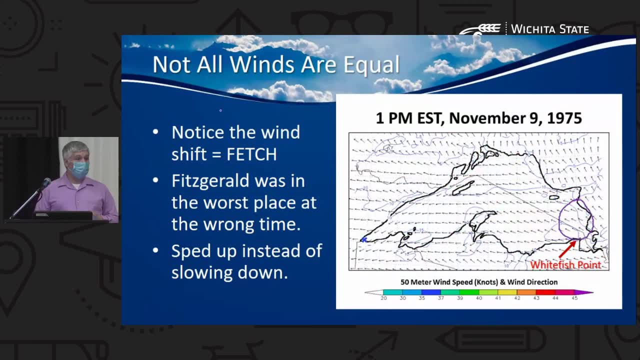 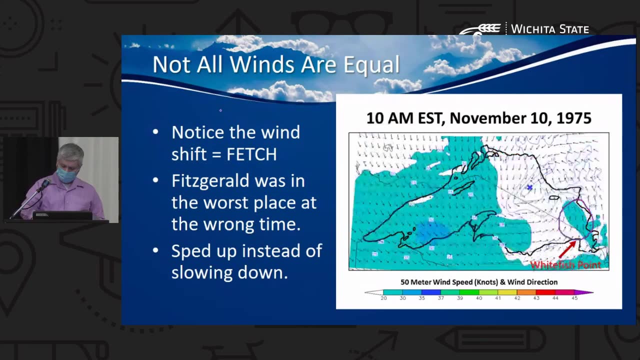 We're seeing this wind shifting around as the low pressure moves And the X that you're seeing on here over time is the location at that point, That time of the Edmund Fitzgerald. So you see the Edmund Fitzgerald kind of going north And following that northern route. 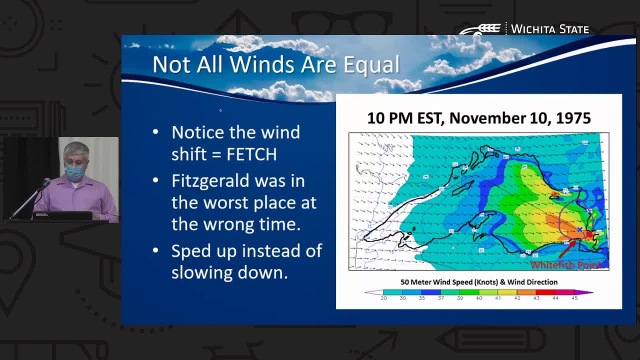 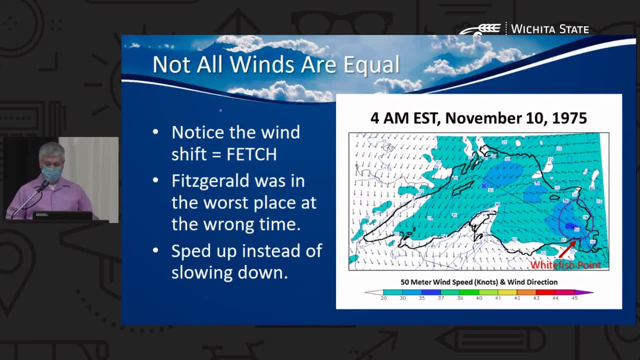 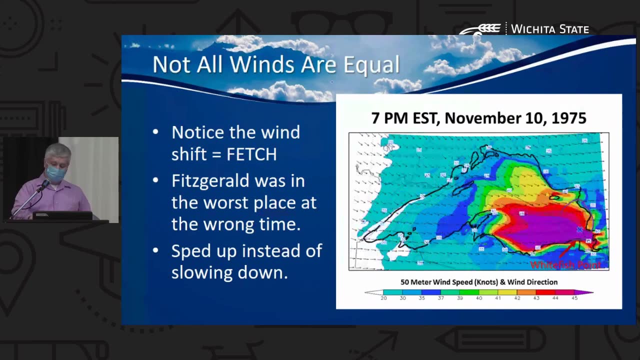 Trying to go through the waters that are still deep enough for it to safely travel, But are shallow enough that the waves aren't being kicked up as high, But literally the time that the low was producing the highest winds and wind speeds coming across the lake. 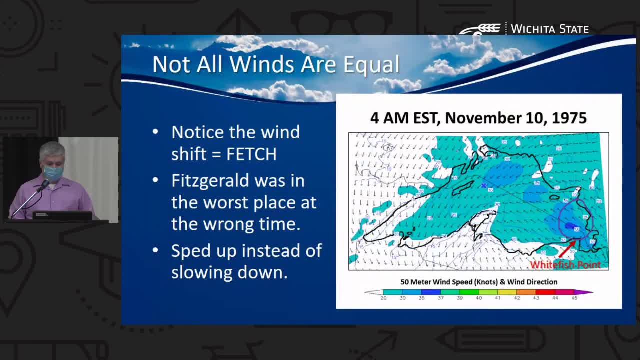 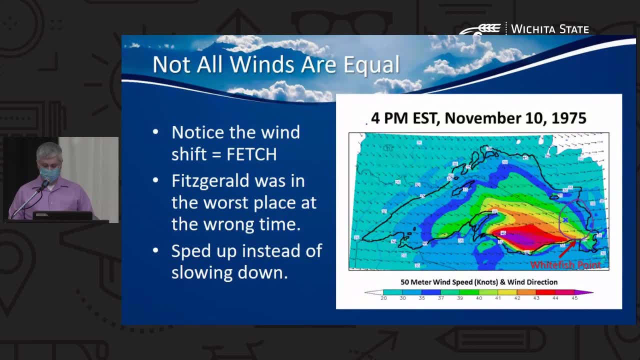 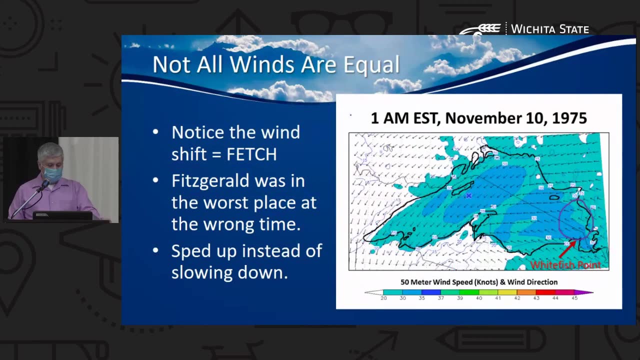 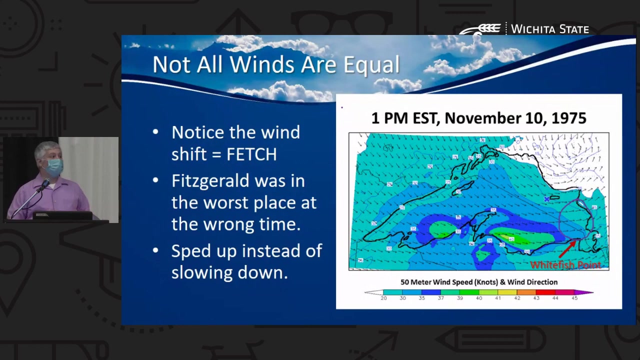 From the northwest Was the worst Right, where the Fitzgerald is going through the most hazardous part of Lake Superior. So the Fitzgerald made the wrong decision at the wrong time, In that they were trying to get ahead of the storm as much as possible. 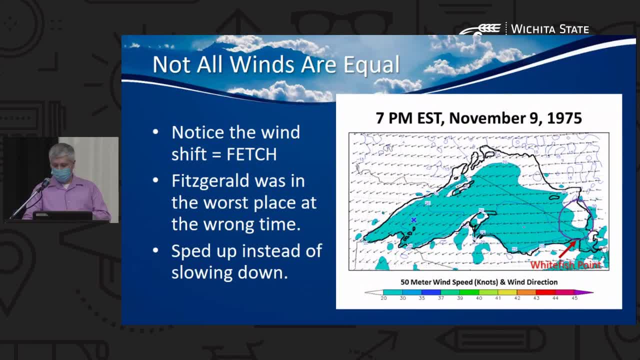 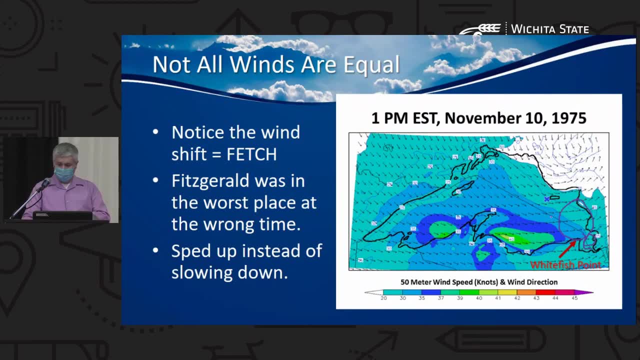 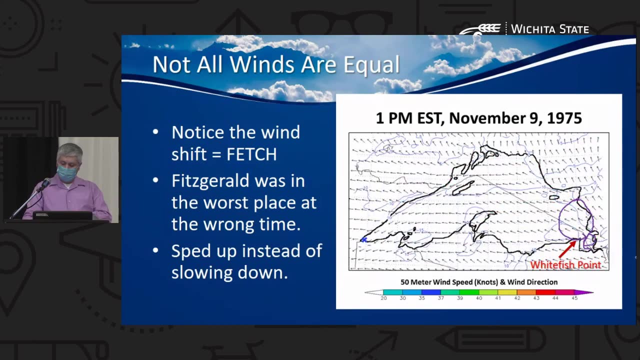 To get past This Whitefish Point. Once they were past Whitefish Point They would be protected from the high waves, Because you notice it gets kind of narrow in here And then you have the high winds But the waves across Lake Superior are broken up. 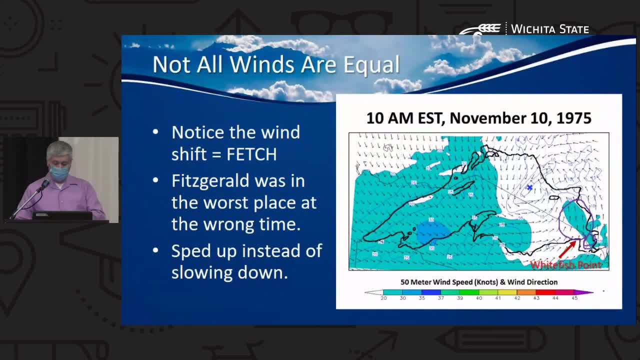 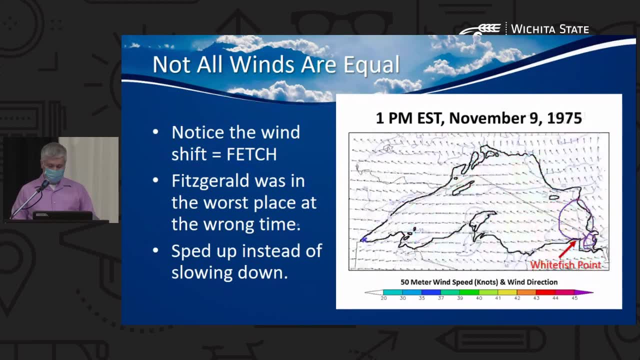 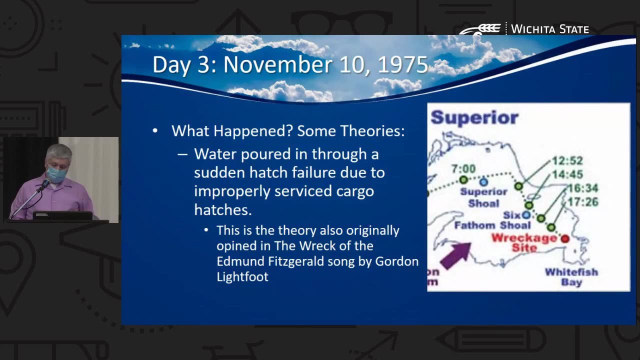 Because, well, there's not as much space for waves to develop there. So basically got the worst possible Hit when At the most vulnerable time. This is sort of showing a little bit again of the progression of the Edmund Fitzgerald over November 10th. 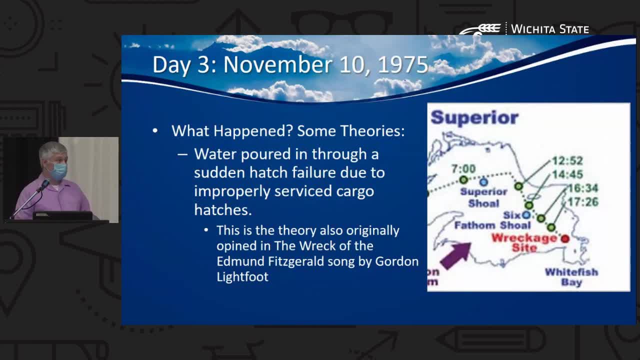 And there are a lot of theories as to what led to the sinking of the Edmund Fitzgerald. No one is 100% sure It was partially a mechanic, In terms of the hatch sealed down enough, Since this was a shipping vessel. These shipping vessels are loaded in from above. 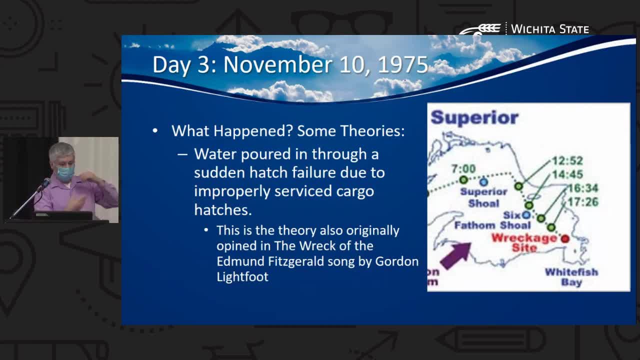 And so you have these large hatches that open up And then you just put in the iron ore or whatever into these large hatch areas, And one of them was that the hatches weren't being serviced properly, And that Was also the theory that made it into the song by Gordon Lightfoot. 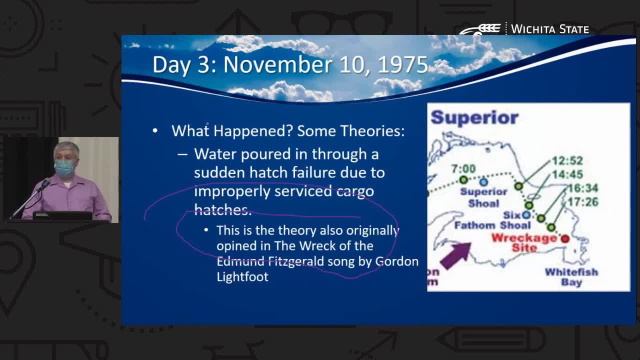 Now interesting side point is that, Well, that still is the way he sings it in the recordings. He's actually changed the wording of the verse that talks about the sinking, And it's changed, Taken out the insinuation that That it was a human error. 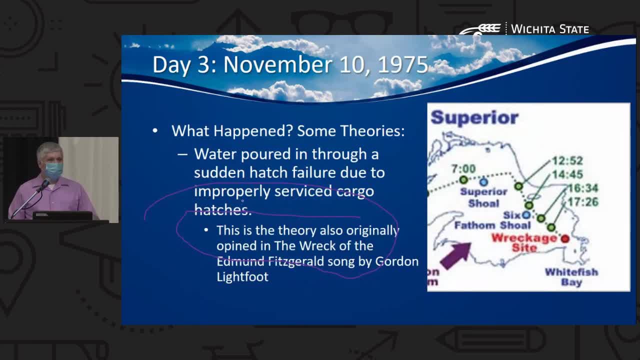 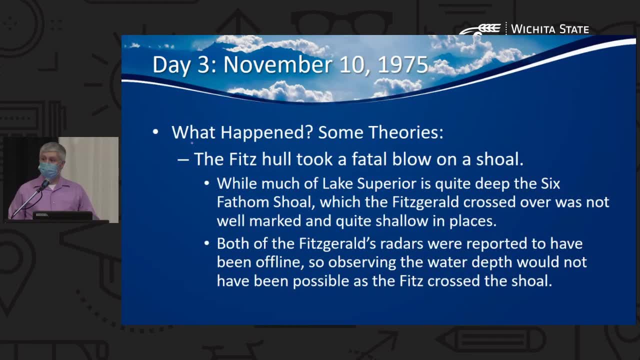 And that it was more of a just freak accident. Another theory is that because the waves were so big. You know, as you build up all of this water into a wave Well, where the wave is really high, there's got to be a place where it's really low. 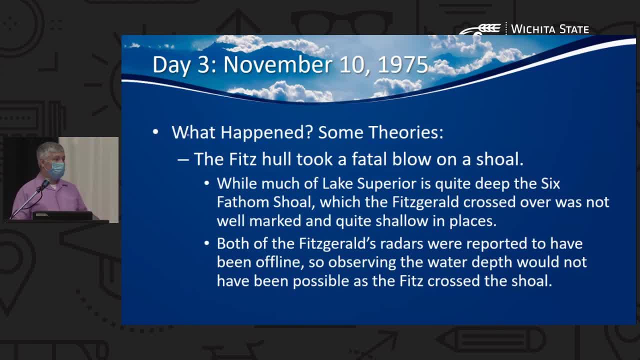 And the Fitzgerald was going through an area of Lake Superior That, relative Relative to Lake Superior as a whole, was pretty shallow, And so there's a belief that it possibly hit ground and ran aground between large waves. And, you know, at that time the Fitzgerald's radars had been knocked offline. 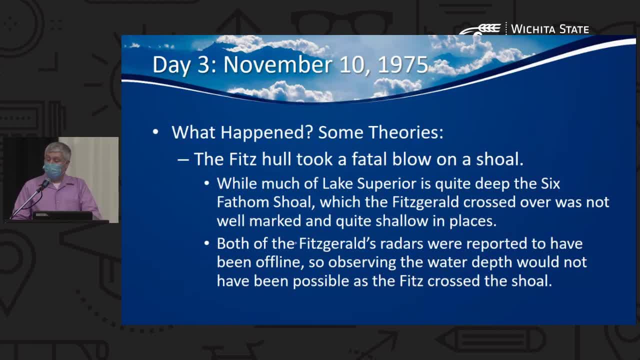 So no radars. You're kind of flying blind to a certain extent. They were up until Until the very end in radar communic Or in radio communication with the Arthur Anderson, Which was another shipping freighter that was nearby And the belief is that it may have gone down. 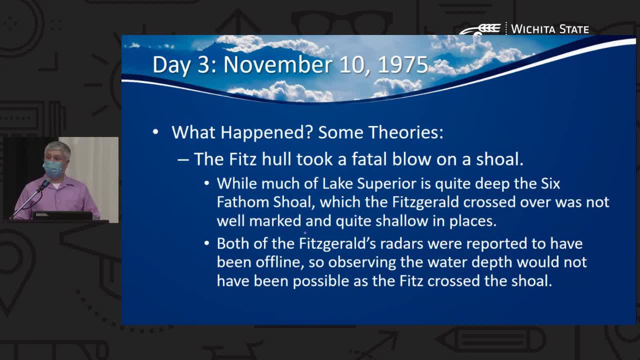 Hit aground and was overtaken by a wave and went down real fast. The last thing that the captain said to the captain of the Anderson was: We're holding our own. That's the fatal last thing said. So that didn't sound real bad. 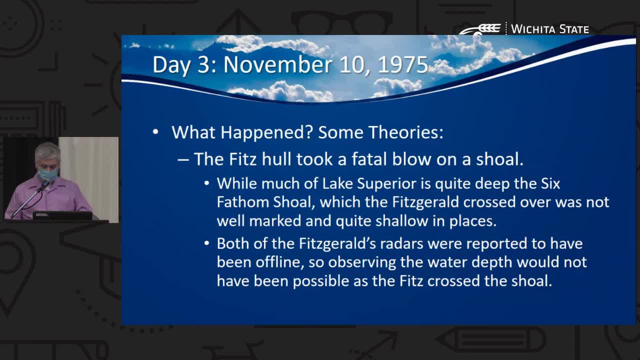 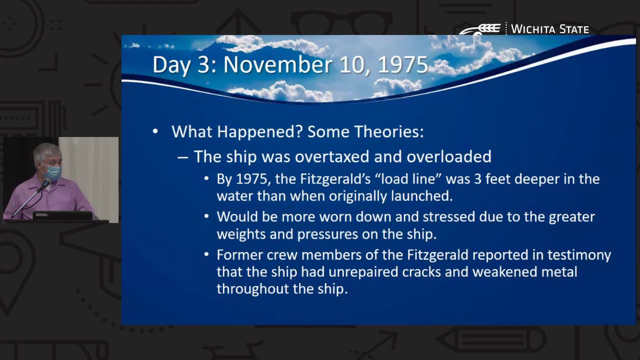 But next thing they know they can't reach the Edmund Fitzgerald at all. Another theory was that the ship was just being overtaxed. I mentioned that it was sort of the pride of the Great Lakes And was continually over its service life, beating its own records for shipping across Lake Superior. 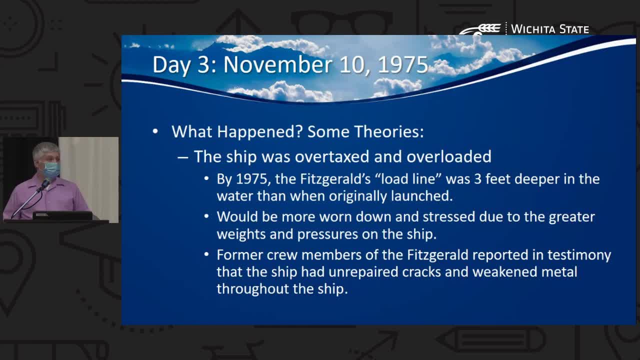 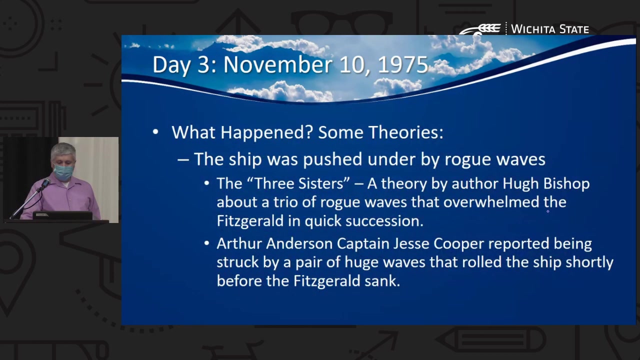 And so the belief is that it was getting loaded so much that it was being pushed further and further into the water, And that would have made it a lot more susceptible to being sunk by high waves hitting it and just overtaking the ship. This is the one that is a lot more. 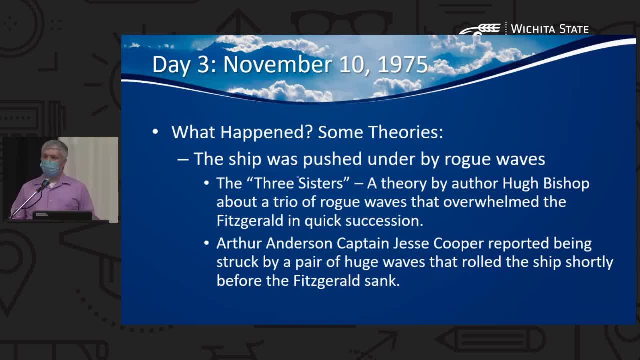 The theory that is Primarily accepted today for what sunk the Fitzgerald was that, Yes, there may have been some mechanical issues going on. There may have been a case of, Yes, maybe it was a little bit overloaded, But really, at the end of the day, the Fitzgerald was in the wrong place at the wrong time. 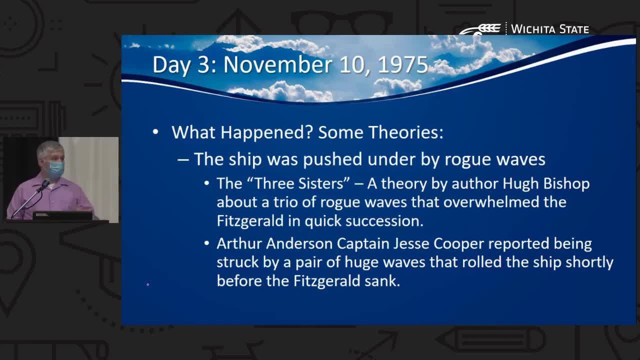 And got hit by two or three really massive waves that were just too much for the ship and brought it right down. There is some evidence that supports this in terms of reports from shipping captains that were in the area of the Fitzgerald, And there's been 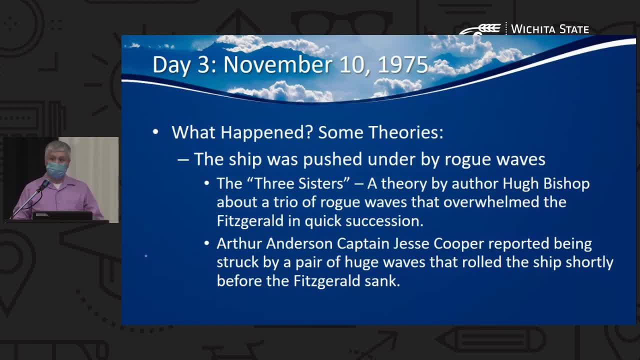 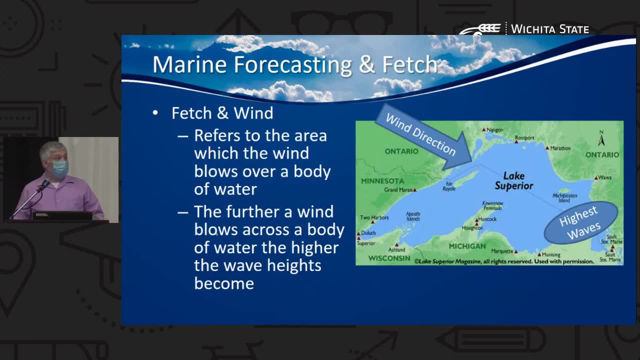 These theories have a fair amount of support meteorologically as well. We talked about the winds and that not all winds are equal, And this is very, very true when we're talking about maritime forces, And this is very, very true when we're talking about maritime forces. 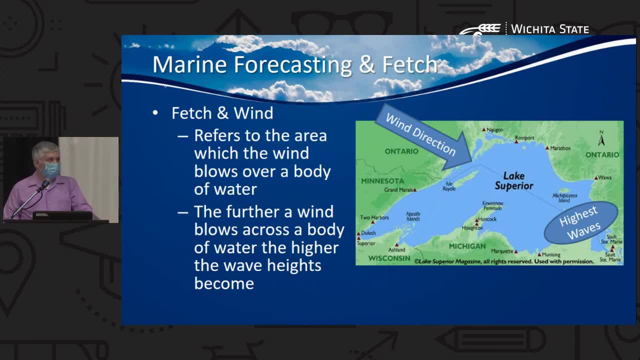 And in this case we always have to look at Fetch, And Fetch has nothing to do with your dog. It's a reference to the area by which a wind blows across water, So we don't worry too much about Fetch here in Wichita, Kansas, because we don't have large bodies of water. 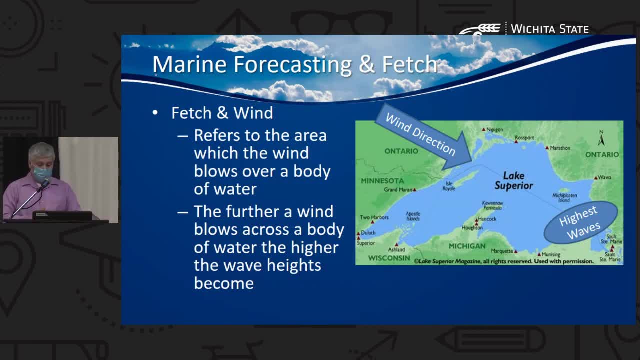 The Great Lakes, however, have very large bodies of water, And so what direction- The direction the wind blows really matters, especially over time. So remember, our low-pressure system was up here when the Edmund Fitzgerald sunk, Actually probably a little bit further north. 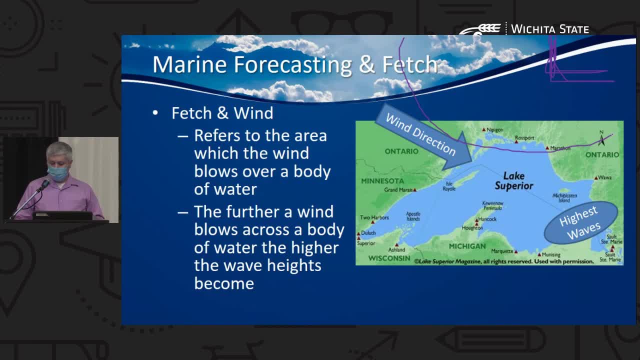 Well, we know that counterclockwise flow around a low-pressure area And so we had tight isobars, windmills, Wind coming from the northwest across Lake Superior. That is the largest stretch to very easily have unabated wind across the body of water. 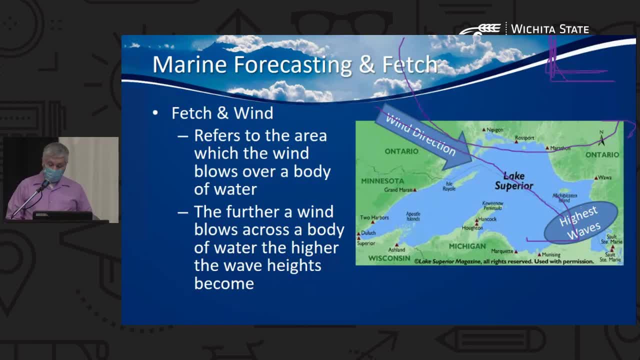 So when we get that set up, we get very high winds or very high waves right here. Now, if I were to turn that wind direction more northerly, which, as that low-pressure system continued to move, would happen- 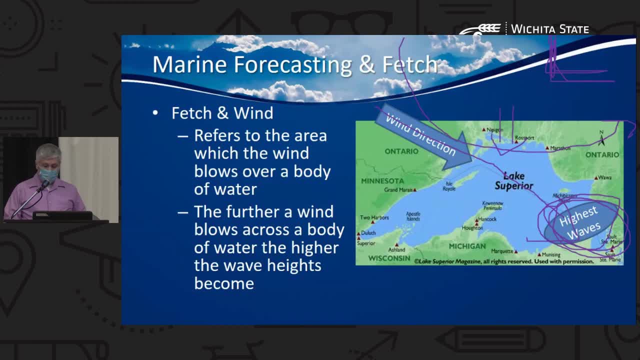 you're going across a shorter amount of the lake, And so your waves don't get nearly as high down here as they do when you've got that northwesterly direction. So, literally, the Fitzgerald was in exactly the wrong place at exactly the wrong time. 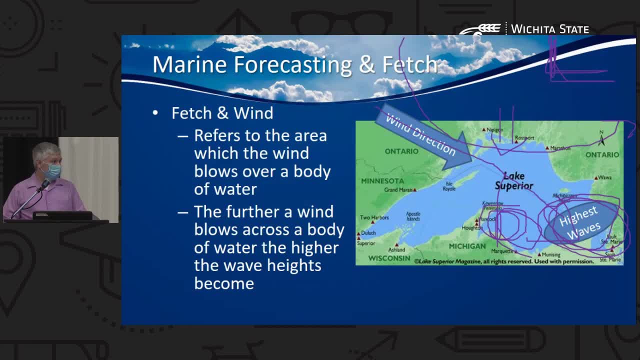 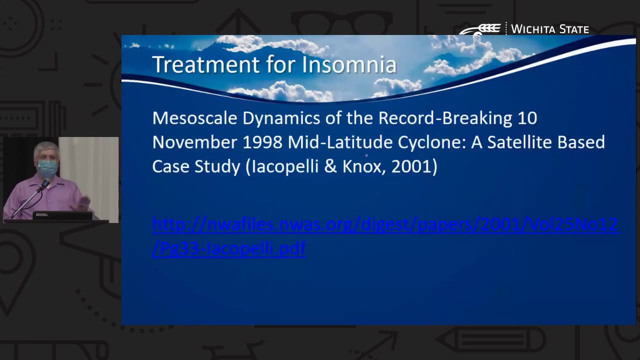 which again supports the meteorological conclusion- that probably got hit by some 30- to 50-foot waves in Rapids. So that's a little bit of a conundrum, But it was just too much for the ship. Any questions? 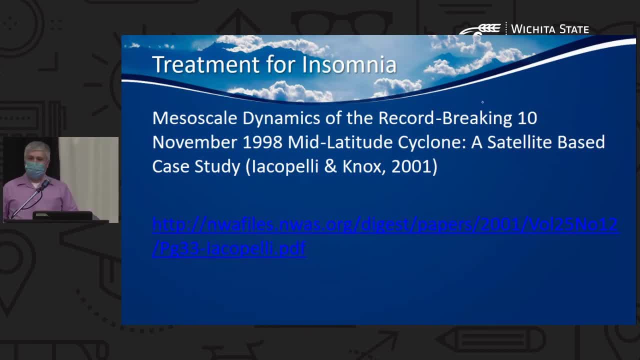 Okay, It turns out I actually have done a little bit, along with a former professor of mine, research on what was really a copycat storm, or at least we believe it was a copycat storm- for the storm that sunk the Edmund Fitzgerald. 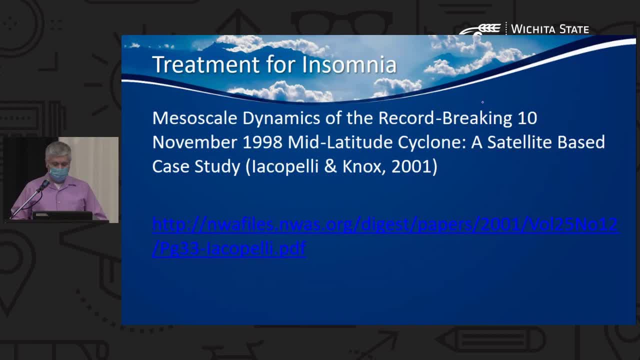 If you are having trouble sleeping, you're going to have to do a little bit of research. If you are having trouble sleeping, it's a great paper to look up And it turns out because I had to search for this this morning. 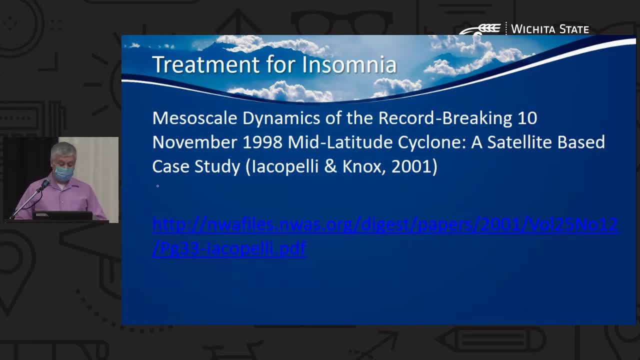 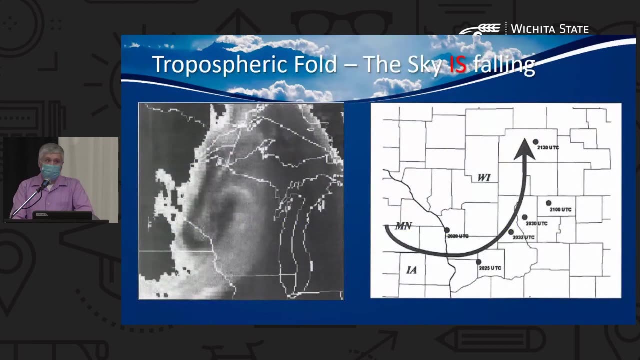 every now and then I kind of check to see if I can find it somewhere on the Internet just sitting around And it is there out there in a PDF format that somebody's got up there And basically here's the conclusion that we had out of that. 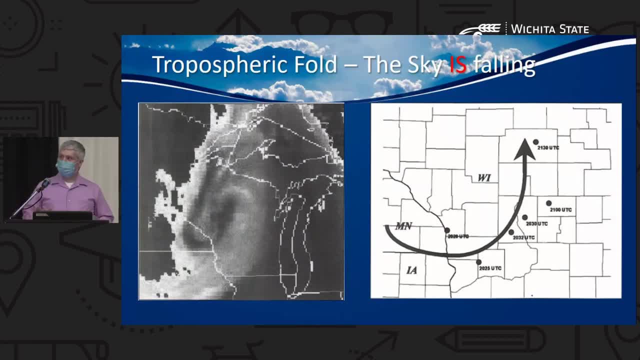 And then, oh good, I went fast through it, But I stayed a lot more on target time-wise than I thought I was going to. What we found when we were going through the data- and this was something that had been worked on a little bit by another researcher for storms off of the coast of the European. 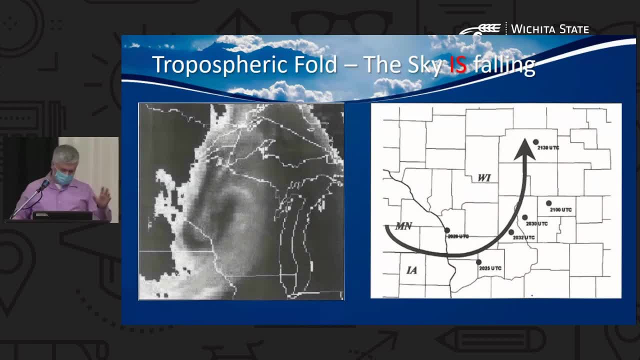 well, yeah, really more the European coast, similar type of mid-latitude cyclone. But it was a pretty good situation And if you have kind of older printouts of the slides, you might not have this because I added it in just recently. 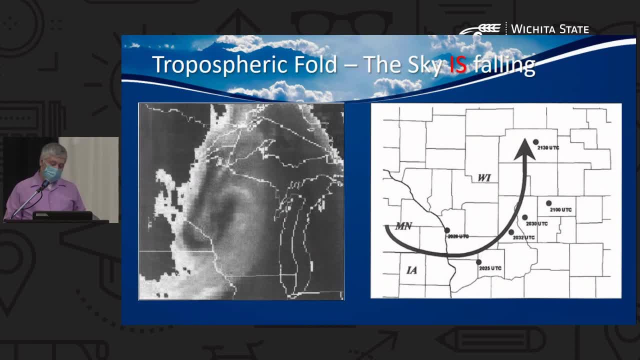 But what we found with this storm, and this is a storm from 1998.. It was like almost the exact same day, I think we were shifted by a day or two. But we noticed on the satellite this hook shape. And that hook shape, it turns out, was associated with very, very mesoscale, so small scale, very high winds at the surface. 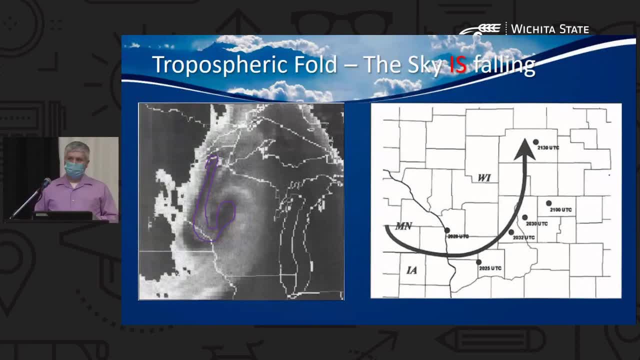 And that is what has been referred to as a tropospheric fold. We have several different layers of the atmosphere And the troposphere is the lowest layer. That's really where all of our, That's where our weather occurs, But there's the stratosphere above the troposphere. 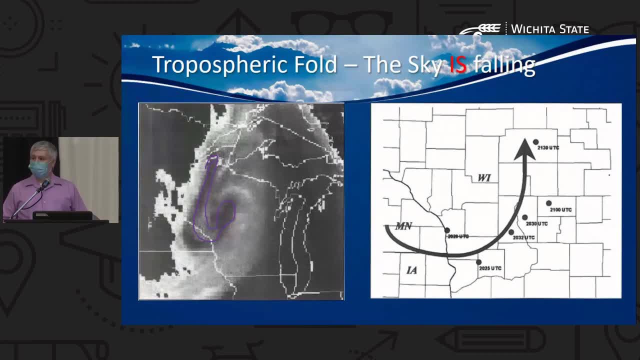 The stratosphere is very quiet. weather-wise, There's really not much of anything up there. It's very dry air, And so where there's dry air, there isn't clouds, And so what we've, you know, noted and found was that the low intensified so much that it started literally dragging the atmosphere down with it. 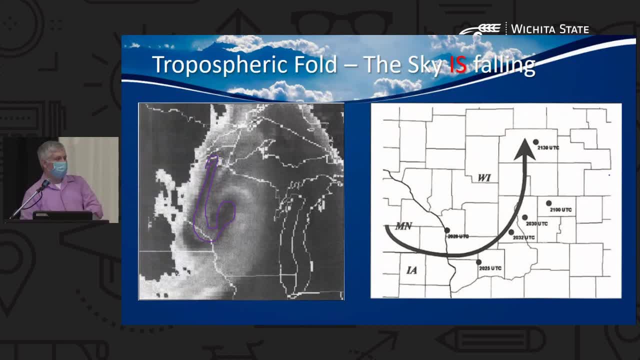 So it was dragging. It was dragging the stratosphere almost folding upon itself, And as it does that, you're getting highly tightened airflow across a very, very small area, And what we have on here are times, And these are in universal time. 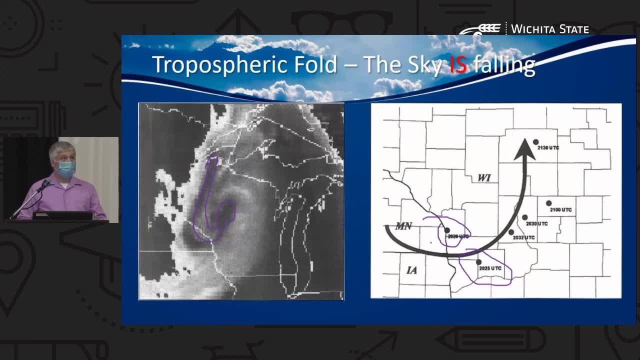 So I can't. I'm trying to do my mental math. Yeah, About 3 o'clock here And onward. So we're seeing over the course of time here And it's a time progression of high. These are high winds at the surface. 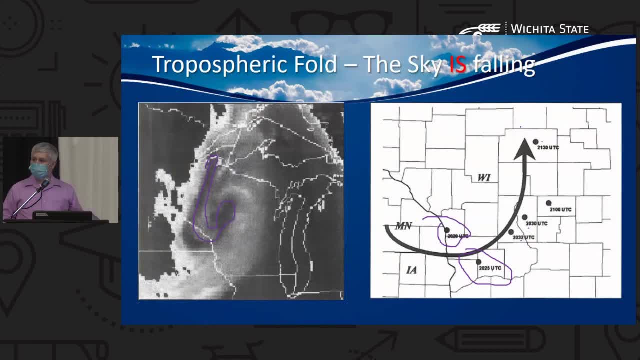 Overall the wind flow. it was windy but not real, you know, real intense, Especially if you're in, you know, Wichita, where we can sometimes get some real high winds that are sustained. But these individual reports, right along The same thing as this little fish hook on the satellite- were very high, intense winds which led to actually some fatalities. 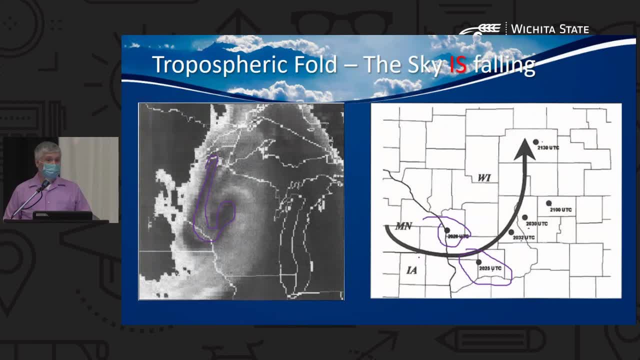 Because individuals didn't expect these really high wind gusts to come out of nowhere, And so what my professor and I were suggesting is that it's really this tropospheric fold That was also occurring At the same time. you're already kicking up really high winds. 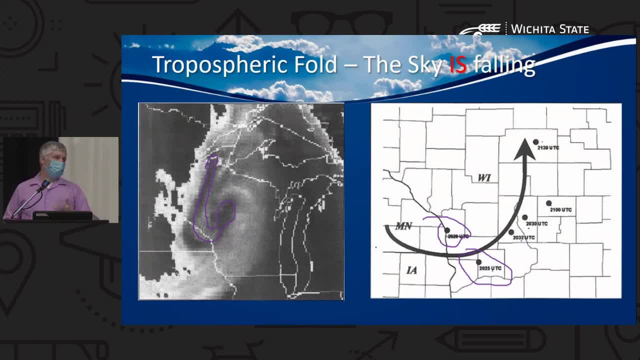 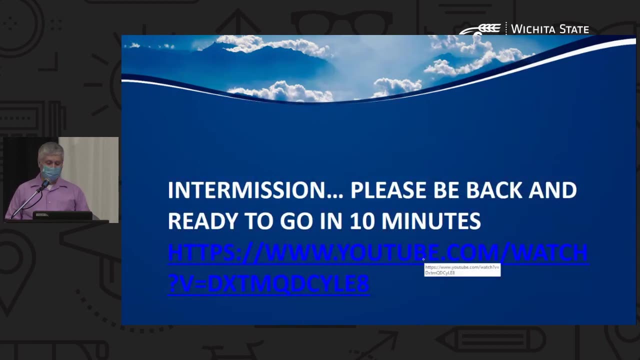 Or really high waves. rather, You were also getting hit with a very intense wind gust at the same time with that system that sunk the Edmund Fitzgerald. So that was some of the research that I did in that area, And I still managed to keep things relatively on time. 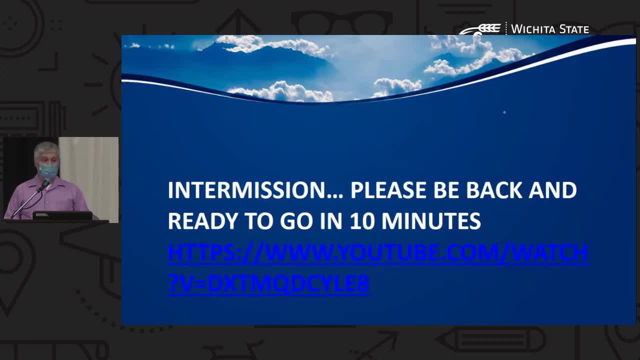 I went through a lot of information there So I'd be happy to answer Questions. That is probably as thick of material as we will cover over the course of the four weeks here, So if you need me to try to clarify, I'm happy to do so. 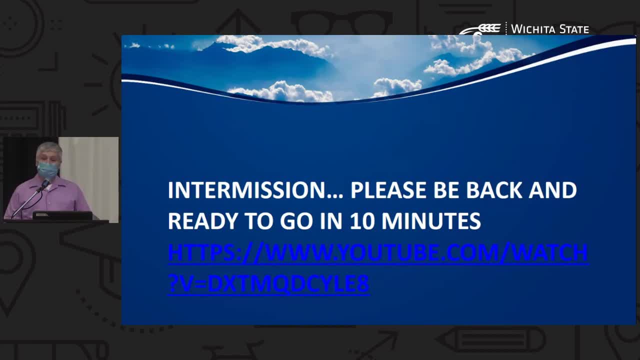 If we've got any questions from those of you watching at home or wherever you are, shoot them to me. Otherwise we will be just about ready for a break. Oh yeah, I'm sorry. I'm sorry. What was the weather in Wichita doing in the 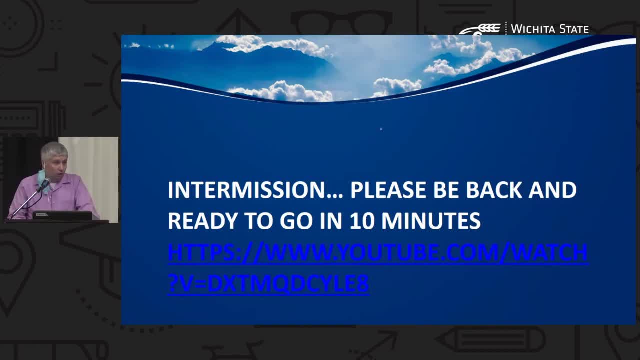 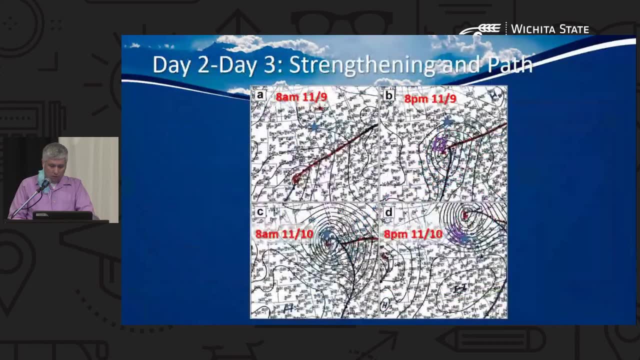 Well, really it was fairly calm. Let's get back to those four. Let's back it up. There we go. We're just starting to see the wind, or the system, intensify as it's coming across, Okay, Safai, as it's coming across the Wichita Kansas kind of Central Plains region here, And you know. 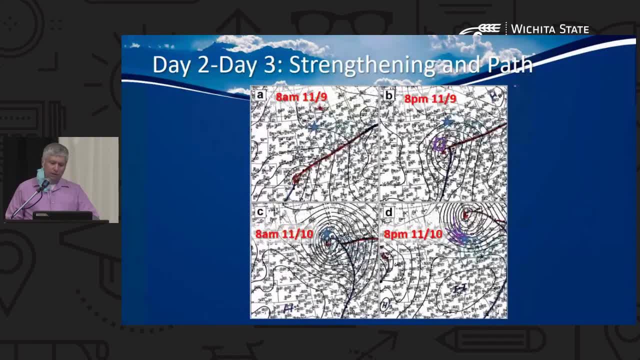 behind the system as it passes. you know it's going to. you know your temperatures dropped off a bit. It's a cooler evening. It looks, I believe, by you know evening. any precipitation that had fallen was already passed. You're going to be getting clearing behind the system. It's definitely. 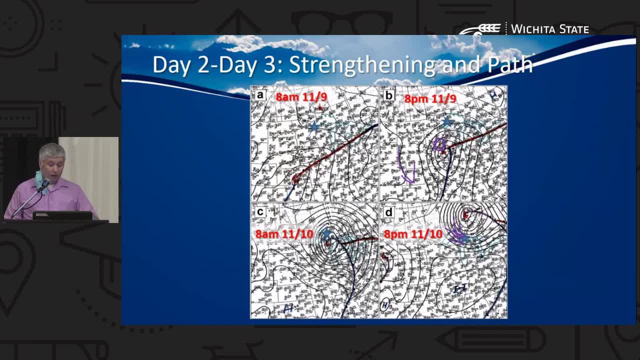 going to be a little bit colder on the 9th than it was on the 8th overnight, And then, time you get to the 10th, here high pressure has built in- It's going to be, you know, kind of a chilly start to. 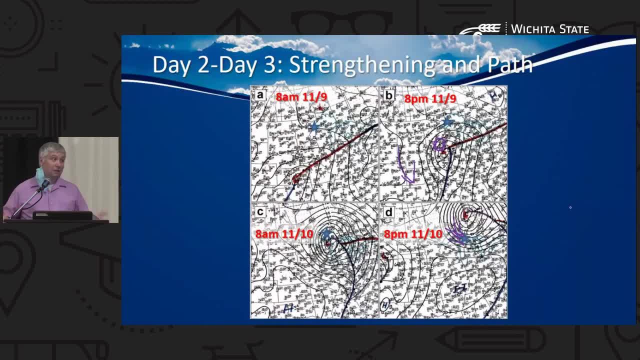 the day but clearing skies, probably a really nice day here. I didn't look specifically back at the records from you know the hourlies or anything on the 10th in 1975.. Believe it or not, some of that information, especially this internet age, is a. 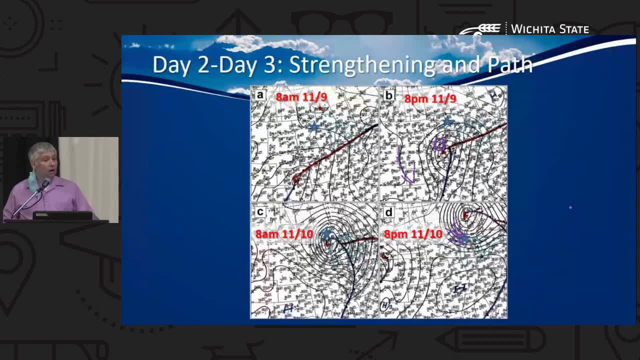 little challenging to dig back out in terms of what the hourly temperatures and things like that were, But it would definitely have been kind of a cooler day but a fairly calm day across the Central Plains on that same day that the Edmund Fitzgerald was getting buffeted across. 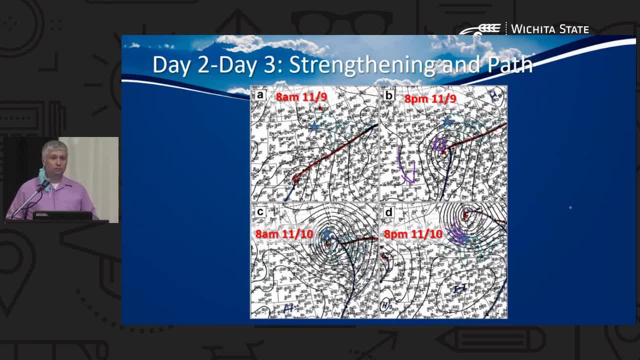 the Atlantic Lake Superior. Other questions. Yes, Yes, I probably I was going to. I was so afraid that I was going to run real long in this first half that I cut it off, but I was going to play the song, or a tribute video to the crew of the Edmund. Fitzgerald. But yeah, But 26,, what 29,? yeah, 29 souls went down on the Edmund Fitzgerald, Aging in range from 21, was the youngest and the oldest was the McSorley, the captain, 65,, I believe. 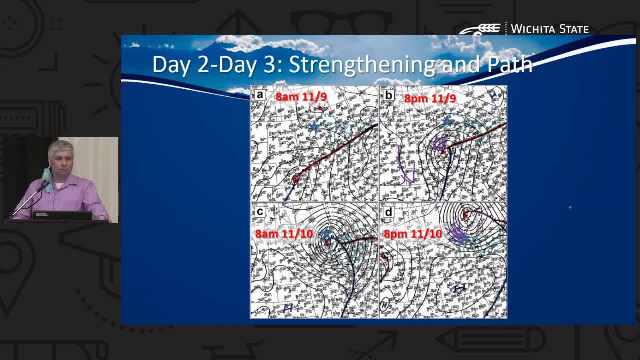 was his age And most, and except for the newest people on the ship, a lot of most of the crew was quite experienced. Um, some of the uh reports, uh after the the accident, uh, former crew members that. 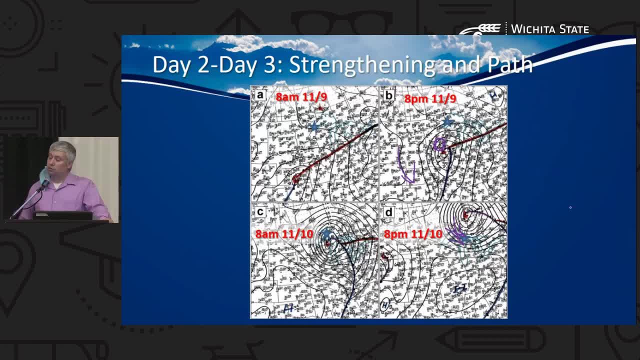 had been on the ship did, and this is what kind of fed into the uh theories that said that the ship had been uh poorly maintained. Uh, some of the former crew members were were attesting to that- is that the upkeep 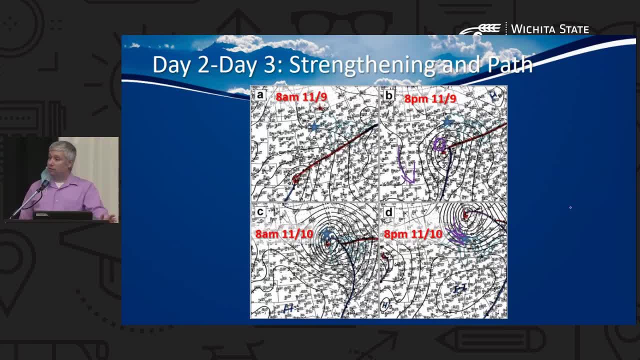 of the ship wasn't what it should have been, and things of that, uh, nature, And again, well, that may well have been a contributing factor. Um, the common, the, the, the more commonly accepted theory at this point is that, um, 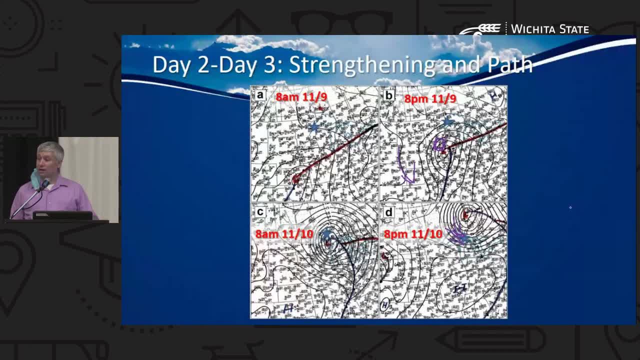 frankly, the Fitzgerald was just kind of in the wrong place at the wrong time. I mean, we, we take it for granted today just how much information we have in terms of the atmosphere at any given time. Uh, there was very little um that they had necessarily to work off of. uh, to know uh. 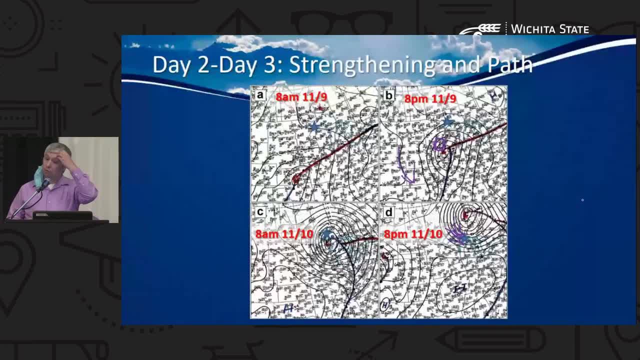 uh, where they were? Uh, there was very little information that they were necessarily relative to where the most intense um uh, waves and winds and things like that would be. Uh and again, the radar had been knocked out on the. uh. well, both radars cause there. 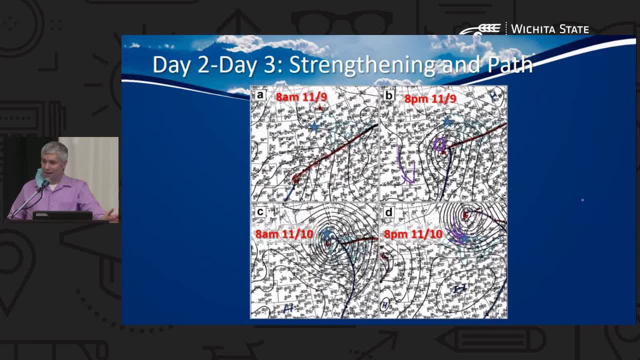 were two of them on the Edmund Fitzgerald, and they were both knocked out. Um and so again the ship was in the wrong place at the wrong time, kind of sailing blind, which was a really bad situation for that to uh ship to have been in. 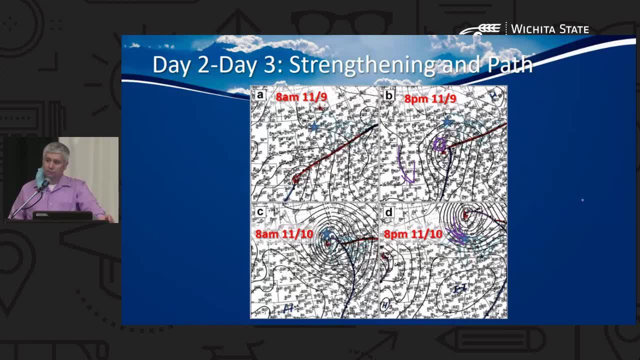 Uh and uh. Arthur Anderson, which was nearby uh, was trying to do the best that they could to help the uh Edmund Fitzgerald along, But I mean they were about 10 miles away. There's only so much that they could have. could do as well in terms of providing guidance. 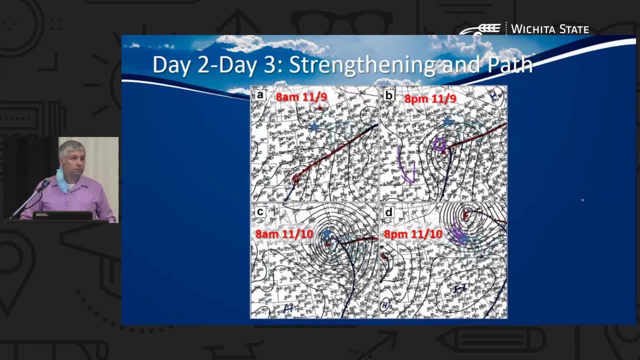 Yes, Yep, Uh, yeah, we, we do believe that it uh, that that storm uh, and there's no good satellite imagery to to show that that the little fish hook, uh, uh, uh. that we saw in the 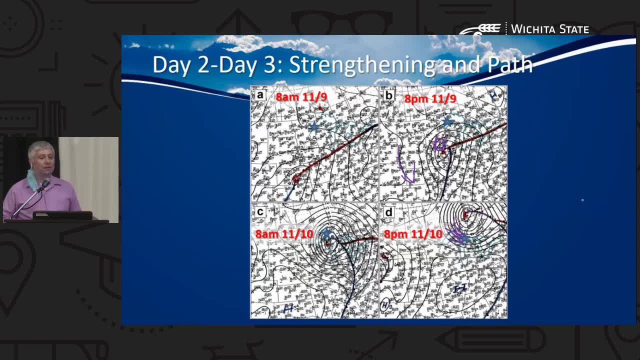 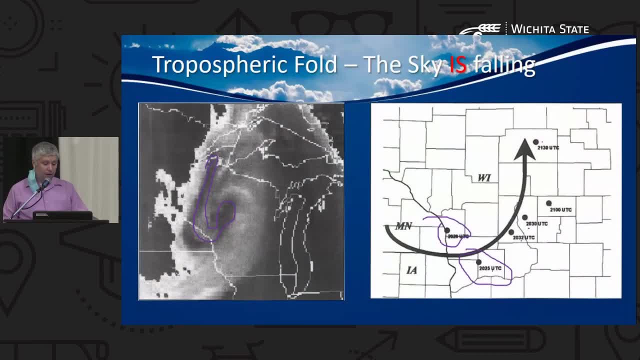 on on that one, you know. so they would not. they would not have had an idea at that point because, frankly, at at at that point, the idea of this sort of tropospheric fold really hadn't been fully understood. 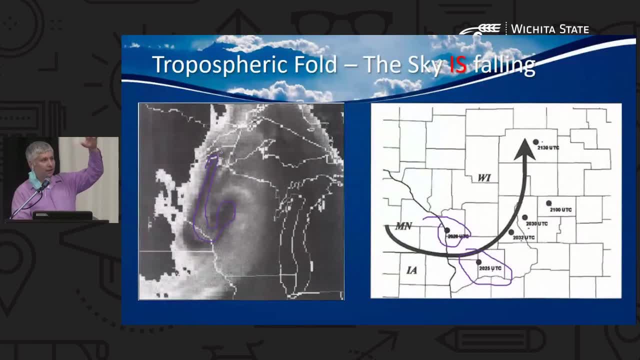 Um and so. so yeah it. it literally is sort of like the atmosphere was sucking down on itself over a really small area and where that happens- kind of like, you know, in another mesoscale type of situation, in a tornado, where you have a real intense, tiny, tiny low pressure, 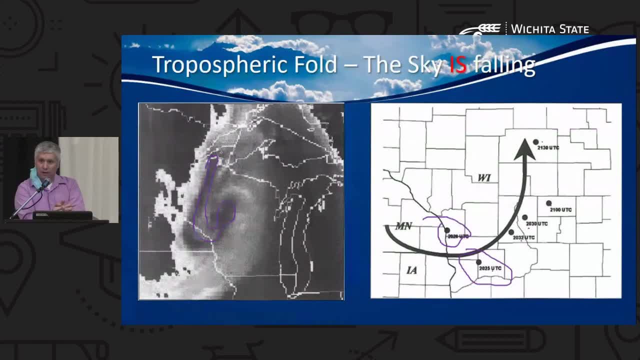 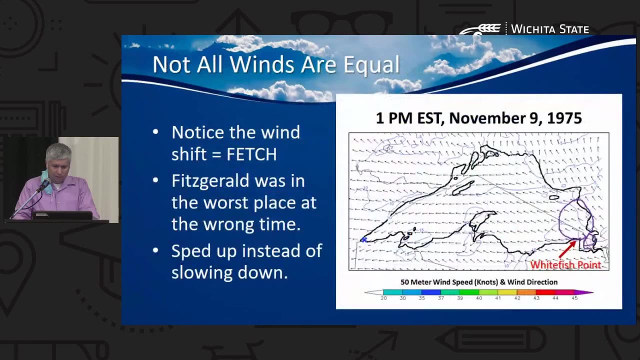 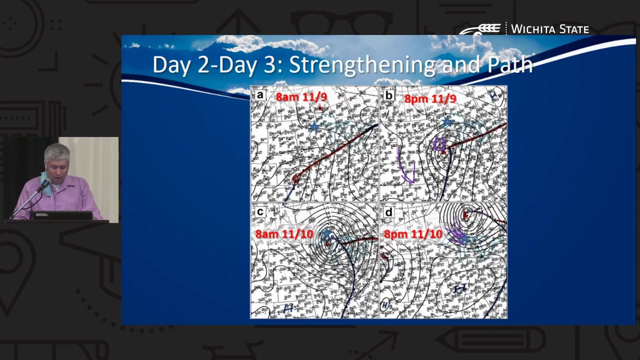 system, which is what a tornado is. You get really really high winds right there, Yeah, Um, let's see here. Uh, I don't think I have that on here. I certainly knew it back in the day, but I'm not a hundred percent sure what the uh uh, what the the uh. 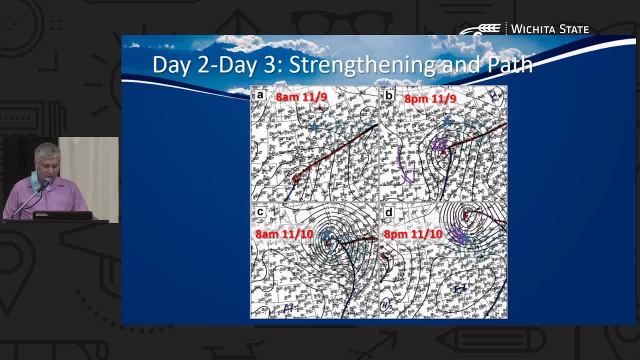 between, uh right about 11,, uh the right here in C. that's where your pressure would have been dropped off the most. This is where the system is at its mature point to starting to uh move toward just kind of cutting itself off. 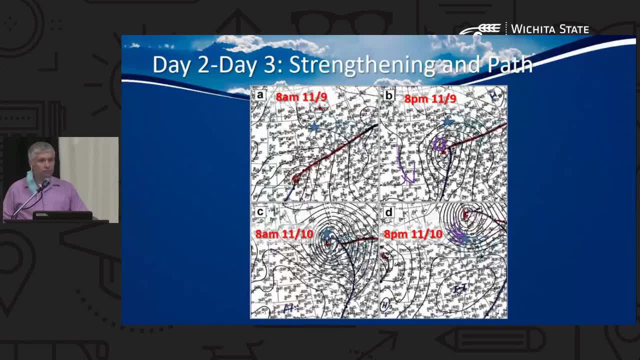 and falling apart. Good questions, Uh, other other uh questions. Well, if anything, uh, any additional questions come up about this? uh, please, uh, don't hesitate To let me know. that was uh uh, as pretty dense information there, Um uh. so if you need some, 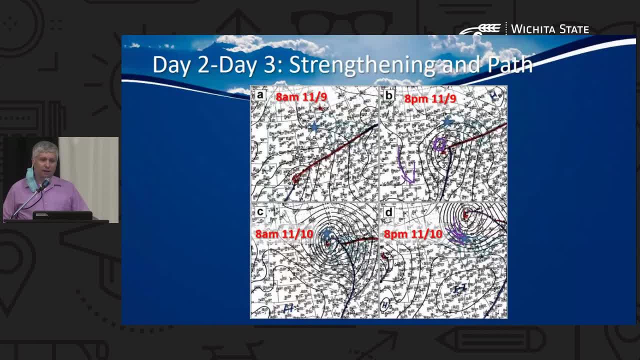 clarification please let me know, Uh, I try to present that as high level as possible, but it gets. it would get pretty intense into a multiple class periods pretty quickly. Um, in terms of what physics, uh, physics wise, is going on, uh, as the the, the low intensifies and things like that. 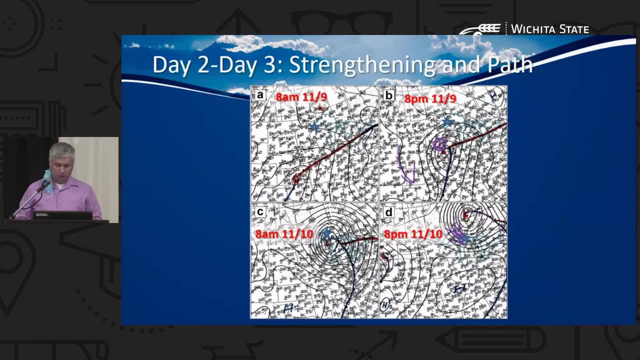 So I think, without further ado, uh, we will go ahead and take a. oh, I shouldn't have hit that. Okay, It's fine. Uh, we'll take a break. Um, it is one 59.. So we will come back and get started. 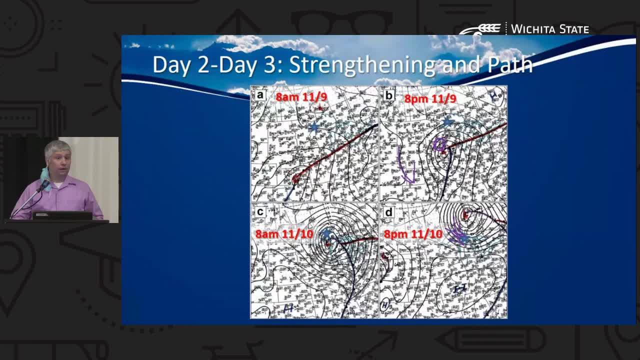 right at two, Oh nine. So, and if any of you, over the break, uh, have questions, you can come up to me. Um, and remember, at the end of class I may have to cut out of here a little faster than. 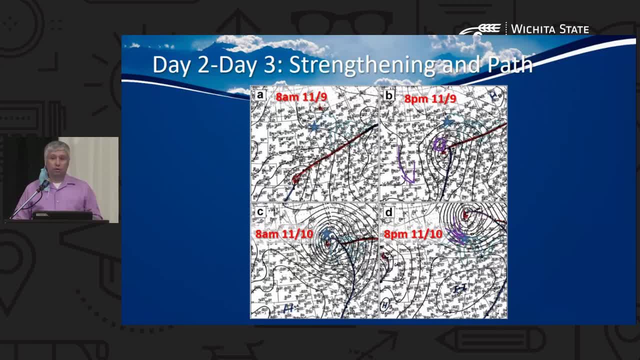 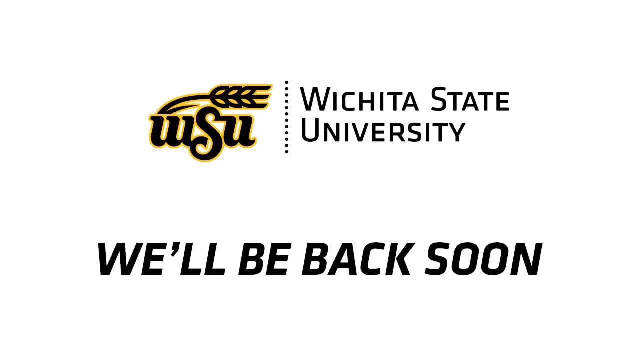 with the other class periods. So, um, if you don't catch me, uh, please get in questions and I'll I'll answer them by via email for you. Thanks a lot, Thank you, Bye, Bye, Bye, Bye. 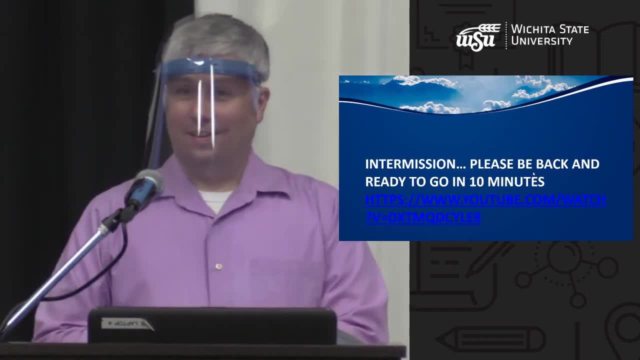 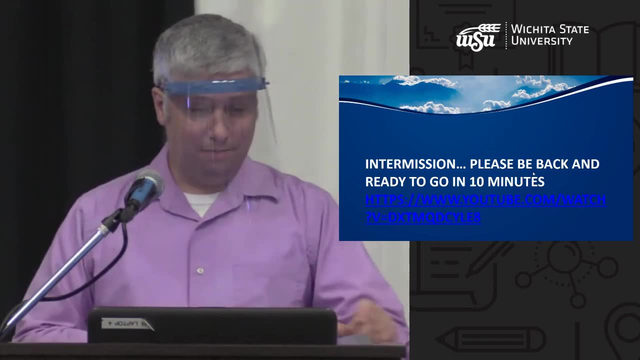 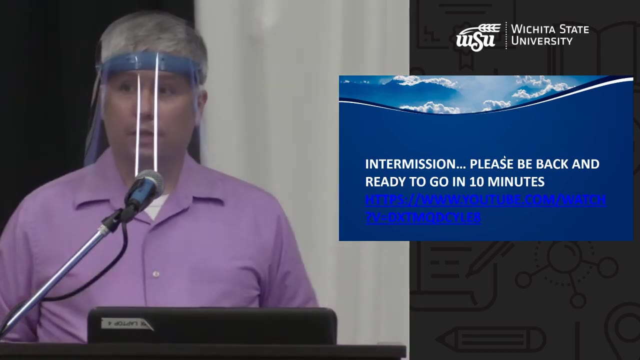 again. I have been uh, uh equipped now with, uh, this high, high, uh, you know- technology mask here to keep me uh good and safe. Uh, well, also, hopefully not gagging on my mask, So uh, 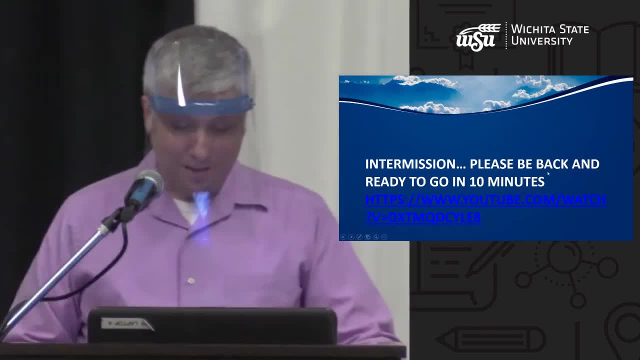 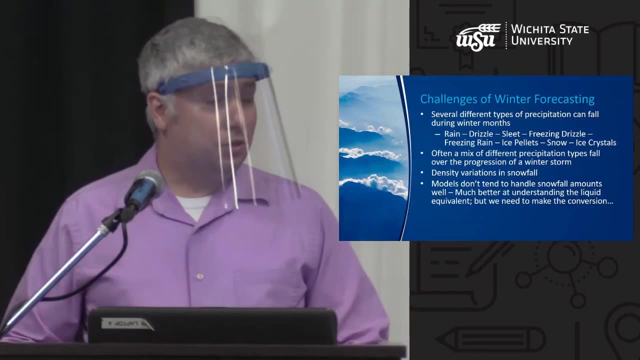 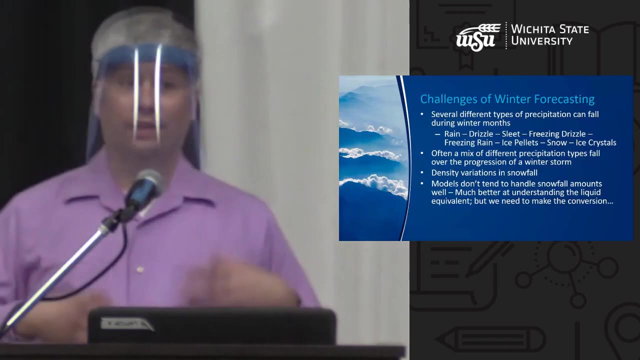 hopefully you're all able to hear me a little bit better, Um, and hopefully I'm not starting to hyperventilate, uh, over the second half of this class. So now we're going to start really getting into winter weather forecasting. We've explored, uh what those mid latitude cyclones. 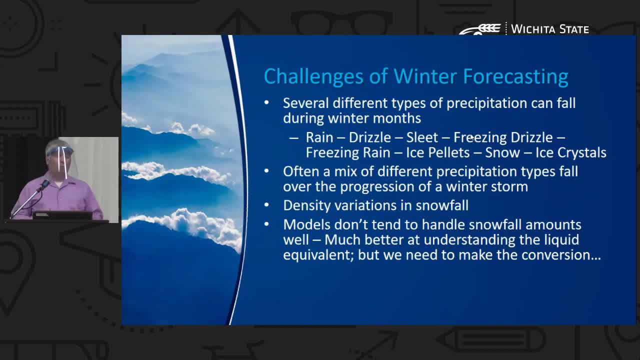 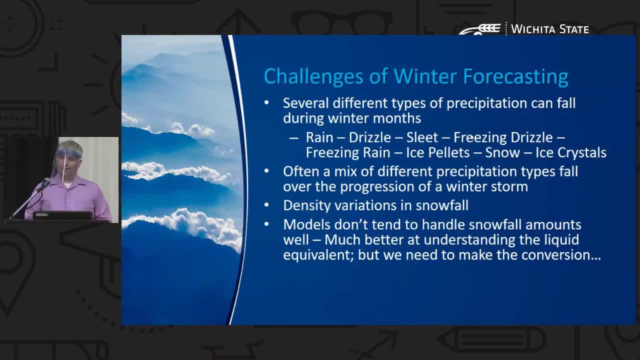 probably the number one reason why it's so hard to forecast is, uh, you know what's the thing that everybody thinks when, um, you know when, meteorologists forecasts: oh, it's going to be two to four inches of, uh, snow. Oh well, I didn't get two to four inches of snow. 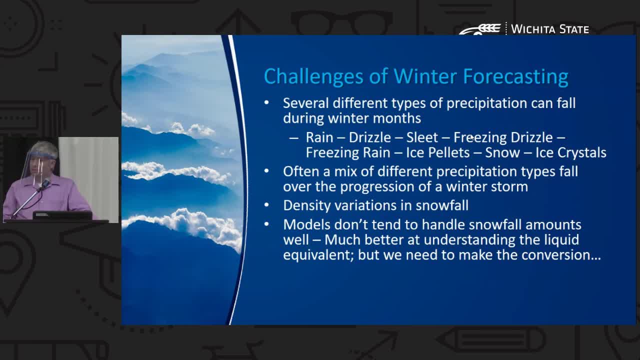 Barely snowed at all. Um or uh, you forecasted snow and location gets. uh, starts out with freezing rain for the first few hours, uh, before switching over to snow, And so there's hardly any snow that winds up falling behind the storm, And then you wind up with an ice storm and people. 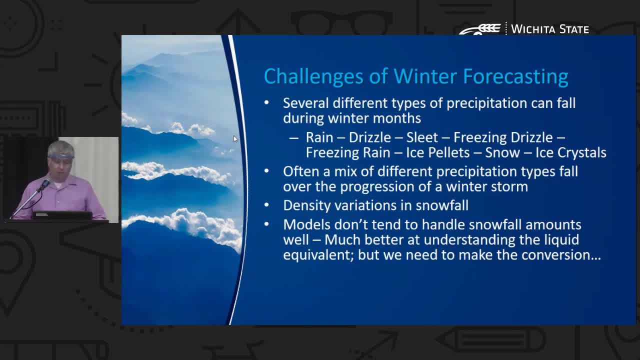 sliding off roads. Um, the the big challenge of forecasting in the winter is the fact that different types of precipitation will fall at different times. Um, and it all depends on not just what's going on at the surface, but it also depends on what happens. 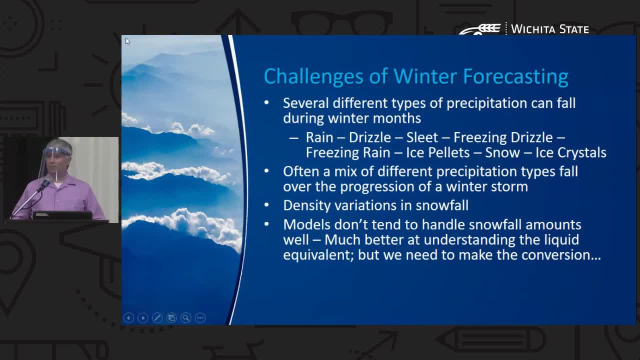 above the surface of the earth, And so we have to look at all the three-dimensional atmosphere and understand all of that and also understand how it's changing over time, to really have a full comprehension of what is going to fall at a specific point or across a certain area. uh, 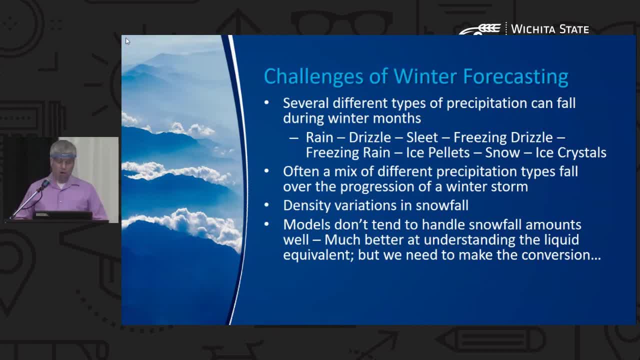 as we are, um, uh, have these storms coming across? Um, now, the other thing is, you know, like I kind of alluded to, usually when we have a storm come through- uh, we've all seen this before- It's not necessarily one type of precipitation that falls. 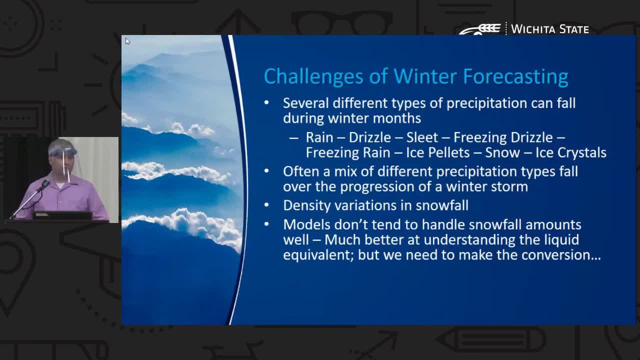 as the storm comes across the area. Uh, typically we may start with a little bit of rain, and rain maybe turns over to a little bit of freezing rain or freezing drizzle and eventually kind of becomes sleep for a little while and then becomes snow. Uh, sometimes that transition happens. 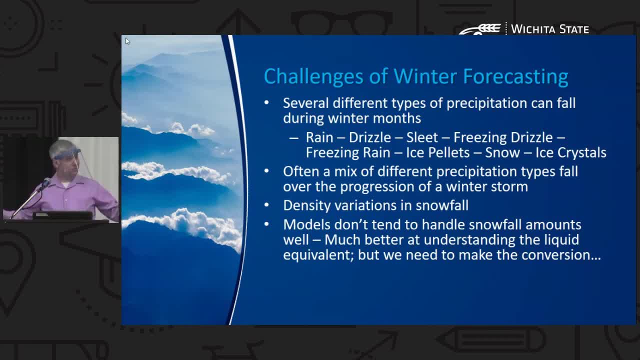 very quickly, Uh, and then it becomes snow. Uh, sometimes that transition happens very quickly, Very fast, And sometimes that transition gets drawn out, depending on how rapidly the system is moving across the area. Uh, another thing is the density in the snowfall. uh, depending on where a 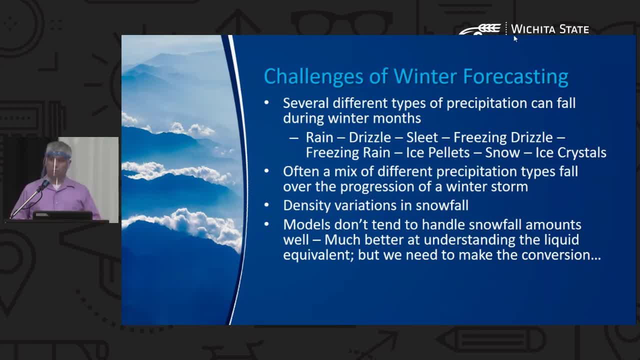 system originates uh and comes through your area, uh plays a fairly significant role in the uh, the type of precipitation you're going to have and how dense that precipitation will be Uh. and finally, as sophisticated of models as we have today, um, they still, to this day, don't. 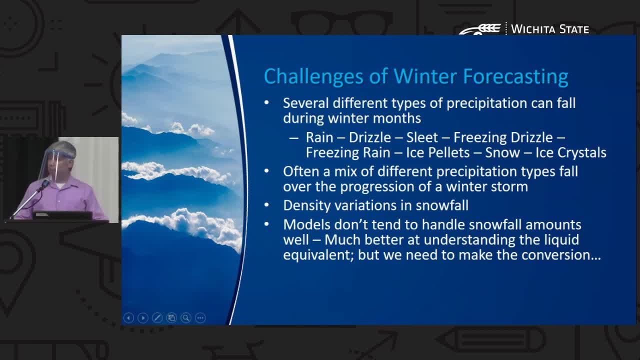 handle snowfall particularly well and freezing precipitation particularly well, because, again, it's so complex as to what's going to happen. as specific a point, because it all has to do with how thick your warm layer is versus your cold layer and everything else. Uh, our models. 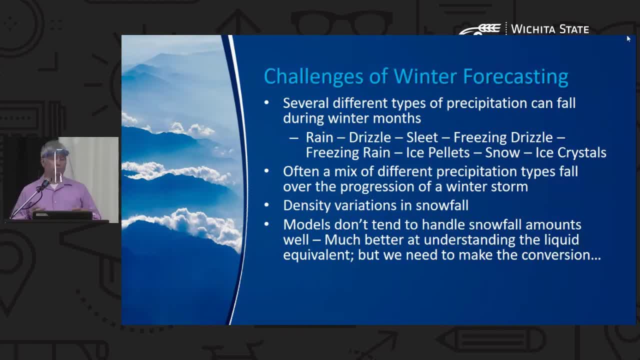 are pretty good At particular uh forecasting and understanding how much physical moisture is in the air at a specific point, And that is helpful information. That's why during the summer we have- and you know, you may or may not notice this- We're actually pretty decent at forecasting the uh. 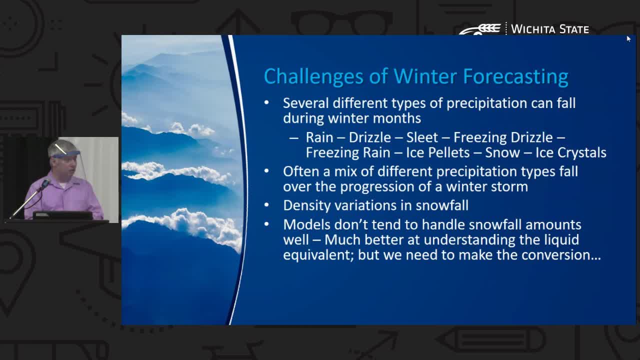 amount of rain that might fall, uh, at a, at a location. Typically we're pretty good at that, except in real extreme flooding- Um, but when, once we start bringing in that freezing component, it gets a lot harder to predict exactly how much physical solid precipitation will fall at a point, because how is it going to? 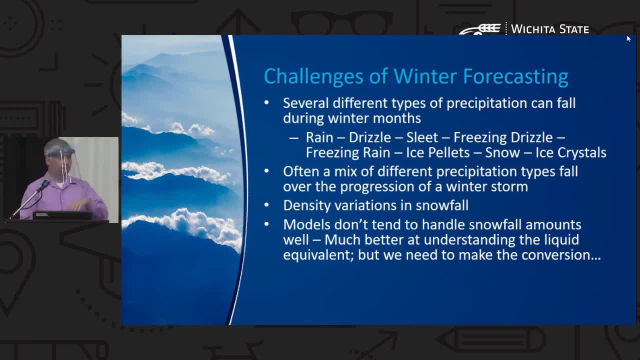 fall. How is it going to pile up? Um, if it falls really heavy, it's going to be smaller depth than if it falls really light and fluffy, So it and some of that winds up being even perception at your specific location. So it's going to be a lot harder to predict exactly how much physical 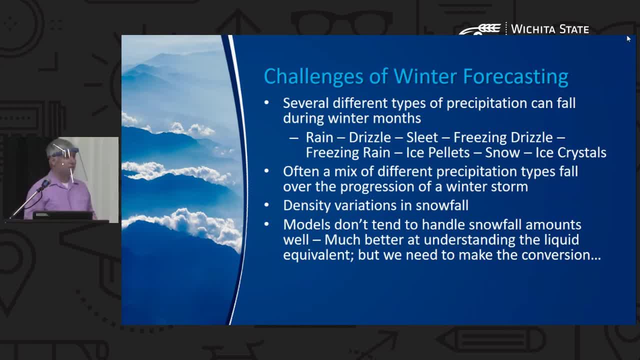 snow will fall at a location where there's some winds. Did it pile up some snow drifts, uh, at a location versus, uh, you know, not blowing the snow around? So there's all these different factors that play a huge role in how much snow fell at your house, basically. So we're going to sidestep. 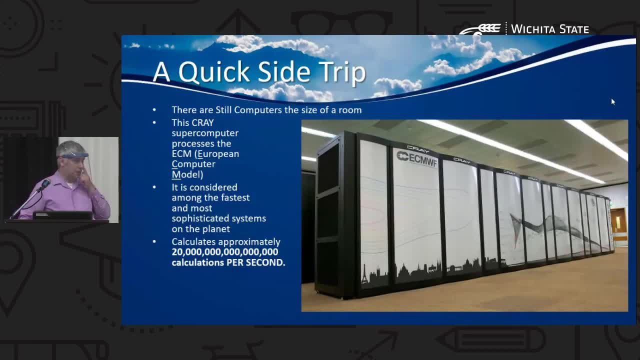 here quickly. We've talked a little bit about models in previous classes, Um, but I it occurred to me as I was putting these slides together, I hadn't really shown you what a? uh a computer that runs a? uh a model looks like, um, in the early days of computing. 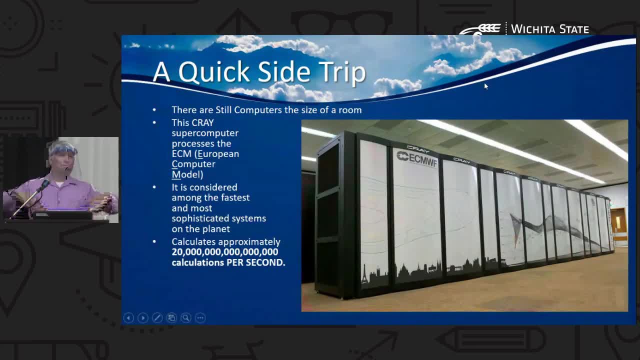 uh, you know our early computers. there was a big as a room. Well, those computers still exist. They process a lot more than what the computers in the uh uh sixties and seventies processed. Uh, but we still have these ginormous uh Cray computers, Cray being kind of a brand name. 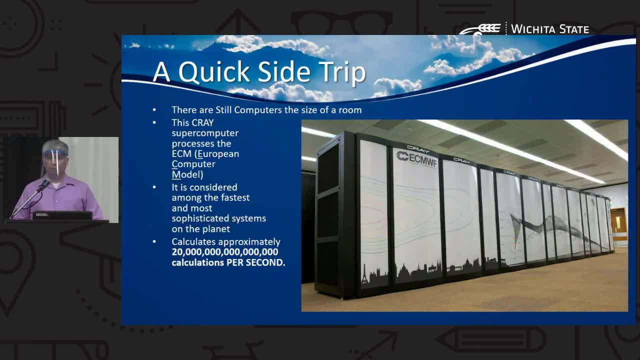 That makes that special, makes these massive, massive computers with huge, huge computing power. Um, and this in particular, as you can see on the side of the uh, uh, this row of uh systems, uh, it's the ECM WF, that's a European computer model weather forecast. So this is the uh. 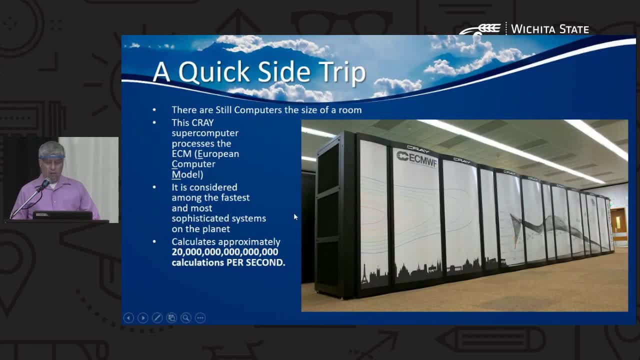 computer- actually it's really still just a part of the computer- uh that processes uh the ECM model every uh. well, it it does uh some of the work every four hours And then uh, they've. 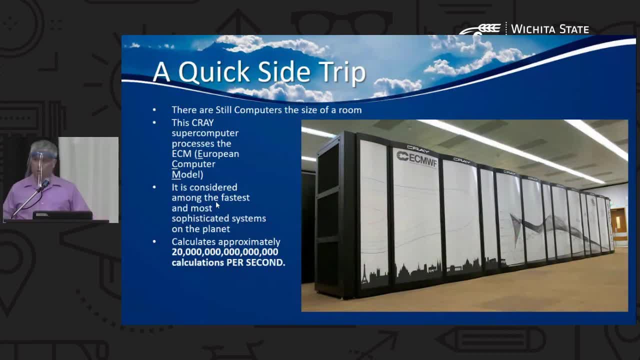 got different uh sets of models that it creates over the course of a 24 hour day. Uh and it. this is this computer in particular. uh is basically considered the- you know, the most sophisticated computer on the planet. Um, it's got incredible processing power. It can take in. 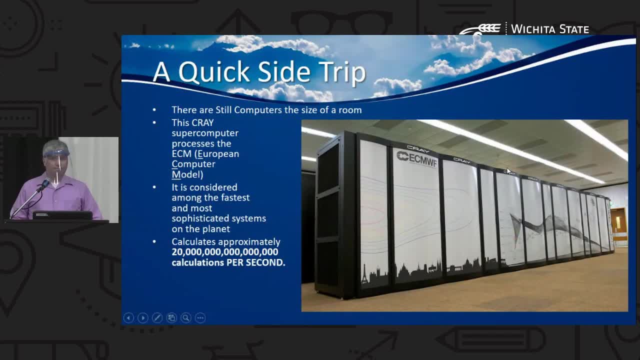 uh, all sorts of data and calculate every possible thing you can think to calculate, Uh, and it does 20 quadrillion, um, uh, approximately 20 quadrillion calculations every second. And yet it still takes four hours to process and process all the data it takes in and kick it out in a 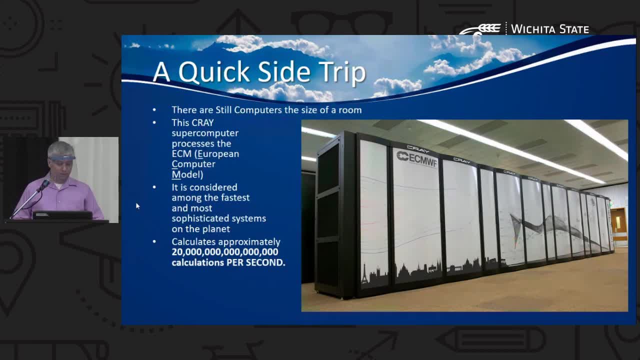 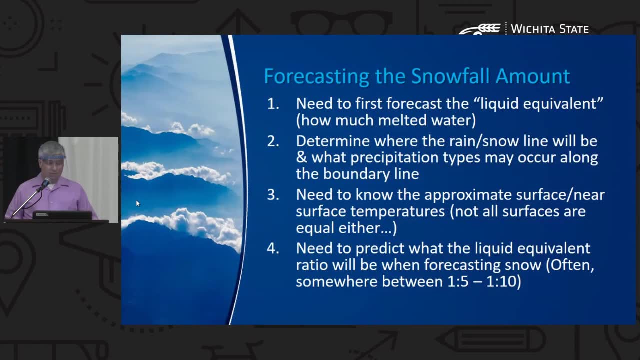 a digestible forecast, And yet, in all of that, of course, it's still not great at necessarily forecasting how much snow is going to fall at your house. Uh, and that's because there are several steps that are involved. Um, first, we need to uh be able to forecast what the liquid equivalent is. 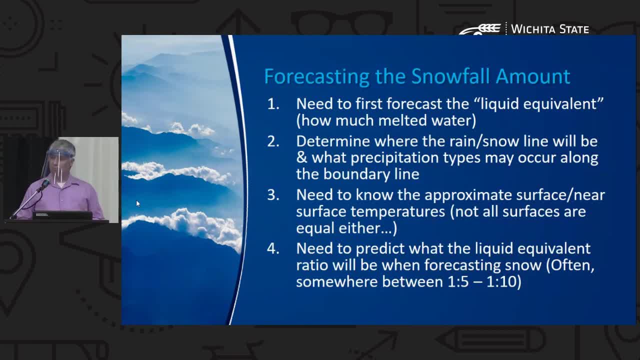 that's going to fall at a location. Now, that part usually, uh, especially when we're in about 12 hours of when that system's going to hit you. usually it's a pretty good estimate that we've got, But the problem is, of course, as I alluded, 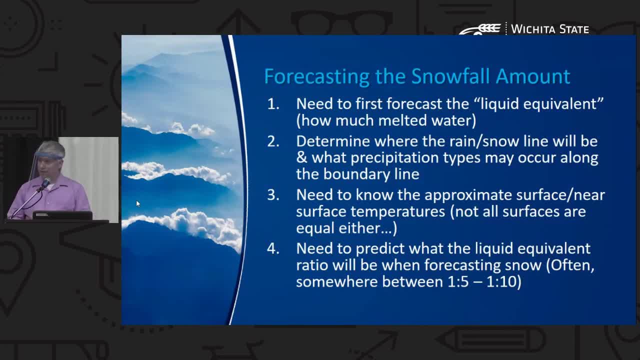 to earlier, we've got to determine where that rain and snow is going to fall and what kind of precipitation is going to fall as well, And that's where we've got to have a, uh, a pretty good feeling for what that depth of the atmosphere is. Um, and then, uh, you know, uh, we also have to 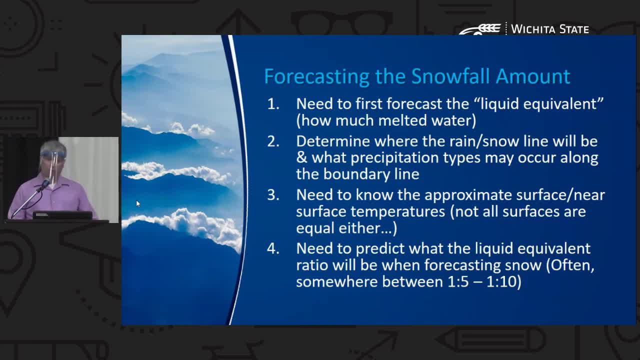 forecast how fast that boundary line uh, the cold front, warm front, occluded front, how how fast those are going to be moving. Um, usually, uh our general understanding uh and experience with uh synoptics and and how the waves move, you can get a pretty good. 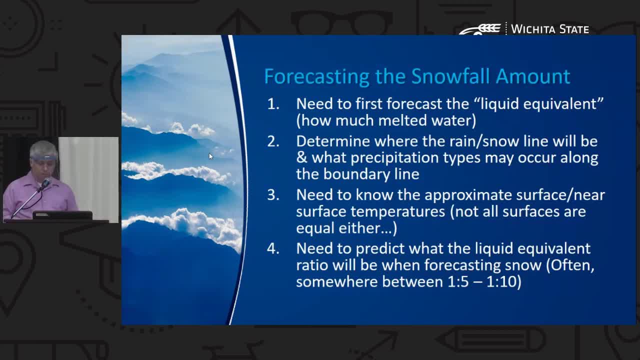 short-term feel for how fast or how slow something's going to move, but uh, it's not. it's certainly not perfect, even in, uh, the year 2020.. Um, and then we need to be able to again predict what the snow equivalent ratio will be. 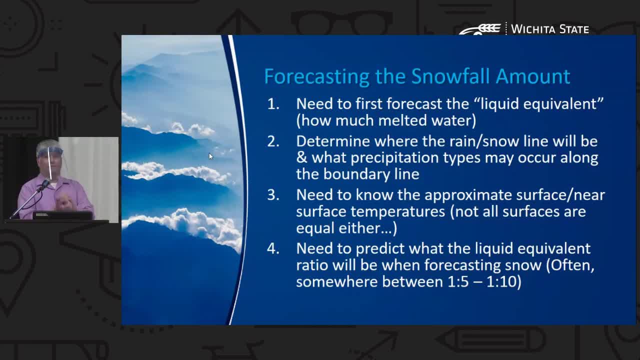 Um, you know, your, your very wet, heavy snow doesn't pile up the same way as your light, fluffy snow, And so when we're doing a forecast, uh, you know, across an area, I mean every, every winter, we see these graphics. 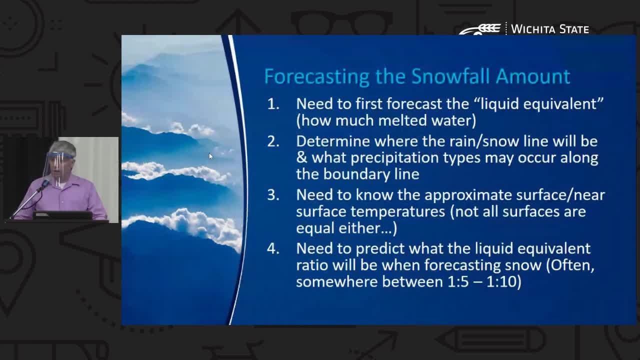 put up by our uh TV meteorologists uh, where they kind of hash in the areas of two to four inches, four to six inches, six to 12 inches. Um you, they're having to make that uh prediction. 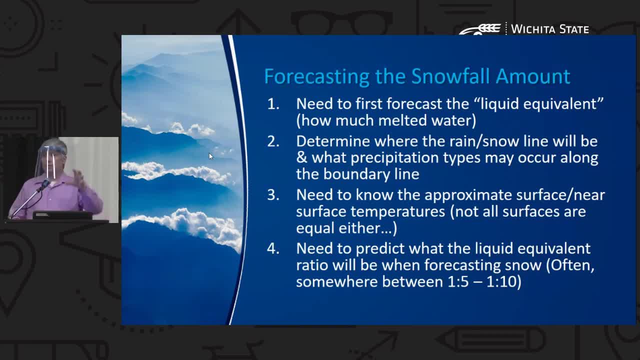 in their head of, okay, of this one inch or one and a half inches of water that I know is going to fall out of the air, how much of it's coming down- uh, down- on a specific location, And how dense is that snow going to be? Now we can get some general ideas based upon where the 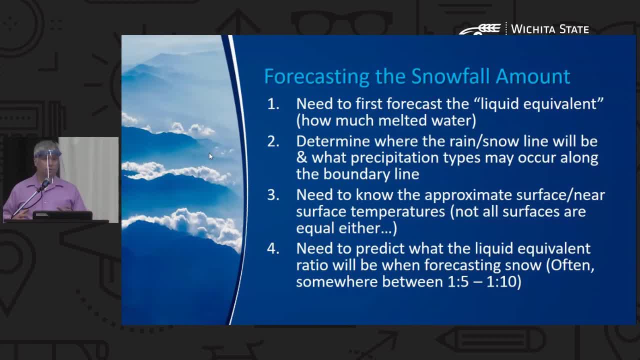 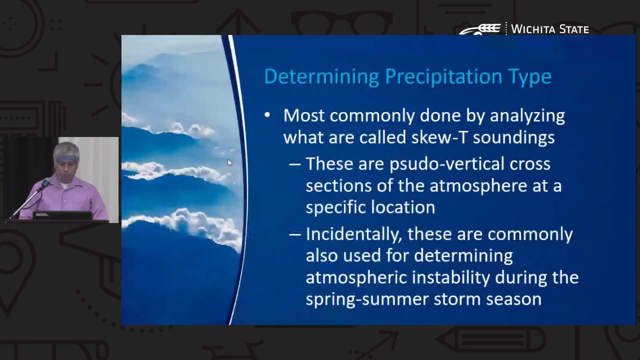 low pressure systems formed and how much access to warmer, moist uh air that uh the system's going to have as it's coming across the area? Uh, but it's certainly an inexact science as to exactly what that uh um density of the snowfall will be And, of course, if that's not complicated. 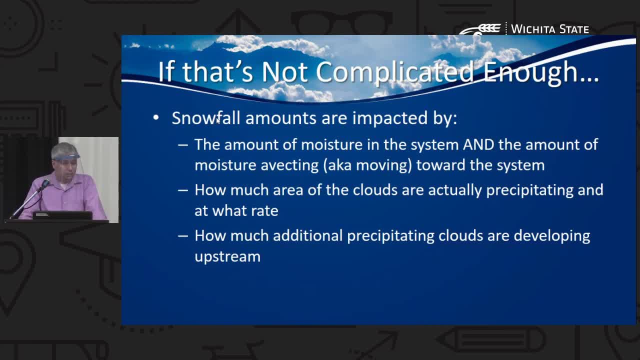 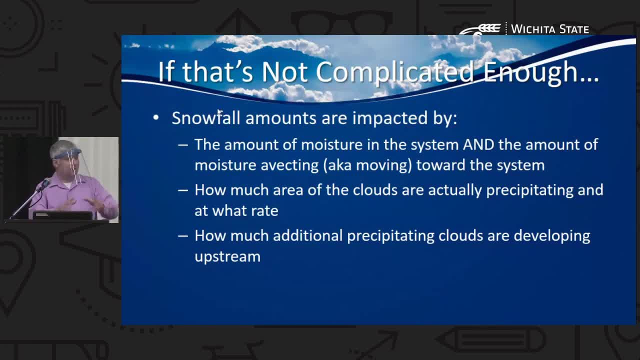 an area of increased moisture. that it's. the system's going to pick up even more moisture over you know a 12 or 24 hour period And you know how. what's the rate that that moisture is going to come out of the clouds? Uh, it doesn't all come out at one time. It comes out over a 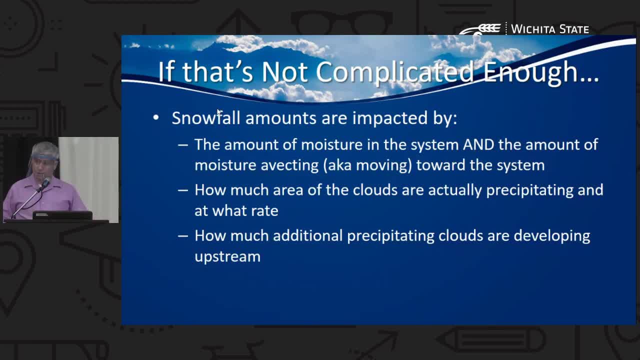 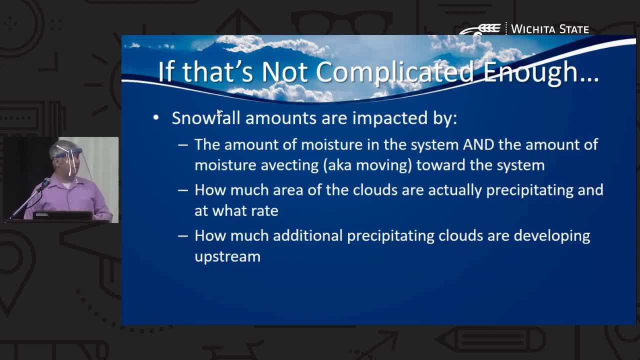 evaporation is going to happen out in front of the system that the system's going to move into and collect that additional moisture and then drop that as well. So there's a lot of little details that we have to uh process as meteorologists, uh over our forecast period And uh if it. 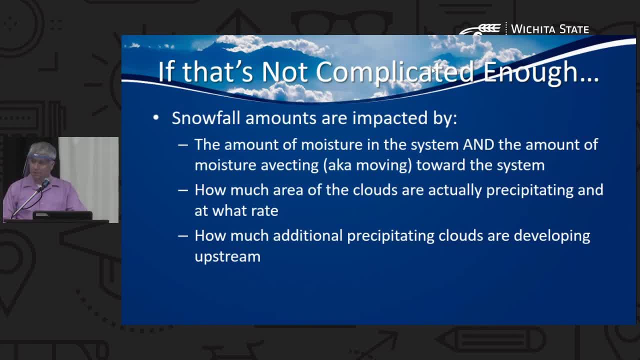 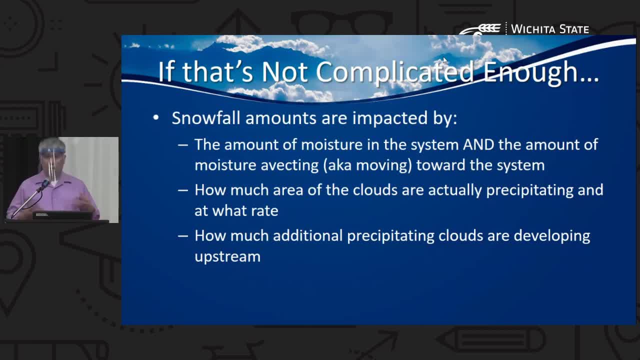 four hours just processing all of that information, just taking in, uh, all the data and just thinking through: okay, here's the information I have- and applying my own human understanding of meteorology to that information to come up with a forecast, And hopefully I do it. 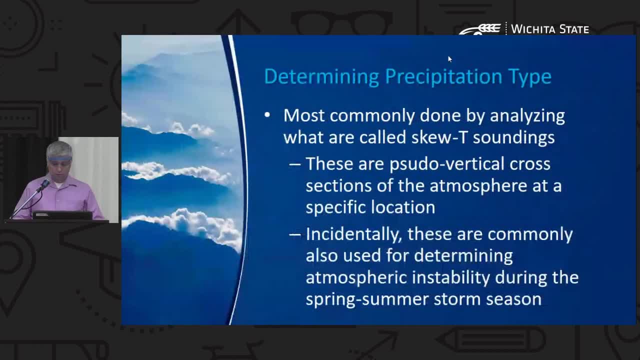 Okay, So I mentioned the fact that again, we have to not just be looking at that surface and what's going on at the surface, but we really need to know what's going on above the surface, especially in the lowest, about one kilometer of the atmosphere. Um, because that's what's. 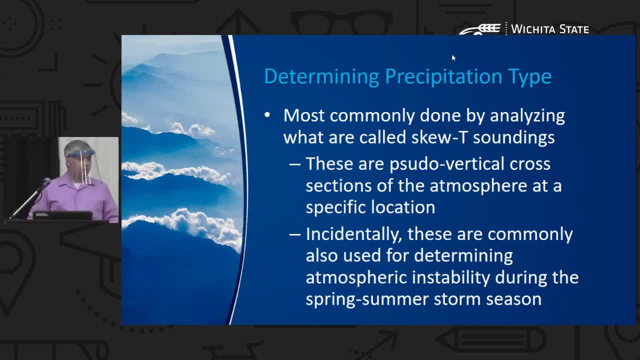 going to tell us what type of precipitation is likely to fall at a point, but here's where it gets, uh uh, interesting. Well, we don't necessarily know what the vertical temperatures are above us at any given point. Um, the you probably may have seen, um uh images of meteorologists going out and launching 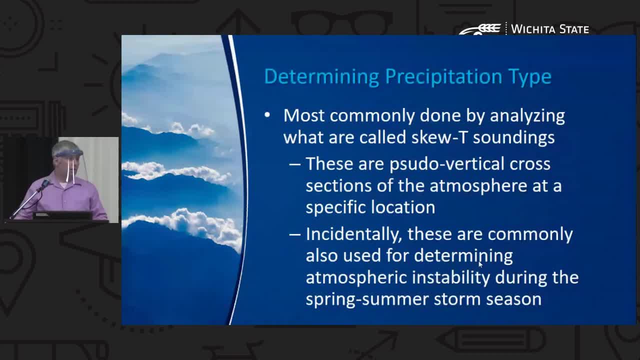 balloons uh at their weather service office. That happens about every 12 hours uh across the country. Uh they sent, they let literally let go of uh a little instrumentation, uh packet that uh that uh measures the temperatures, that measures the humidity- humidity. 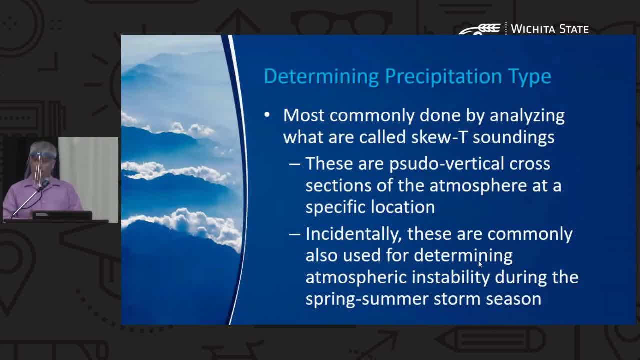 that measures the wind speeds, Uh, and that measures I can't remember. I said pressure, but pressure um at at all levels of the atmosphere, but that's only done every uh 12 hours or so. So we're having to use fairly limited data to uh along with our general. 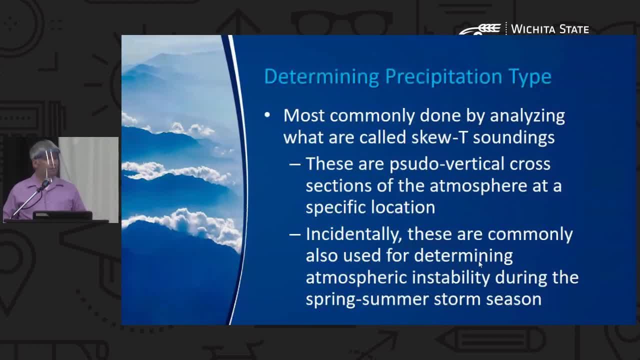 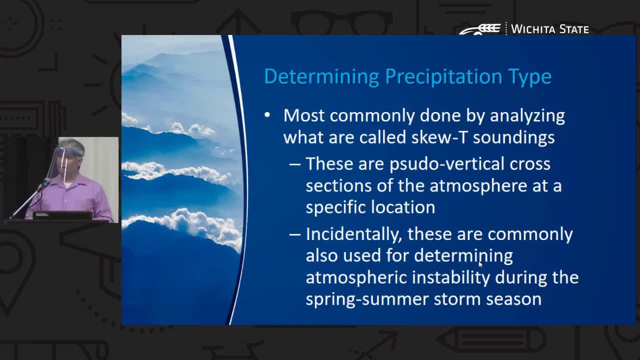 is looking like in order to ascertain how thick is our uh warm area relative to our cold areas. Now, I'm talking in terms of warm and cold uh, because we, if we go aloft into our clouds, it's a lot colder up there Our our uh precipitation in. 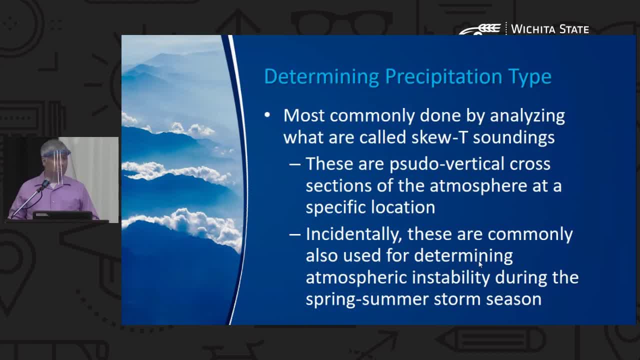 the clouds. uh, especially during the winter months, going to be all snow up there, but that snow is going to start coming down because of gravity. As it comes down, if you've got a frontal boundary, there's going to be some warm air being pushed up and over cold air. So we know at some 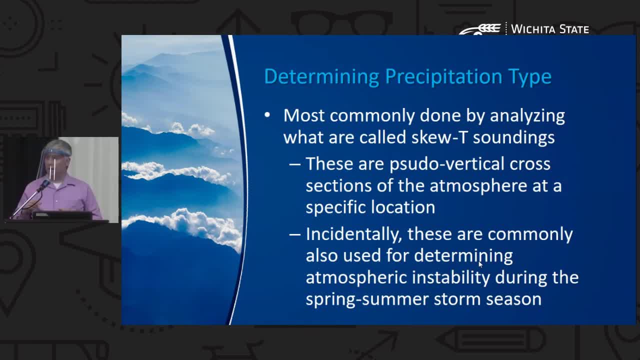 point it's going to come down through warmer air. Is that warmer air thick enough to melt the uh uh snow into rain? Well, that depends on how thick it is, because it doesn't immediately happen as it goes through that layer, And then how much cold air is right near the surface. that matters, because is it going? 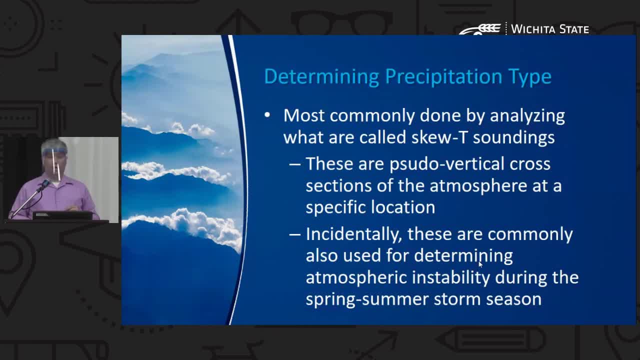 to refreeze the precipitation. And then what's happening at the ground? is the ground at, or below, 32 degrees? If it is, and you've got water hitting it, it's going to flash, freeze, And that's where you get your freezing rain. 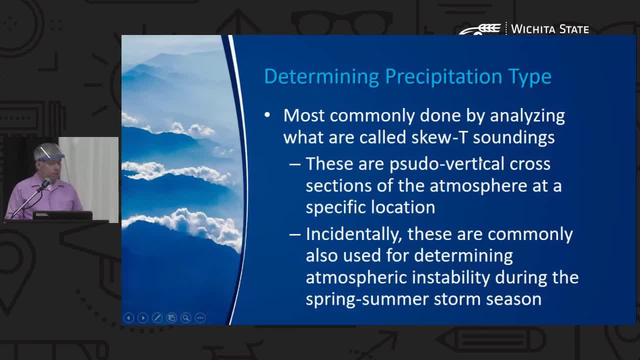 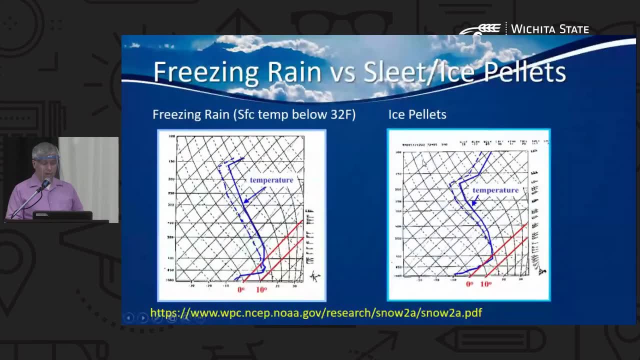 So we look at what are called the skew T. actually, it's really skew T. log P is what the full name of these uh soundings are called. Uh, these aren't the best uh uh pictures. uh, but they were. 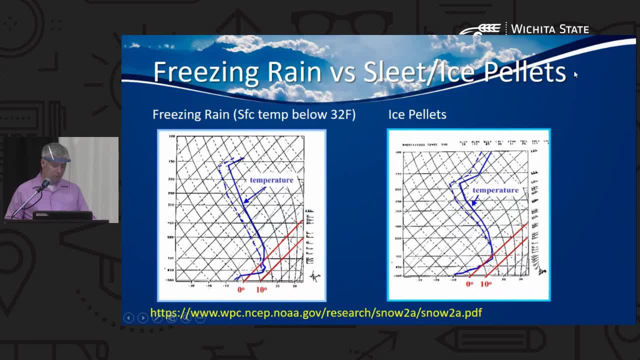 good pictures that I could pull to show. uh, what's going on? And the reason why they're called skew T log P's is at the bottom. here we have our temperatures and our temperature lines are going at an angle up, So you can see this in in terms of that, those red lines there. 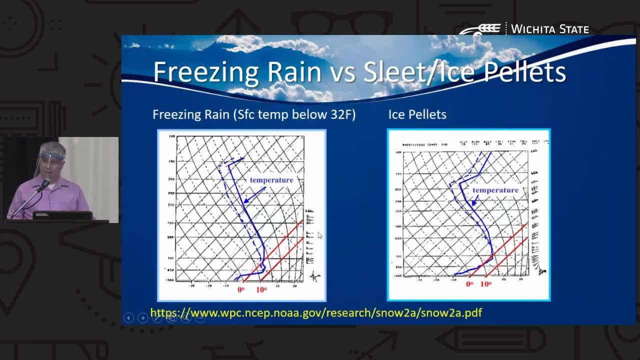 that's the zero degree line and that's the 10 above freezing line, And so, uh, and then the log P is the pressures, and the pressures are just going straight across. So you're seeing an equal pressure at those lines, at a specific point where you're, you're, uh, uh, 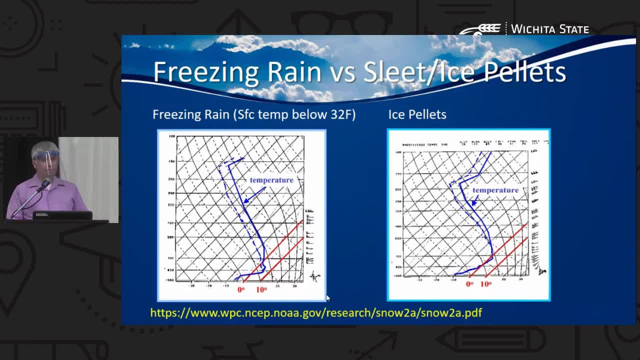 temperature lines are slanted. Now, why do we do it this way? It actually has a lot to do with, uh, severe storm forecasting and understanding how much energy is in the atmosphere at a given time. I guess a little bit beyond what I can cover in this class, but, um, how it fits for. 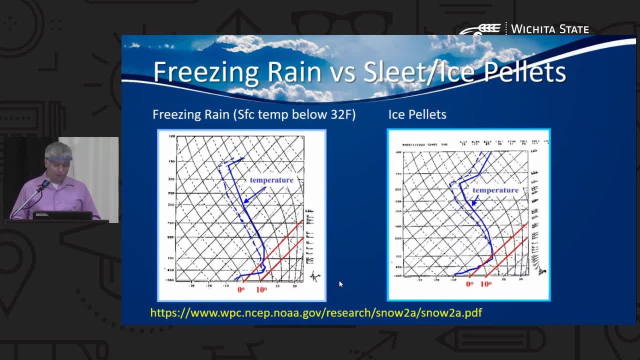 talking about winter weather is you can see the different temperatures at the different heights of the atmosphere. So, uh, you can see that the temperature has gone up into the atmosphere. So at the surface- and actually both of these uh images you notice- the temperature is below freezing. 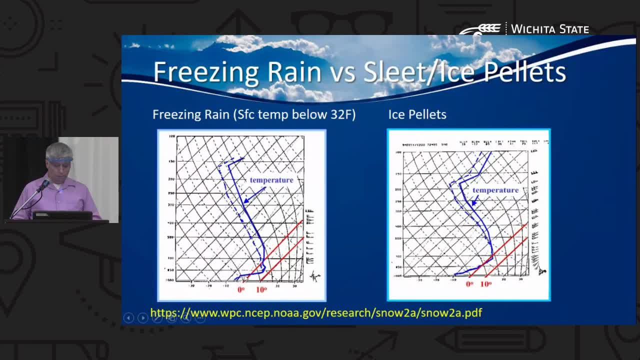 but as we go up in the atmosphere we're noticing that there's warmer air and it actually gets above freezing. uh. on the freezing rain chart here it's right around probably about 900 millibars, So that's uh still very close to the surface of the earth. Uh, and then on the ice pellets. 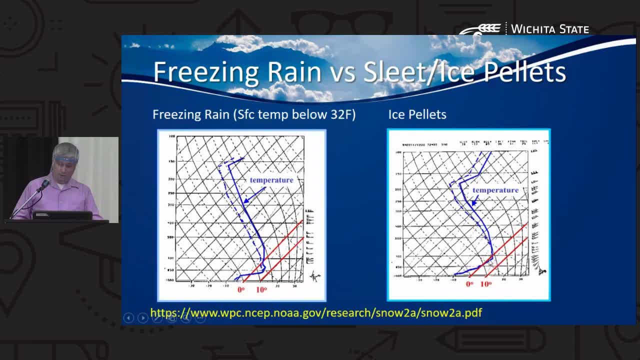 you see, it just barely wind up getting above freezing, And the reason that that matters is: here we've got a large, fairly large, area of melting going on, So the snow's falling down, And as it falls down, it goes through this warm area where it's above freezing. 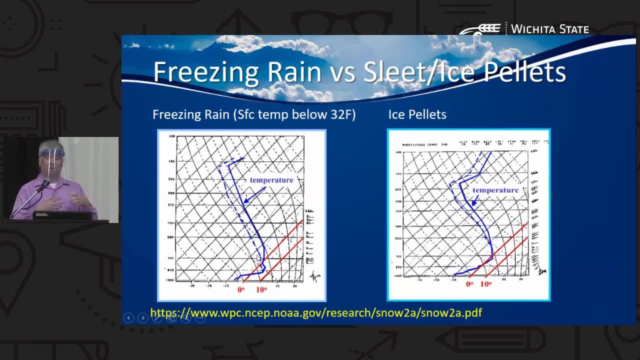 And so it's melting the rain into, or melting the snow into rain in that area. because it's thick, it can fully melt it, But then it goes into this fairly thin area right above the surface, which is not enough area for it to refreeze, And so, even though it's below, 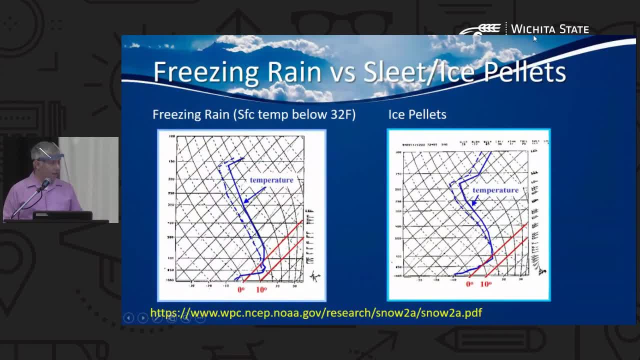 freezing at the surface, you're still getting rain hitting the surface. But because the surface is below freezing, you're still getting rain hitting the surface And so it's not enough area for it to go below freezing. As soon as it hits the ground, it flash freezes. That's why you'll get roads that. 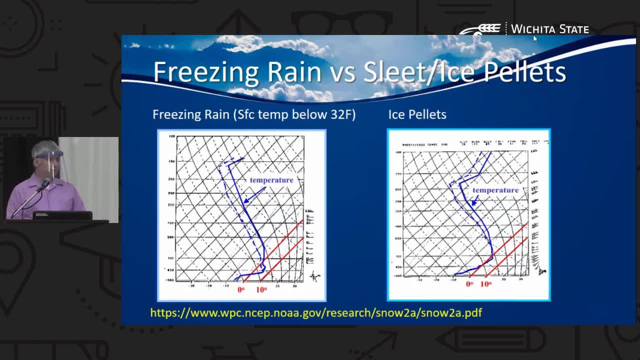 get real slick, real fast in a case of freezing rain, because the rain's coming down and immediately becoming- uh, it's immediately becoming ice as soon as it hits the surface, Whereas with these ice pellets we're getting the melting, but only a little bit. 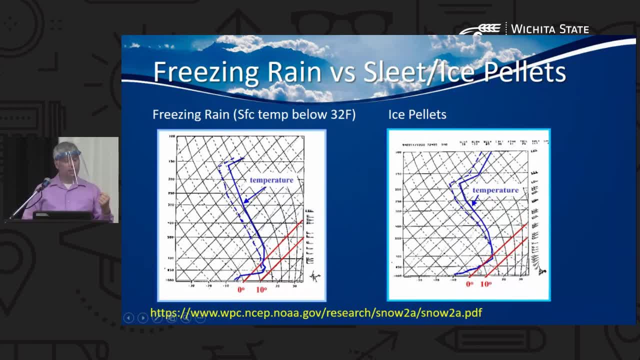 And so that's, and then then it goes through a much deeper layer of refreezing and it becomes kind of a pellet, And those are those are where it kind of almost hurt your face when there's a lot of wind driving it into you And when you're walking to your car. uh, you could feel it, It's all they're almost. 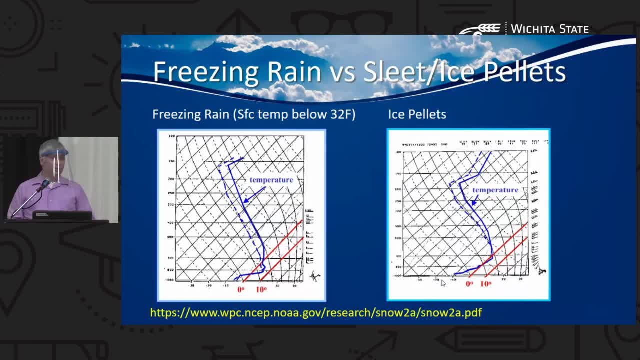 like a mini hailstones, but they're not formed the same way. Uh, hailstone would be formed because, uh, the ice is being pushed up and down in the atmosphere and collecting more and more water around it, uh, and, and you know, making a larger stone. that. 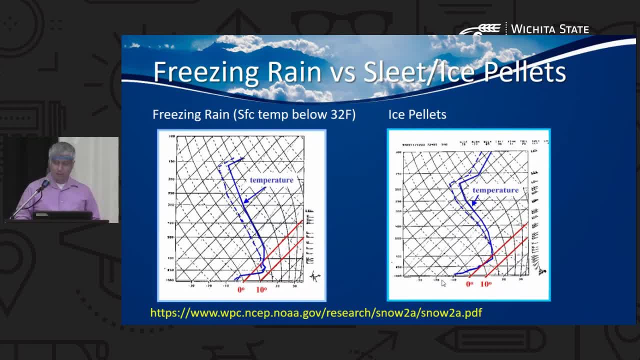 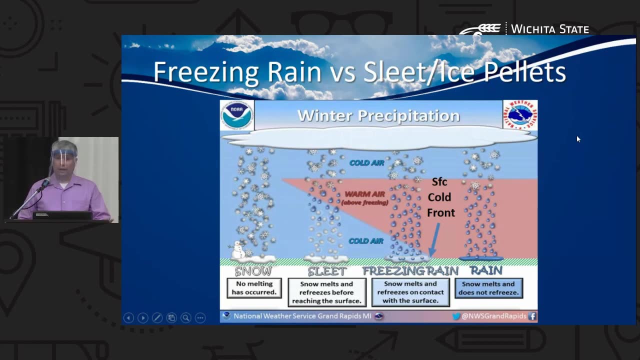 that eventually falls out of the sky, Whereas, uh, this is just one straight shot down of the precipitation. Now, uh, this. this is probably a little bit better of a graphic, uh, than looking at the skew T uh, log P soundings, in order to kind of. 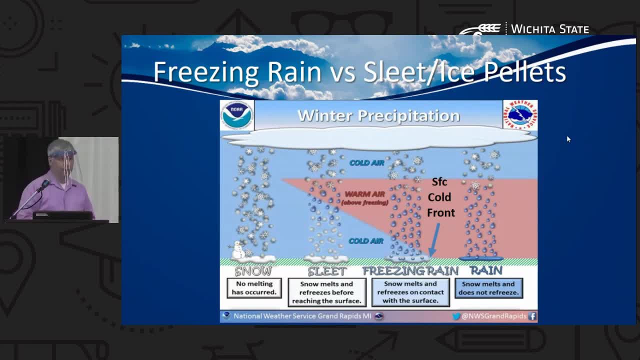 uh understand practically what's going on with the uh different types of precipitation. Uh, and you can kind of visualize here: this is our surface and that's kind of our surface cold front, right there where that cold meets the warm air. If you're out ahead of the uh surface cold. 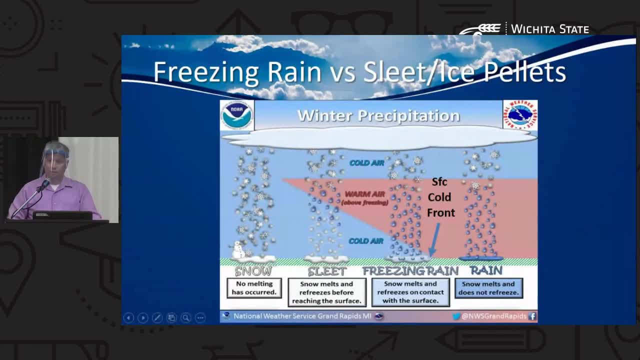 front. uh, everything that's going to fall is rain, because you're above, in this case 32 degrees Fahrenheit, But right behind that surface, cold front. you still have overrunning warm air at that location, And so you still have up above. 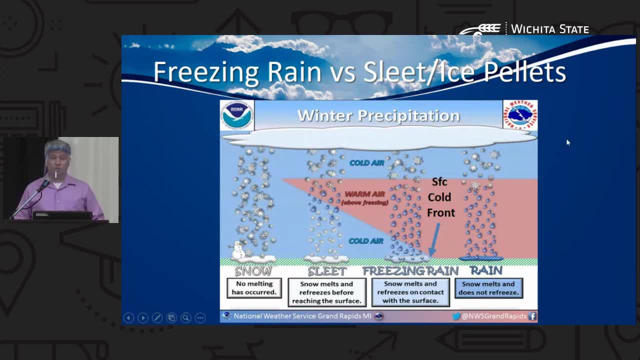 here it's still all that that uh, uh snow falling, And then that snow falls through this fairly thick layer of warm air. This is why, when you get one of these fronts that come by, one of these cold fronts during the winter months, you will often uh. 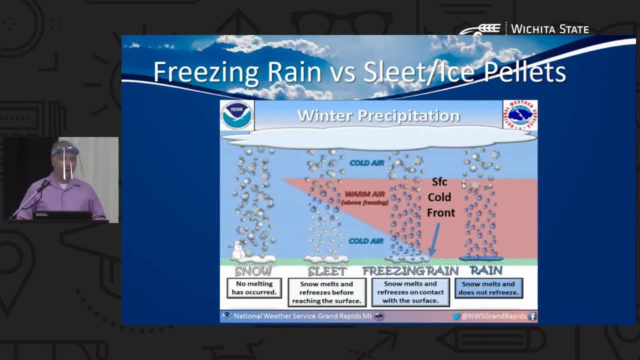 especially in the winter months, you will have a lot of snow falling, And so when you get one of these fronts, especially if it's a slow moving front, you're going to often get that period of freezing rain, And then it, freezing rain, kind of becomes those ice pellets and those ice pellets. then 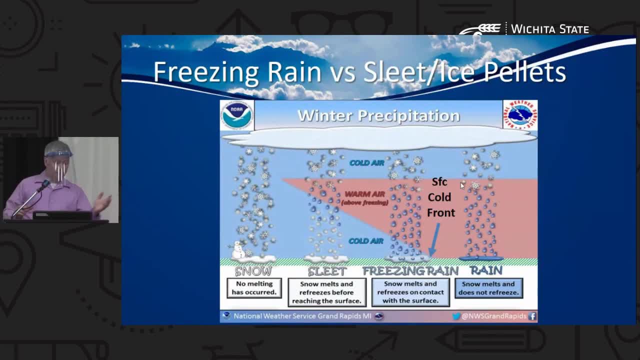 become just all snow And that's as that. that uh cold front is moving through the area. Uh, it's moving through slow enough that you're getting those changing precipitations Now, if you have a case where your warm air- in quotation marks- is actually still. 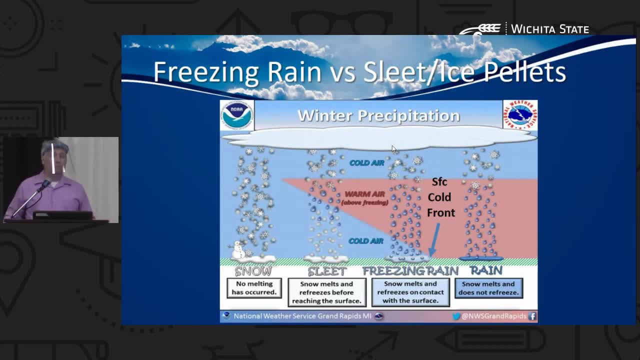 about, uh, you know, maybe a little bit above freezing. well, you don't have. you don't at that point have such an extreme change in temperature that you're going to get that freezing rain. That's why you're not always going to have freezing rain when you have a cold front come. 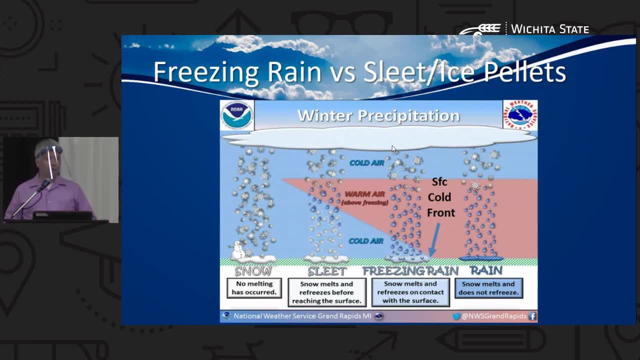 through during the winter months. It's only when you have kind of warm weather at your location that's then being suddenly displaced by uh cold air That's below, uh freezing at a location that you kind of get that, that that warm air that's. 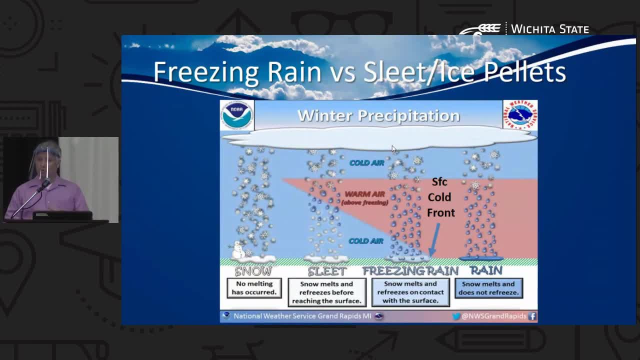 trapped in the middle. uh, that melts your, your snow back into water and then starts to freeze back into snow as it gets close to the surface. Uh, as that warm air starts being pushed out of the area. again, that warm air is higher up. 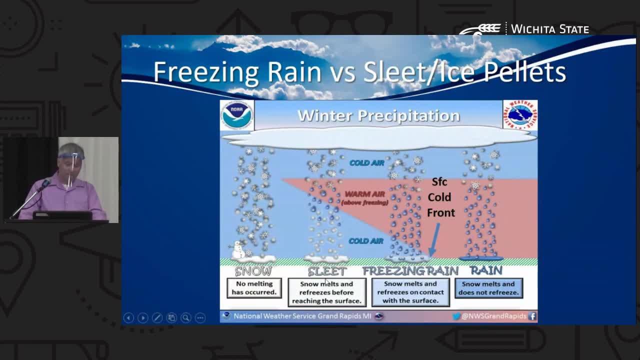 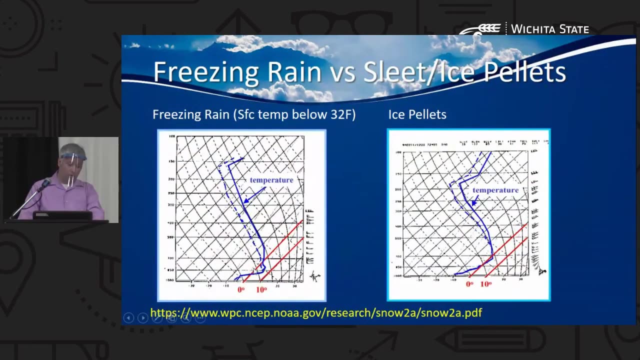 And the cold air near the surface gets thicker, which leads to the refreezing as it falls through that cold air, And so you get those little ice pellets or sleet hitting at the ground, And so again we can look at this and see it kind of graphically- where that freezing rain. 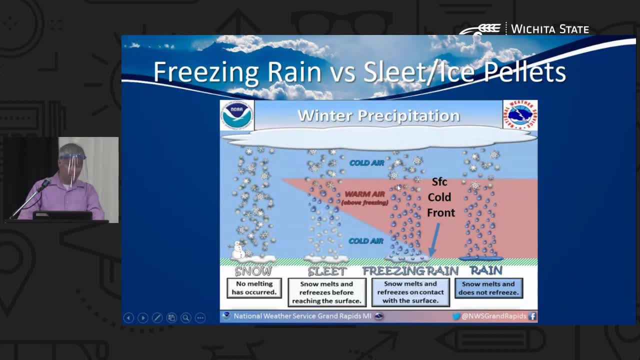 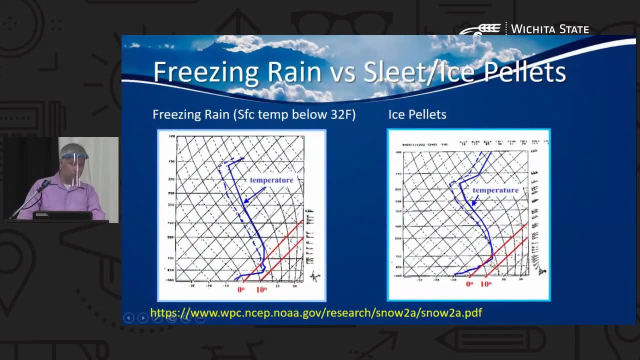 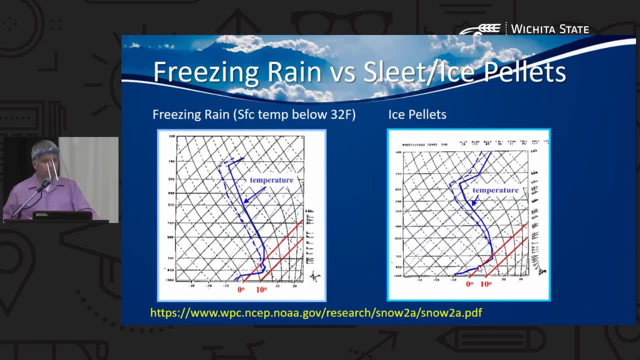 The question was about, um- and I'm going to kind of rephrase it a little bit- If is there any sort of heat island type of effect as a system moves into like a metropolitan area, uh, like Wichita, uh, does that influence the, the precipitation? 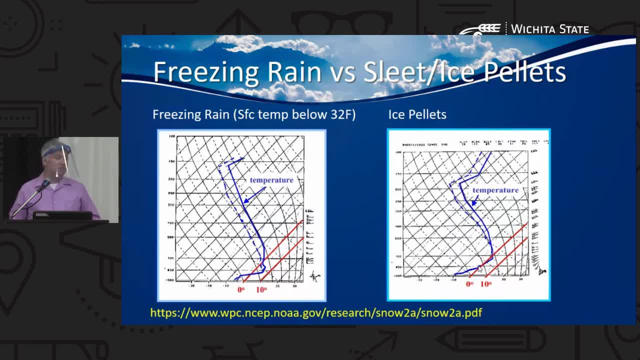 and how it falls. Uh, yes, it, it. it would have some impact. uh, potentially, Um, is it a huge impact? Not necessarily, Uh, but uh, there's definitely the the potential for some enhancement. 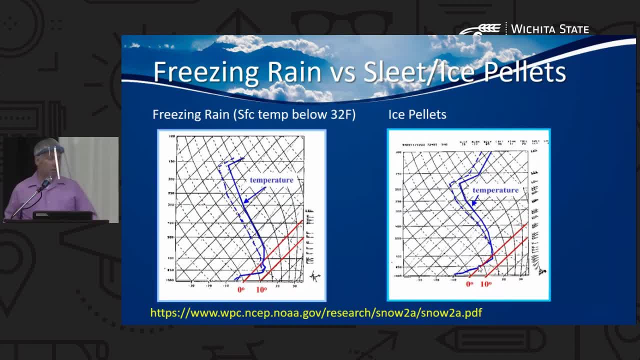 um, of what would happen, And so, yeah, I mean that that's definitely another uh uh wrinkle, uh, that that that can occur. Anything else, Yeah, Oh, the dashed lines, Um, that's actually humidity, I think on this one. 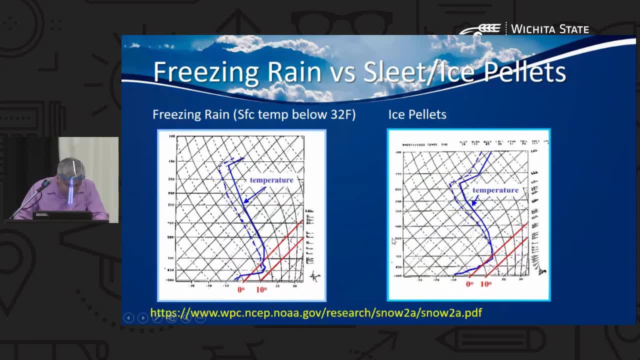 Trying to. well, no, no, Cause the humidity would go the other direction on here. I'm not. what's that? Yeah, The dashed lines. Uh, let's see here. So that's, that's my temperature, Let's see. 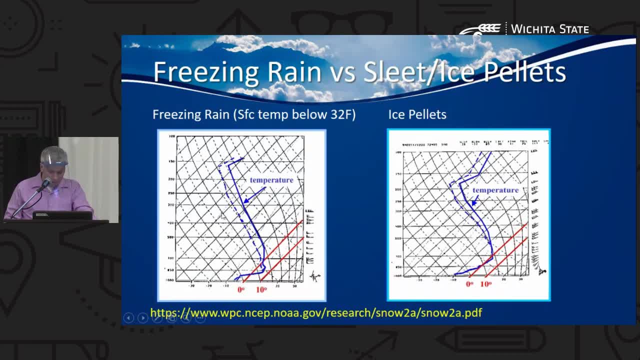 Is that my adiabatic line? That might be the adiabatic line Um, which that's used with um, uh, basically, you trace up um, trying to trying to explain this without getting too far down a rabbit hole. As I alluded to, these charts are also used. 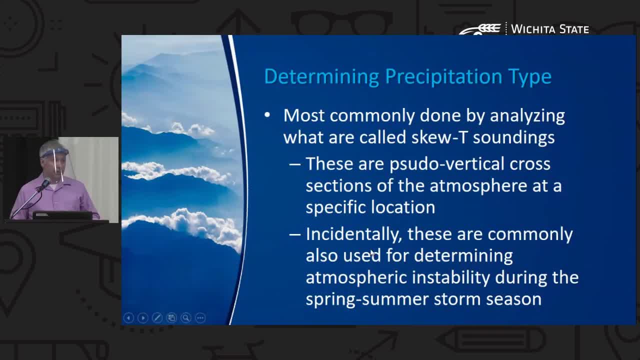 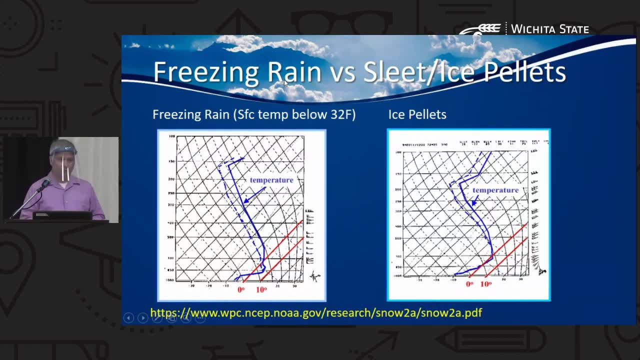 when trying to determine atmospheric instability. And so you know, before we had some of the computing powers and things like that that we have today, all of this would be just done by meteorologists by hand. And so you have, the atmosphere will cool at what's called the wet. 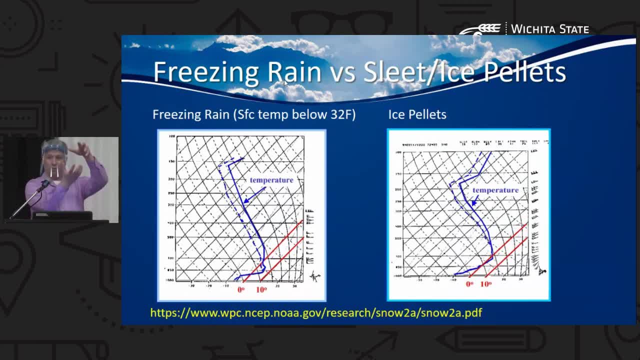 adiabatic rate as a parcel of air goes up in the atmosphere And it will cool at that rate until it's fully saturated And then it moves at or, I'm sorry, it pushes up at the dry adiabatic rate. 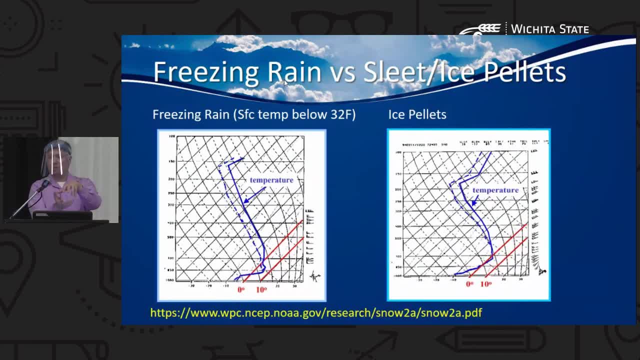 until the parcel of air is saturated. And as soon as it hits that saturated temperature, then it just moves up at the wet adiabatic rate in terms of cooling, And then it always comes down at the dry adiabatic rate. And so this is. 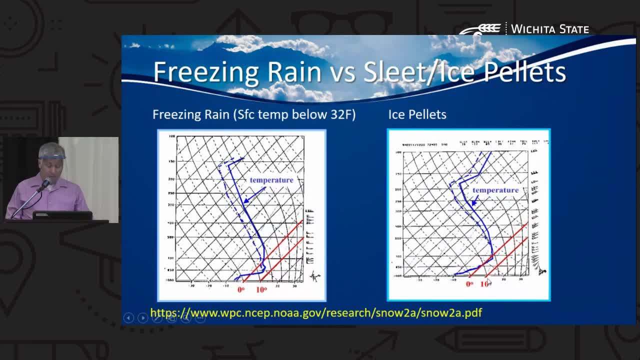 these are our dry adiabats. I'm almost 100% sure that's what they are In this case. I don't have them. They're not labeled on here. But basically, you trace up your cold line, you're dry, and then you come down this line and where certain things cross, gives you the area of 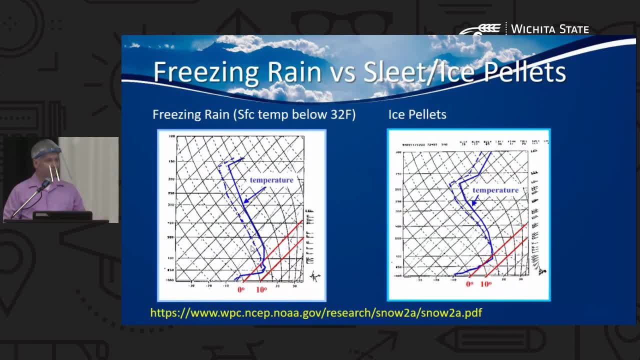 instability on your skew teeth. basically, Without diving too deep, that's what's going on. You hash out during the severe weather season on it, where this area, where your adiabats cross and then that kind of grass graphically shows, okay, there's a lot of instability at this point. 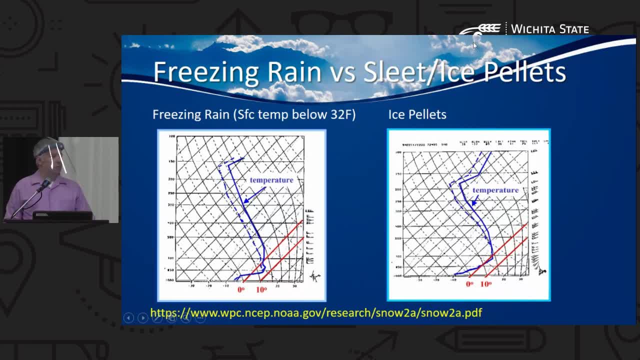 Although these days the computers typically do all of that work for us. But yeah, if you were to look up sounding, I wish I had a good sight off the top of my head. but you can look up some soundings and they will actually show the calculated area of instability and where that. 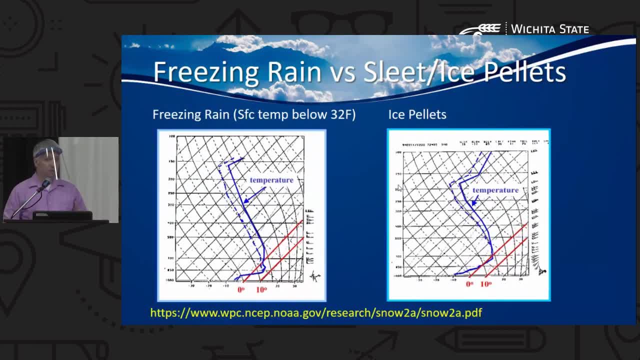 layer is in the atmosphere And again during severe weather, you can see that there's a lot of instability in the atmosphere. But yeah, if you were to look up sounding, I wish I had a good sight off the top of my head. 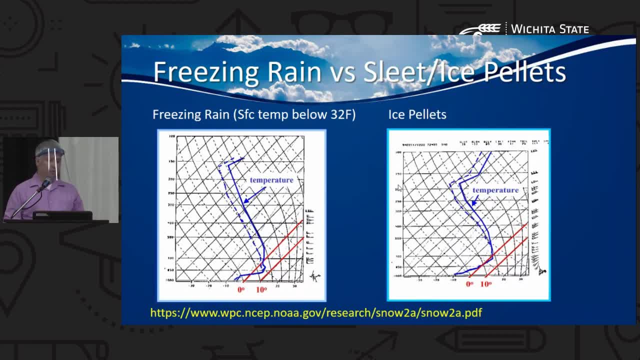 But yeah, if you were to look up sounding, I wish I had a good sight off the top of my head. that really helps us in terms of having a better feel, for if a parcel of air is pushed into this area, then there's going to be explosive vertical development. It's not as much of an issue during. 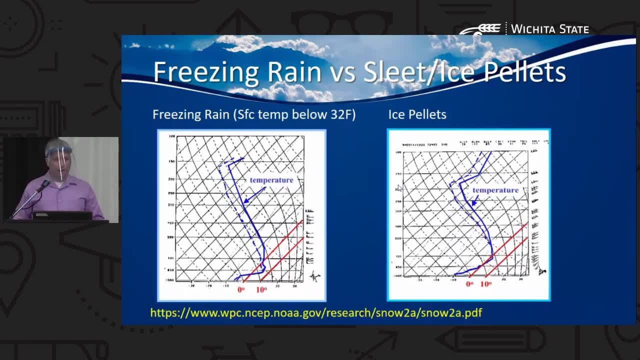 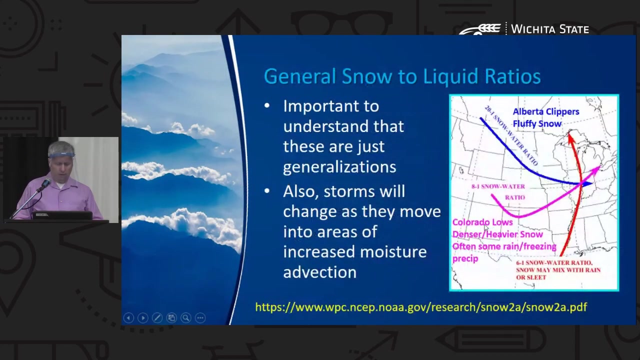 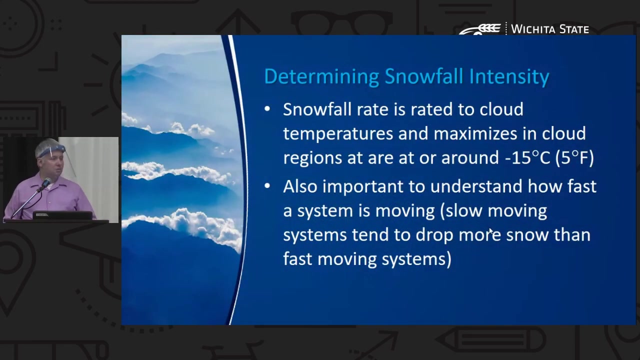 the winter months, because the atmosphere is a little bit more stable, But during the summer months. that's what's going on And those lines are how we basically help visualize on the graphic where instability is. Hopefully that was somewhat clear. Anything else? Okay, Okay, yeah. So we've got to figure out, not just 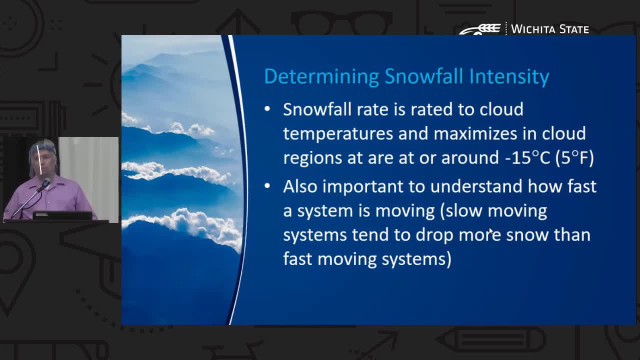 what's falling out of the atmosphere, but how hard it's falling out of the atmosphere, And part of that is in determining how much frozen precip is being developed in the cloud And, depending on the temperature, depends on how much actual precipitation is being formed within the clouds. 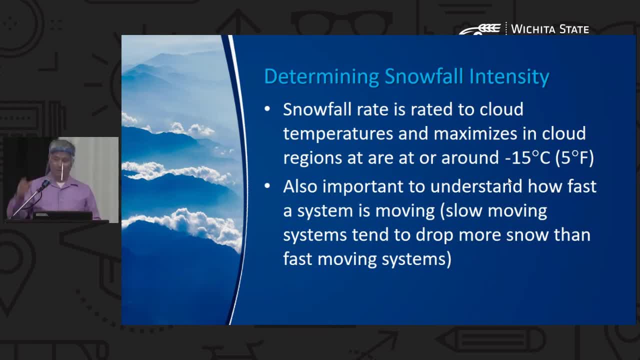 And it's it's sort of a curve that, in terms of how much is being formed, based upon what temperature it is. The maximum precipitation is being formed around five degrees Fahrenheit or minus 15 Celsius And, depending on the temperature, depends on how much actual precipitation is being formed within the clouds, And it's it's sort of a curve that, in terms of how much is being formed, based upon what temperature it is. 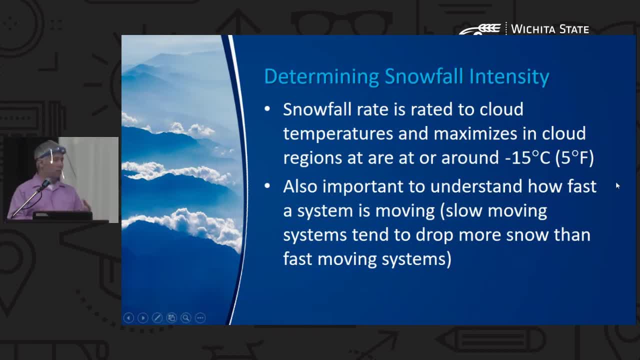 And, depending on the temperature, depends on how much actual precipitation is being formed within the clouds, And it's it's sort of a curve that in terms of how much is being formed, based upon what temperature it is, And and based upon that we kind of know, and this is where the models do help us out. 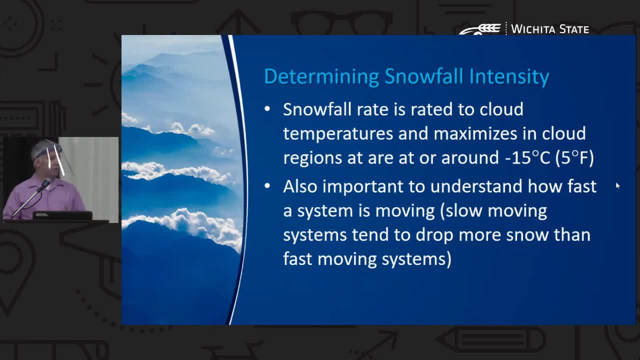 in terms of understanding how much liquid equivalent is being formed within the cloud, based upon what the cloud temperatures are at a specific point and kind of how thick that area is. It's also kind of important for us in terms of understanding the intensity and how fast the system is moving through the area. 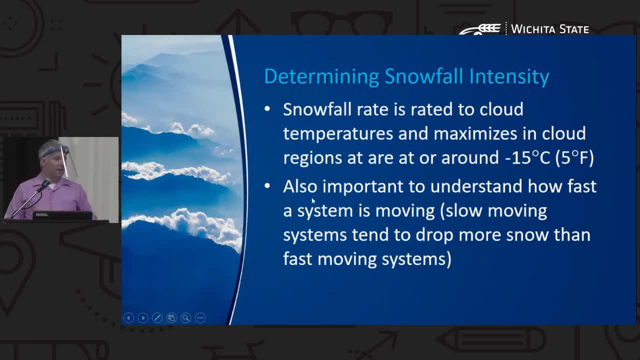 if it's moving really fast across an area, by the time the snowfall starts to kind of pick up at your area, it's already out of the area, so it winds up not being as intense, whereas- and you know, we see this actually probably seen most intensely across the Great Lakes region because of all the 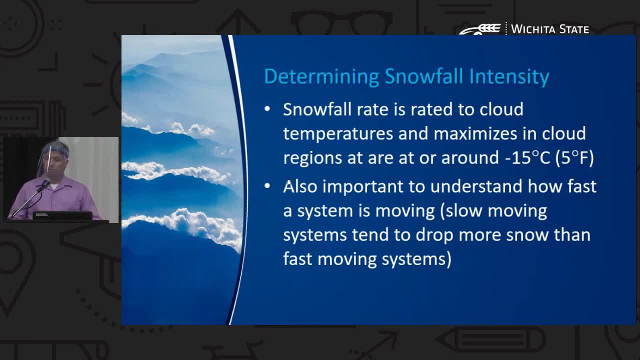 moisture that gets picked up off the lakes. but you'll get into these snow band regions and perhaps most notably is Buffalo, New York, which is right on the lake. the fetch of the lake is such across Lake Erie that it picks up all sorts of moisture as a system. 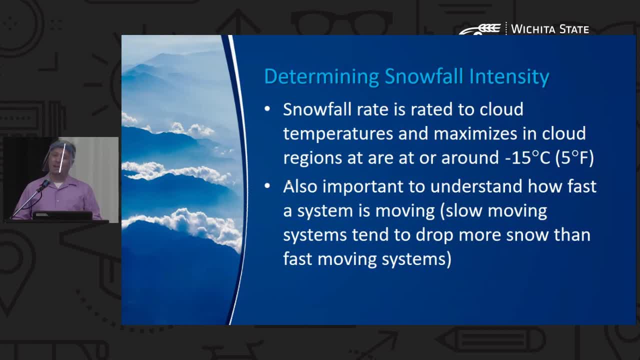 blows across the lake and, as a result, all that moisture gets dropped as soon as it gets to land, and that's why Buffalo, New York, is very notable for very heavy snowfall, because you get these bands of snow that just stay over that area because of the way the winds. 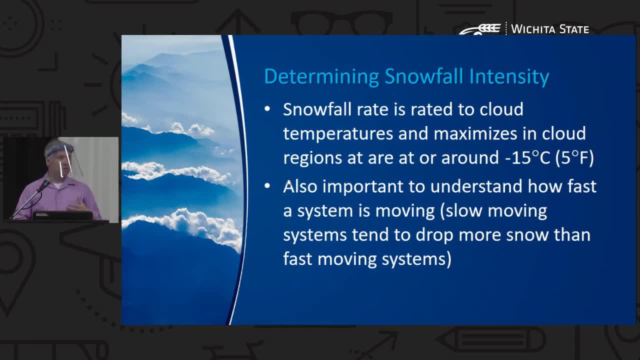 are blowing. so understanding where those snow bands are going to set up- whether you're in the Great Lakes region, where it's a little bit more predictable, or you're here in an area that doesn't necessarily have as much lake influence is is- is really important to note. you know, in this part of the the country most of those bands are going. 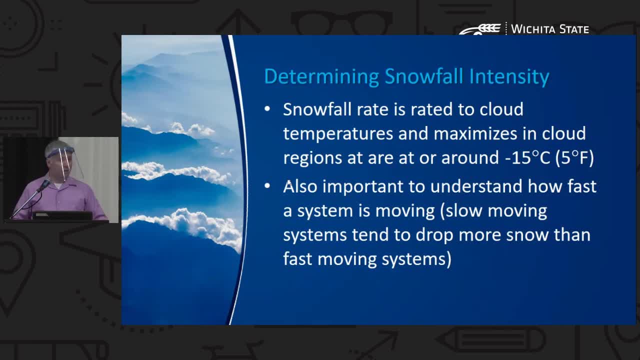 to be set up along the cold front, but depending on how fast that cold front's moving, you may just get stuck within one of those bands for a long time and you may be getting an additional two, three inches of snow. but your buddy a few miles away wasn't stuck in that band of snow and gets almost. 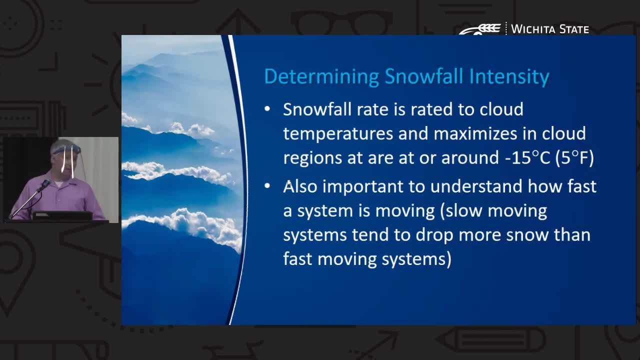 nothing. so again, this, the complexity of it could- really the fact that different locations can get radically different amounts of snow depending on where they are relative to the snow band at a specific time, is again what makes things really complex for us as meteorologists and why it is very difficult for 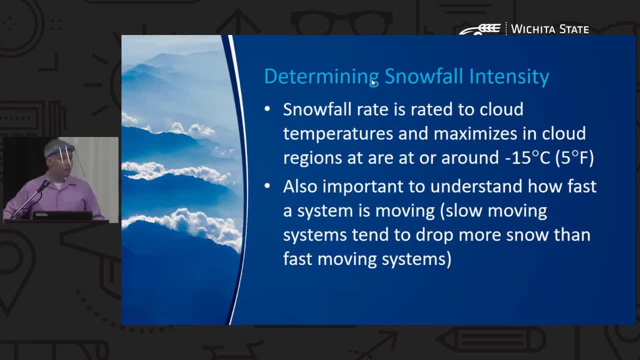 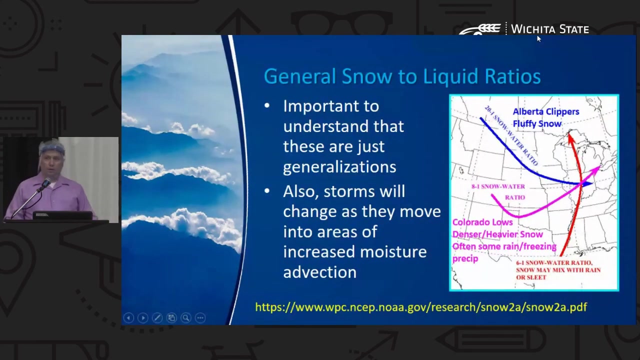 us to not just give like a two or three or maybe even sometimes more than that inch forecast over a period of time for an area, because no two areas are necessarily going to be alike, depending on where the bands of snow line up over time. so one of the things I alluded to earlier was 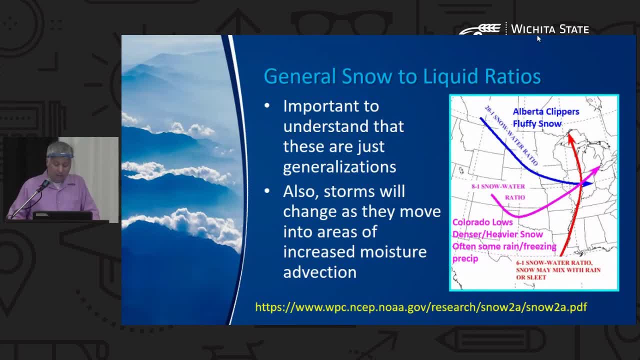 it kind of depends on the density of the snow that's coming out of the sky. and if we've got one of those continental polar air masses, well those are going to be a good example of the kind of density of the snow that's coming out of the sky. and if we've got one of those continental polar air, 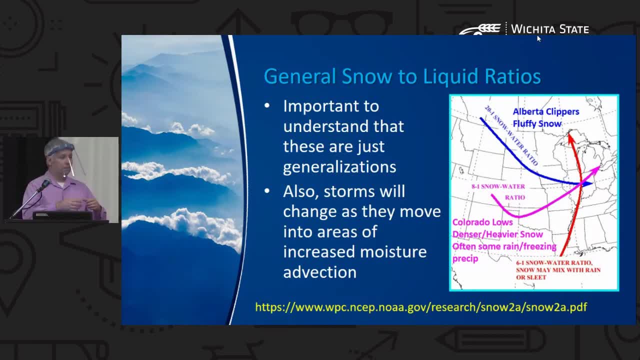 masses. well, those are designed for when you're in the middle of a winter season, so maybe snow is going to be the most possible- are forming over the. those systems are forming over land primarily, and they're not getting nearly as much moisture enhancement into the system. well, if 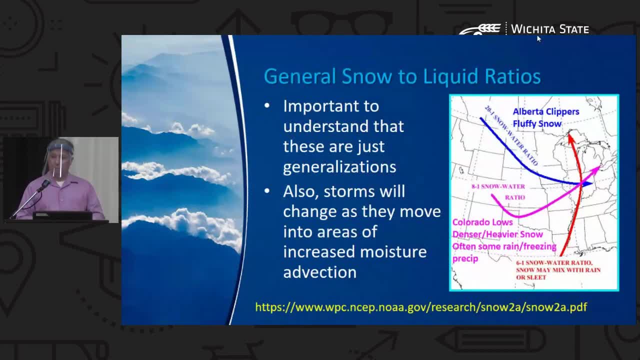 that's the case, then the precipitation, the snow is much less dense, it's a lot fluffier, and so, as it falls, it's going to pile up more. so if I'm uh, you know, forecasting a low that's coming out of, you know, Alberta, Canada, uh, it doesn't have, uh, a lot of moisture content. 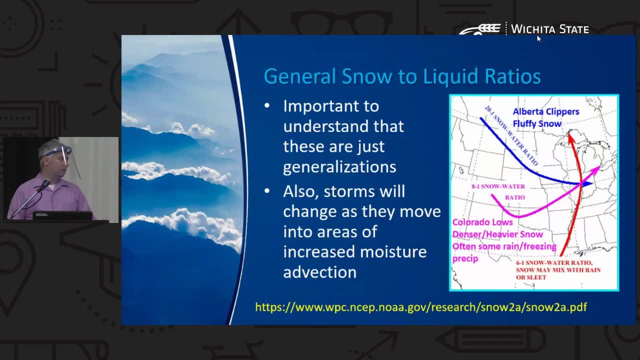 whatever moisture that does fall is going to- uh, you know, pile up quite a bit and so, um, the ratio kind of in more, more of the extreme cases is about a 20 to 1 ratio of water to snow. what that means is that one inch of rain would be the equivalent of 20 inches of snow piling up at a location. 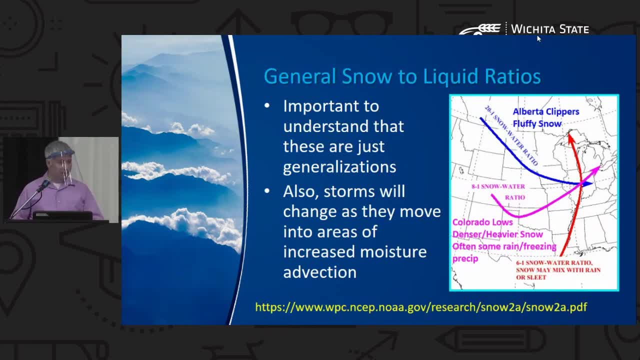 um, and again, that's kind of an extreme case. on the flip side, if you have one of these very, very moisture, you know, warmer kind of low pressure systems coming up, um, you know, if you have one of these very, very moisture, you know warmer kind of low pressure systems coming up, 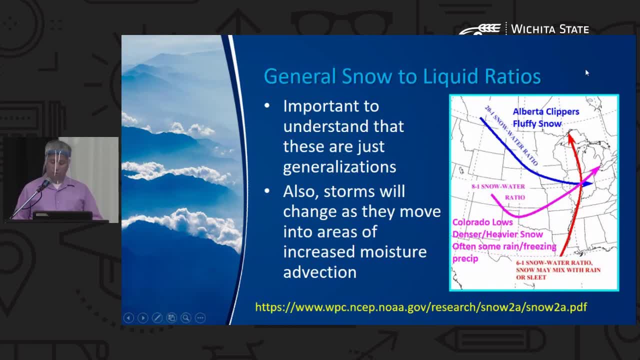 off of- in this case it's kind of this arrow, sort of drawn off of the Gulf of Mexico. uh, your precipitation is going to be a lot more dense and that one inch of rain is maybe, you know, five to eight inches of snow, depending on your location. so this is why, usually the starting point for for us. 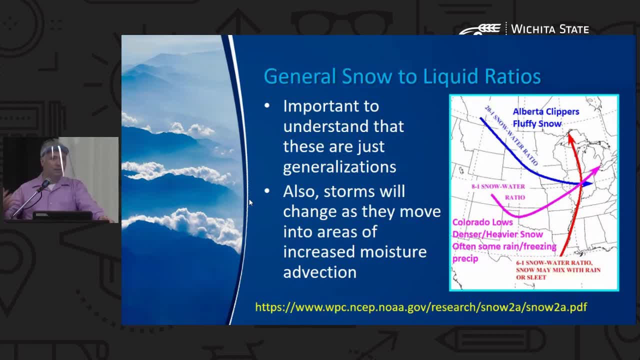 as meteorologists, when we're kind of trying to convert the liquid that we think is going to fall out of the sky at a certain location, we typically start at the, at about a 10 to 1 ratio, and that kind of gives us kind of the middle middle range of probably what that conversion is going to be, and so we'll look. 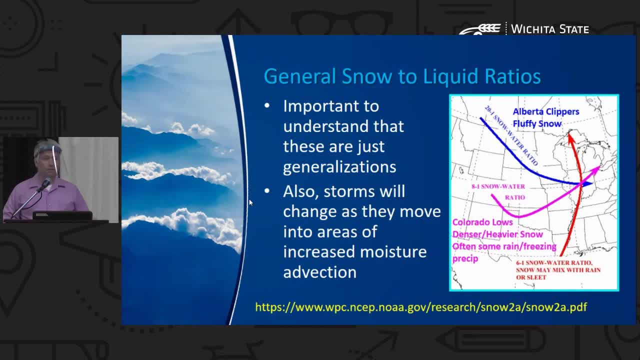 at the um water equivalent on the, the numerical models kind of combine that with our own general feel on the, the system, and that's where we start developing. okay, I know it's going to be cold at the surface. I know this is coming down as most or all. 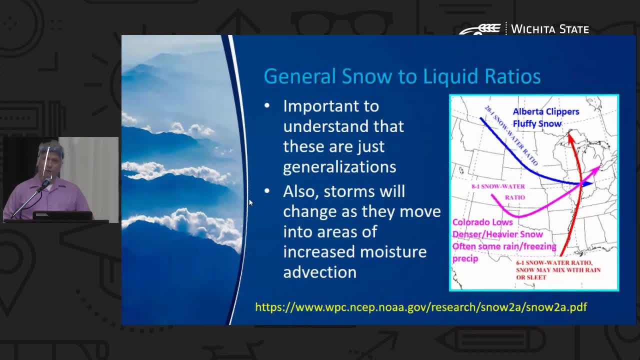 snow. so if I'm seeing about a water equivalent of points you know, 0.5, about a half an inch of what would be rain falling in Wichita, Kansas, and I'm going to go with about a two, just you know, maybe a three to six inches of snowfall as that system comes across. uh, and so that's, that's sort of what. 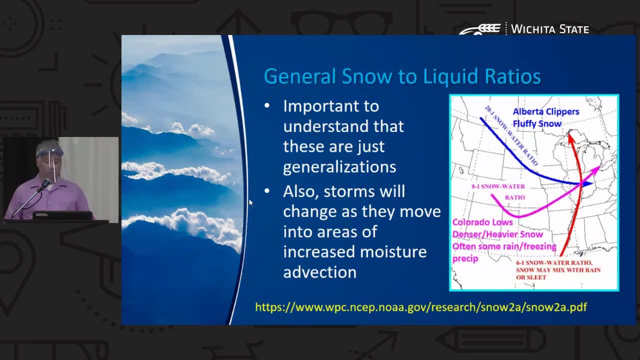 where the the thought process tends to go. uh, as we, we evaluate these systems. but, of course, just because the model has said at one point that it's a half an inch of water that's in this system, uh, if it's picking up a bunch of moisture off the Gulf of Mexico, that half an inch? 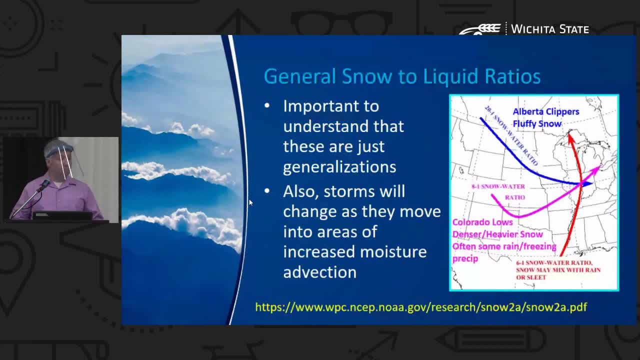 of water can quickly become a full inch of water and then suddenly we have a much heavier snowfall event, uh, in Kansas. so we're having to take in all of that, that information, as we're trying to come up with a forecast, and that's just kind of. 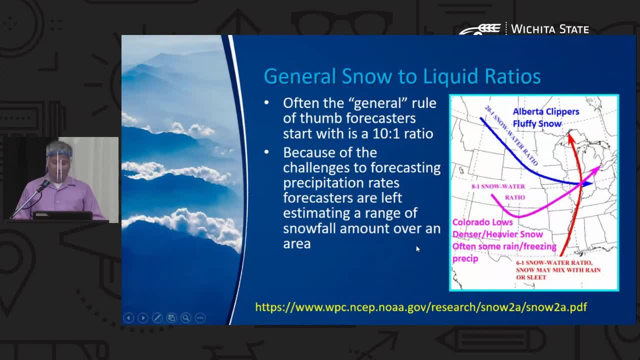 talking about my 10 to 1 ratio and- and this is, you know, all of these little bits of information- how quickly the precipitation is going to go from rain to snow. it's a huge issue and, uh, you know, all of these little bits and pieces uh really impact what our perception is going to wind up being of. 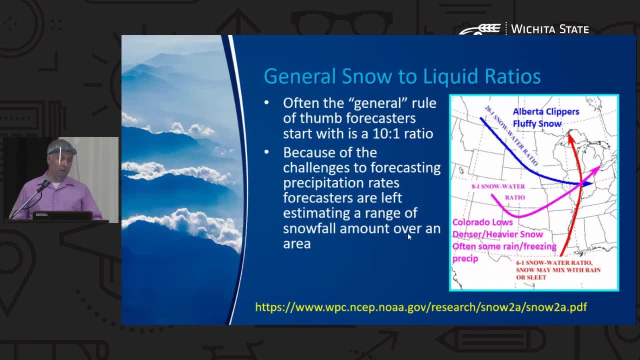 the uh amount of uh precipitations that's going to fall at a location. plus, on top of all of that, if you get that, for example, some rain out ahead of the system and then it turns fairly quickly to snow, well, you just had rain falling on a on the ground and that rain is, you know, warm the surface of the. 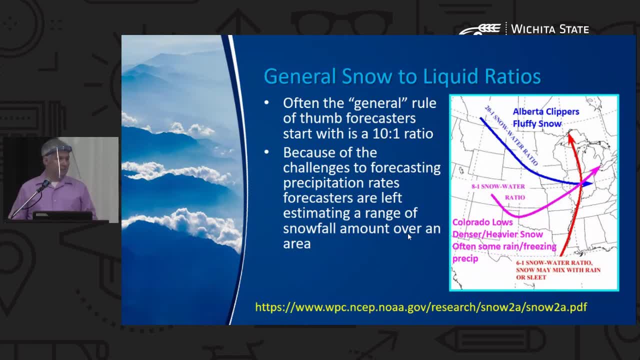 earth up a little bit and then your Snow's falling and melting. so we may have said two to four inches, but that Rain melted some of that first set of snow and so doing that accumulation at the surface becomes even more complex. because, yeah, you were right about. 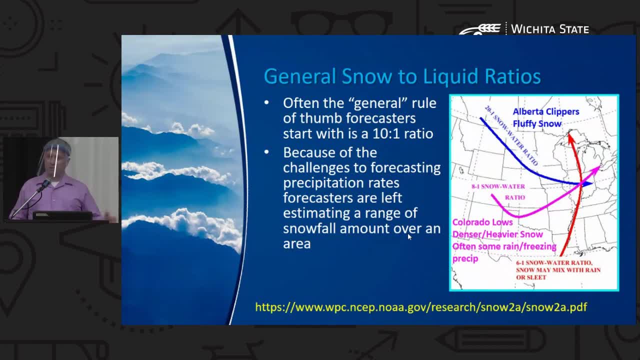 amount of snow that fell, but the first bit of snow didn't stick to the ground, It melted right off, And so these are all reasons, excuses maybe- for why those snow depth and snow accumulation forecasts that you heard may have been incorrect from your meteorologists. It's not that they. 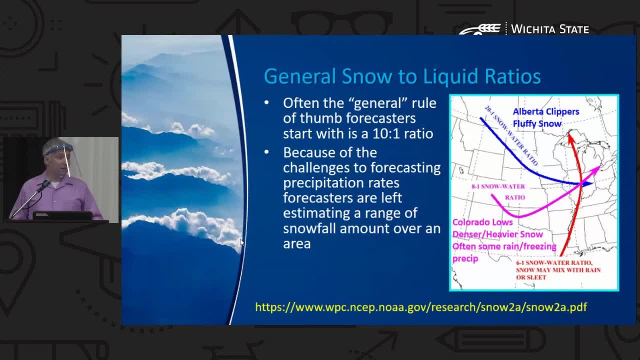 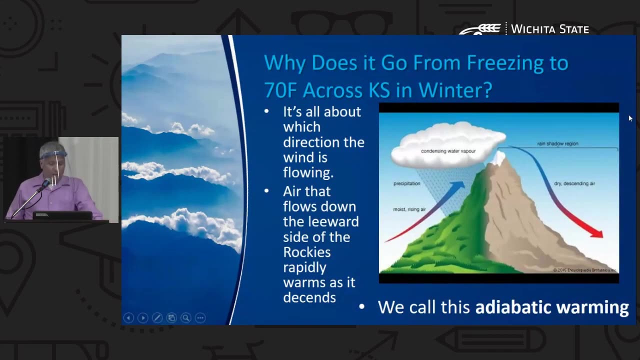 were stupid about what they were doing. It's that, you know, a lot of these little bits and pieces can be very unpredictable, and a little change can make a huge difference in what actually winds up occurring. A little bit of a sidebar here, something that we will observe, at least once. 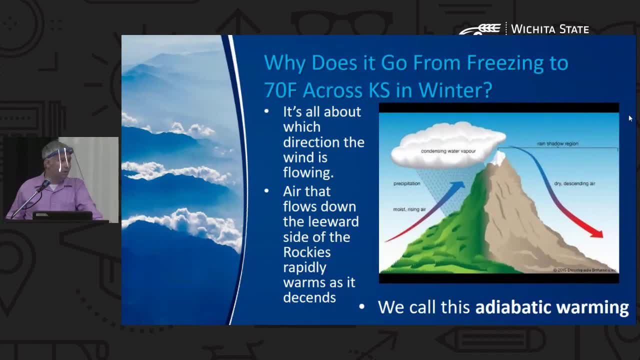 most winters here across the Central Plains is where we've had a system go through. it dumped you know five inches of rain or five inches of snow on us, and then the kids all race out to the little little hills and things like that and go sledding for about a day or two and then suddenly it's all. 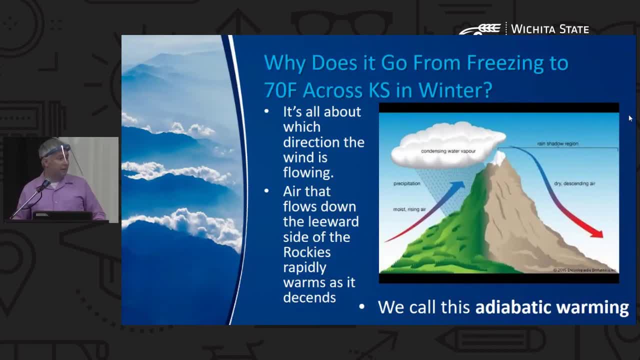 gone because the temperatures went way back above freezing again and we just say, oh yeah, crazy Kansas weather, right? Well, there is something that's going on. It is related to the topography across the center part of the US, center and western part of the US, and I talked a little. 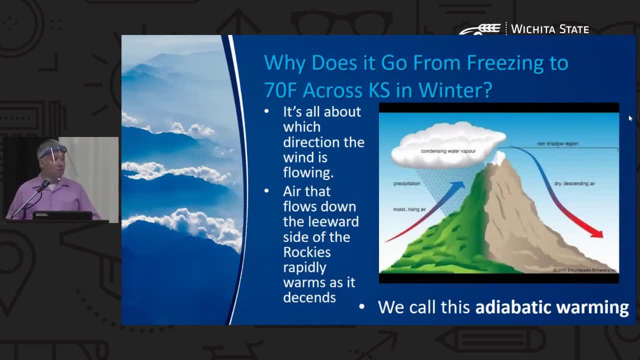 bit about the adiabats and adiabatic heating cooling when we were fielding the question about the soundings. Basically, as air is pushed- oh my gosh- as air is pushed up and over the mountains, and in the case of here in the Central Plains, this would be the Rocky Mountains. 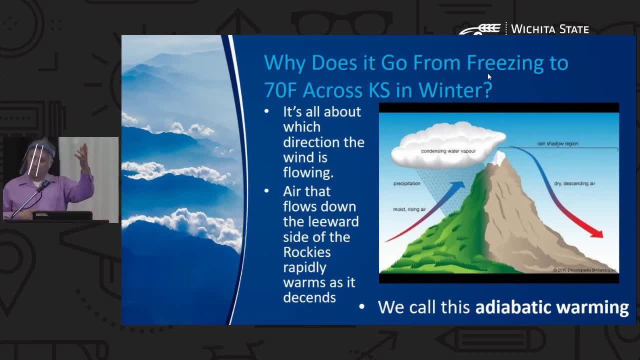 it cools as it goes up the windward side of the mountain and precipitates out, dries out that air mass, So that then on the back side it starts. that same air warms up as it goes, comes down toward the earth. That's because the rate at which the air as it pushes up one side of the mountain, 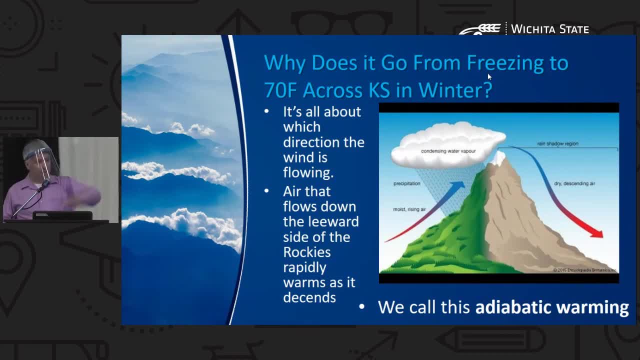 cools is slower than the amount that it will warm coming down the other side of the mountains. So that's what leads to this: On here, it's specifically showing a rain shadow. So if you're on the- This is why, for example, Seattle very wet city, Well, you've got the Willamette Mountains and 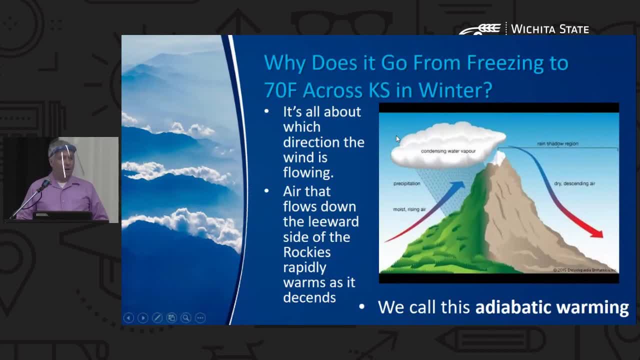 things like that, the northern part of the Rockies there- and it's on the wet side of those Rockies If you go across the state- precipitation is much, much less, and that's because they're in the rain shadow of the mountains, But the weather is also much warmer as well, And so, as a low 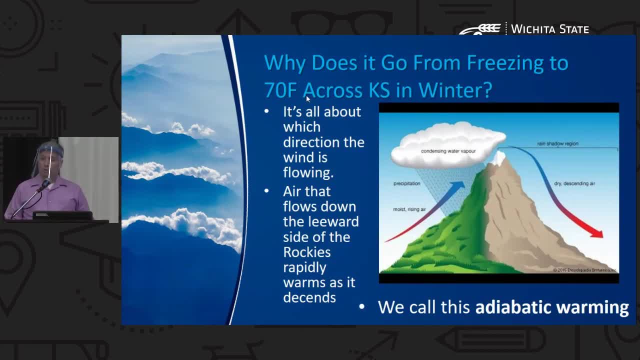 pressure system pushes through the area. we've talked about how the winds blow around that low counterclockwise. So once we get to the back side of the low pressure system, it generally brings our winds around from the west. Well, if we get a real strong westerly flow, well then you're. 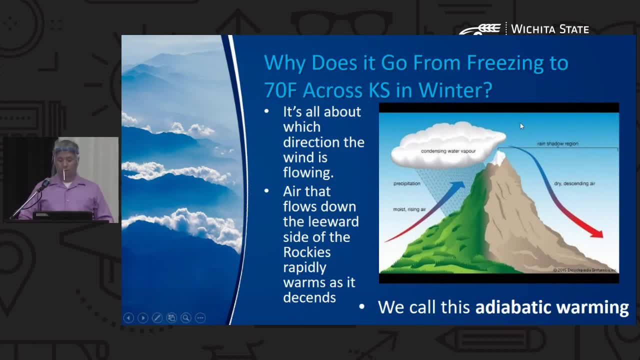 getting this very setup where the air is being blown over the mountain, cooled a little bit but then Then allowed to warm a lot on the back side, And so you get this rapid warming after a day or two, once that low pressure system's passed, And suddenly we're pulling out the short sleeve. 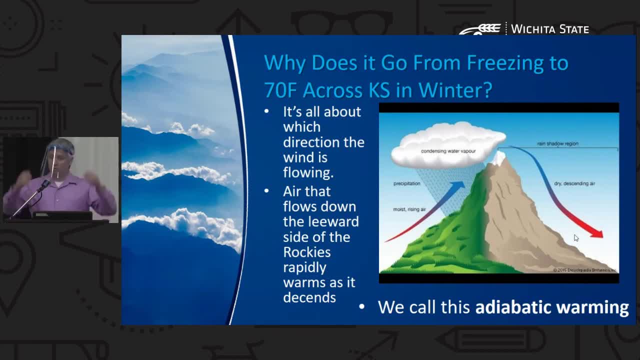 shirts for about a day before the next system comes through and drops the temperatures back off again. So next time you notice that- probably at least for a day or two this coming winter- you'll sort of know what's going on. It's probably because we've got a westerly flow across the 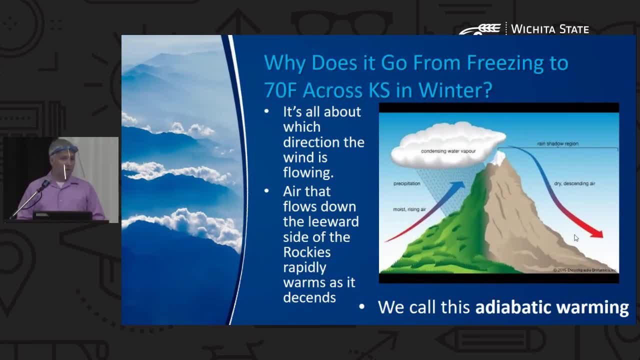 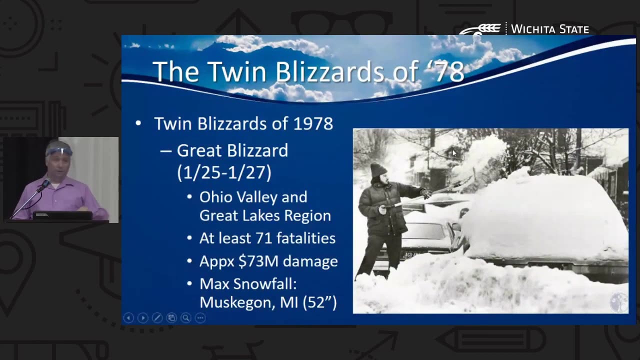 Rockies. It's probably because we're warming up the central plains, And that has, frankly, nothing to do with global warming. It's just the general flow of the winds as they go across the Rockies. So I wanted to kind of finish up with at least one sort of case study of winter weather that has 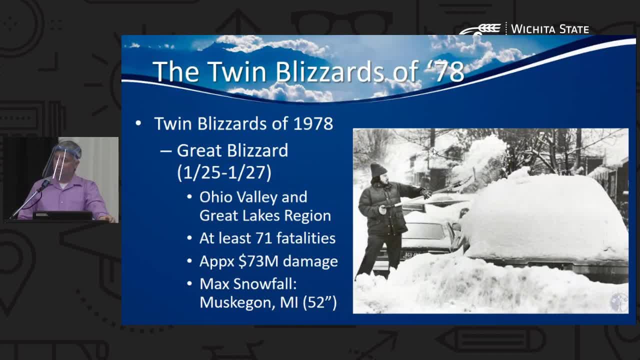 dropped a whole lot of precipitation on really across much of the US, And this is probably one of the more notable storms of the second half of the 20th century, kind of the twin blizzards of 1978.. As for me, I was very comfortable in my mother's womb when this happened and 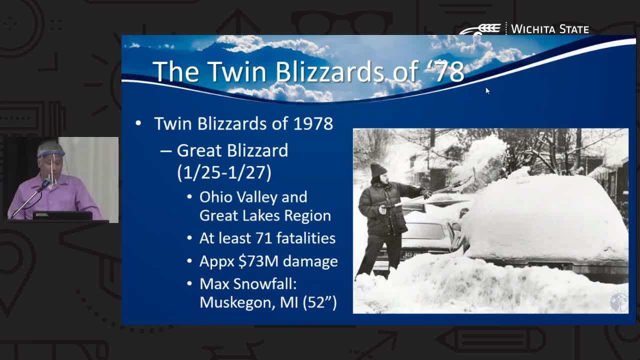 completely unaware of what was going on, But there were two blizzards that kind of converged and happened right around the same time. You've got this first one. that was a huge event across the upper Great Lakes region from, really you know, Wisconsin, Michigan, across, you know, the Ohio. 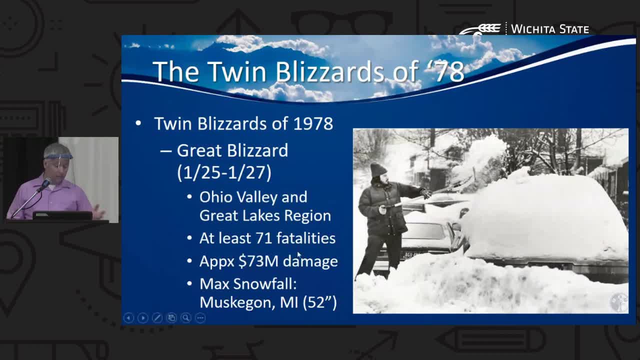 Valley region. that caused, in this case, about seventy three million dollars in damage. This is oddly enough. this is the blizzard that is more notable and more talked about, even though it's the next one of the twin blizzards that really caused a lot more damage and a lot more fatalities. 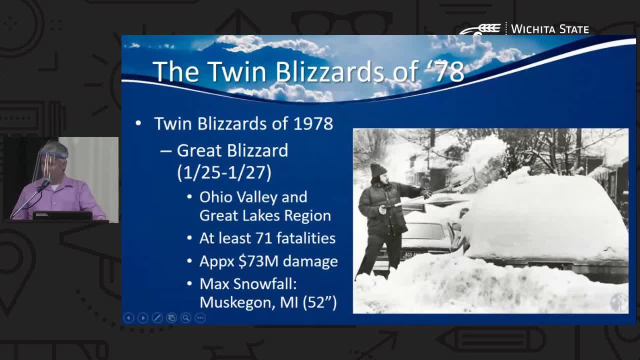 But this one dropped a lot of snow, a lot of thick snow across the area. The maximum snowfall as it came through was 52 inches in Muskegon, Michigan. Muskegon is right along the lake shore. In this case, it just set up a line of snow that just kept falling and falling and 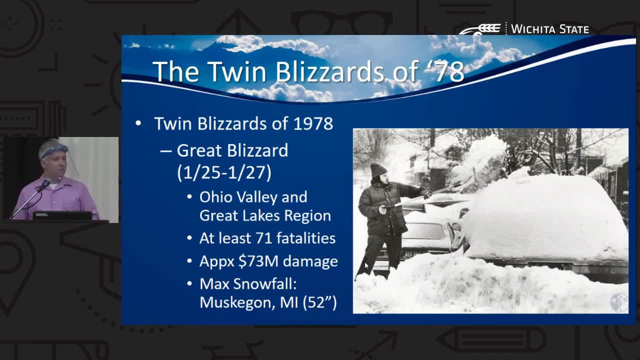 falling because of the fetch again across Lake Michigan. All sorts of warm- relatively warm- water and moisture from the lake was picked up and enhanced the blizzard And it all dropped across the across Michigan and the Ohio Valley region. There was at least 71 fatalities from. 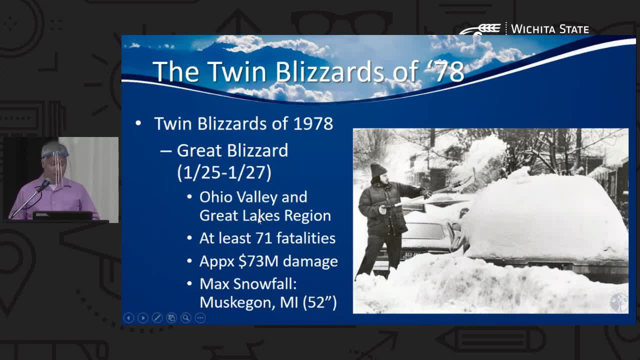 this storm And the area spent the next week and even more than that, just kind of digging out from it. Stories that I heard, that I've heard from my parents, were: you know that you had a lot of roofs that collapsed in across the area because you had three feet of snow. 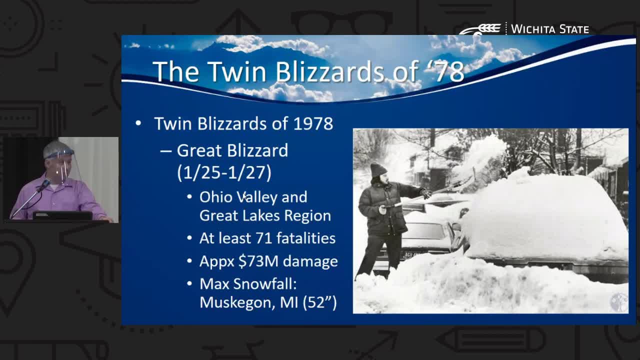 that fell on rooftops and had no chance to melt or anything like that. In this case, it was a system that got enhanced by the Great Lakes and also was getting enhanced with flow up from the Gulf of Mexico, And so all of that, those factors, combined to leading to a very intense storm. 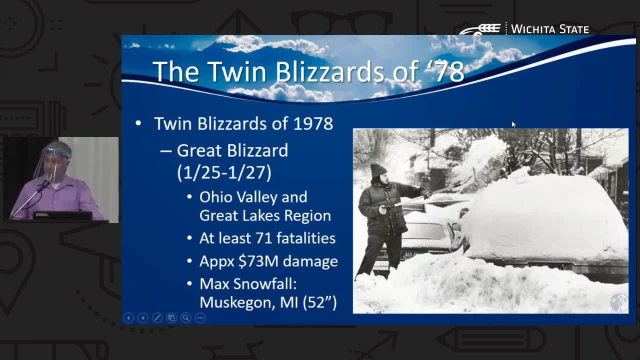 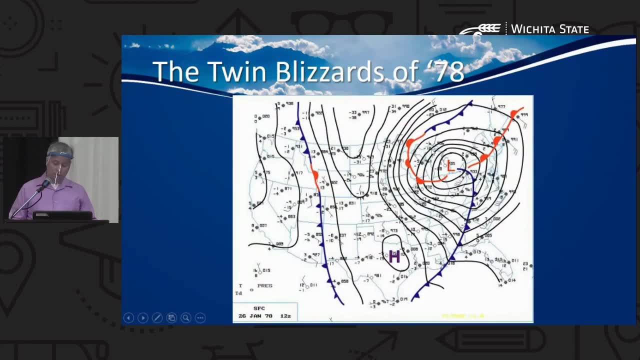 For a couple of days across the Great Lakes And this is kind of a picture of the surface map from that storm as it was coming through And it was really kind of on the back. This is from the 26th. The most intense snowfall was 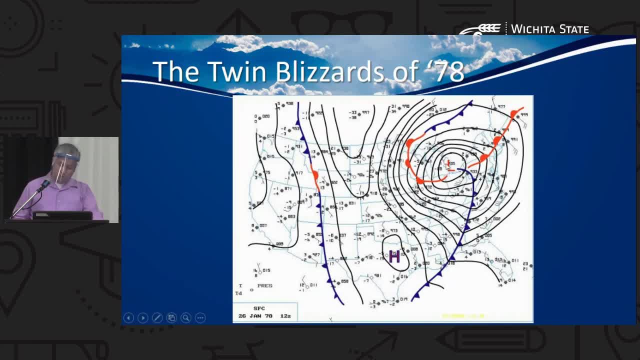 happening from about this time to the next day, when the winds started shifting a little bit further Around and that led to a very high fetch, especially across western Michigan. as you see, the winds coming down around the low crossed a great deal, in this case Lake Michigan, So picked up. 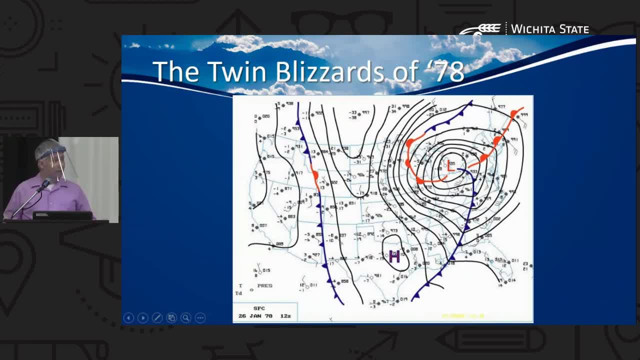 all sorts of relatively warm water again off of Lake Michigan and just dropped it all on Western Michigan. Incidentally, as you go across western Michigan, Descending somos, from the west side of the state to the east side of the state, there's a very wide variance in. 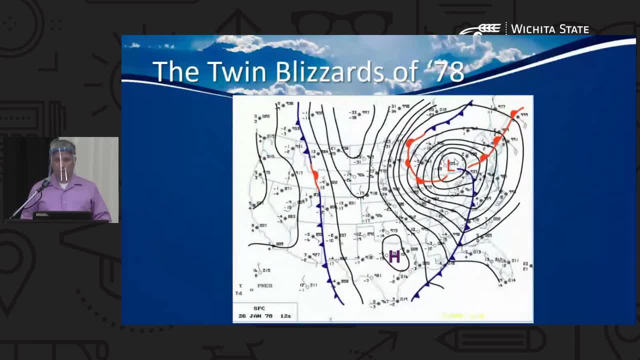 average snowfall over the course of the winter. The heaviest snow in lower Michigan falls to the western part of the state, and the eastern part of the state generally doesn't get nearly as much snow. And then you've got Buffalo, New York, right there. that gets dumped on because 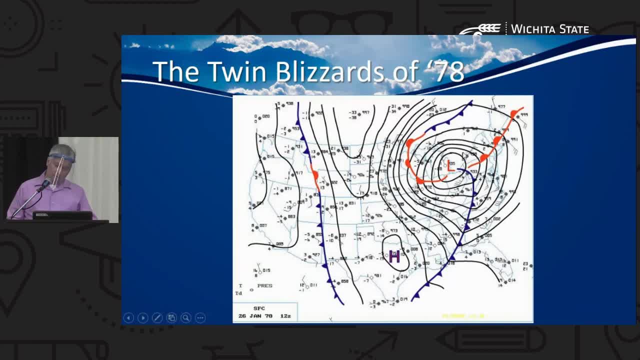 of the flow out kind of in front of the storm that just goes straight across Lake Erie and just drops all that moisture on Buffalo, New York, which is why you hear about Buffalo, New York every year getting a lot of snow. That's what's going on with that. And then lastly, and that's 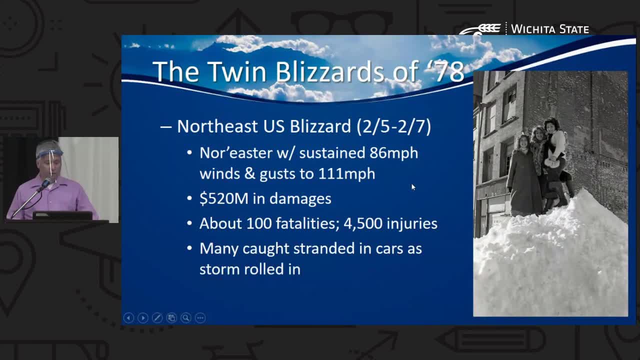 going to drop us pretty perfect. you had the northeast US blizzard, which really was a nor'easter, So we remember kind of where that nor'easter, the Hatteras, low kind of forms, And this was right around just. 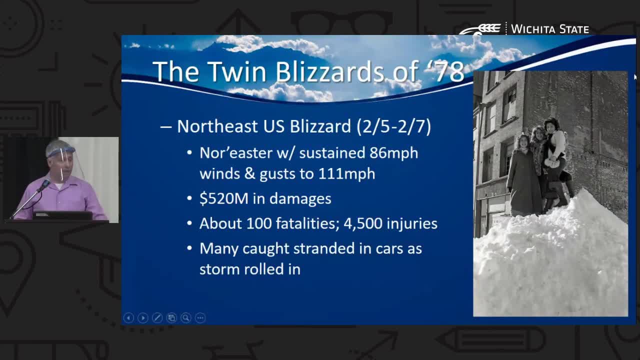 kind of after the first system that came through and was one blizzard. This was coming right up the Atlantic eastern seaboard and, intensifying, had gusts well into the hurricane strength range, which is not uncommon for a nor'easter. In this case it was $520 million in damages, about 100 fatalities, 4,500 injuries, And then 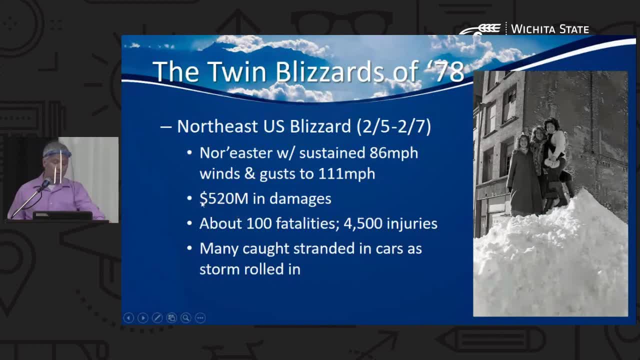 what made this storm as bad as it was is some of the more populous areas, like New York, things like that. It was at its most intense when people are trying to commute And so a lot of people were getting caught in there. So they had to get into their cars and kind of caught off guard with really intense whiteout snowfall. 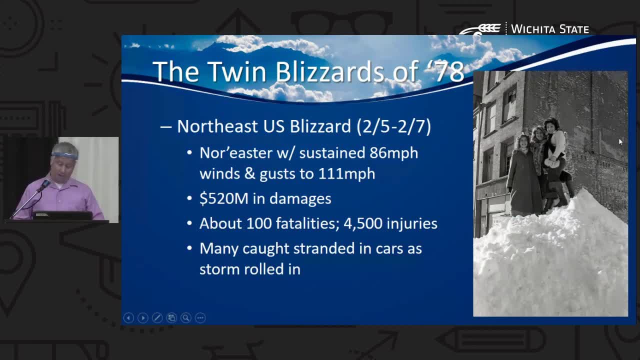 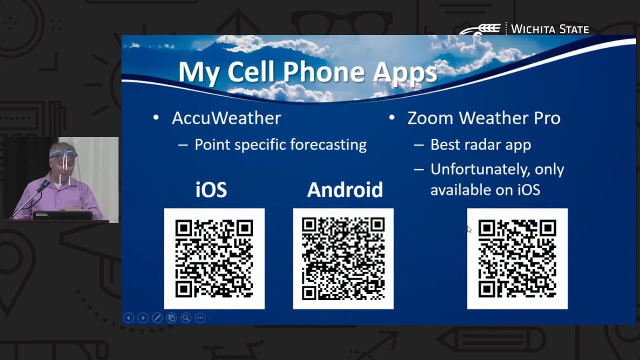 conditions and got stuck and had to be rescued. And yeah, this is a picture of the aftermath. This is a just snow plowed up pile here and a couple people photographed there. Again, this is a kind of the cell phone apps. If you haven't already gotten them in place, you can go ahead and watch that. 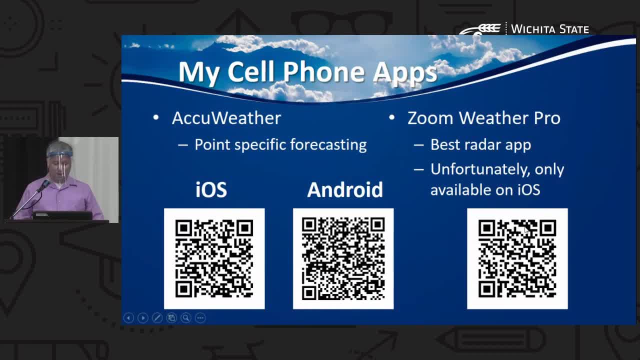 Again, this is a kind of the cell phone apps. If you haven't already gotten them in place, Let me think about that. Hello, Hello, Yeah, Hello and uh, look ahead to next week. next week we're going to talk about uh client a little bit about. 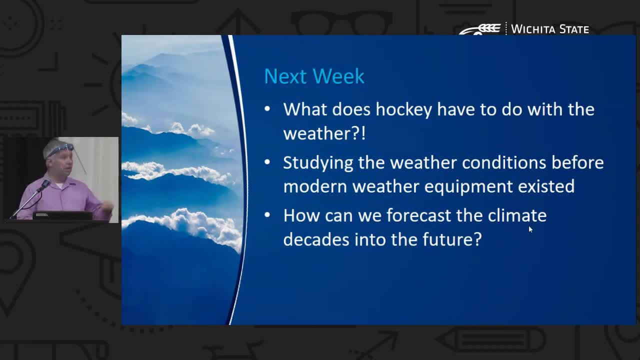 climatology, uh, climate change, climate forecasting, things like that, um, and so what does hockey have to do with the the weather, studying the weather conditions, and how we did that in times before we had our weather equipment, as we uh talked about in the first class, um, our ability to measure our 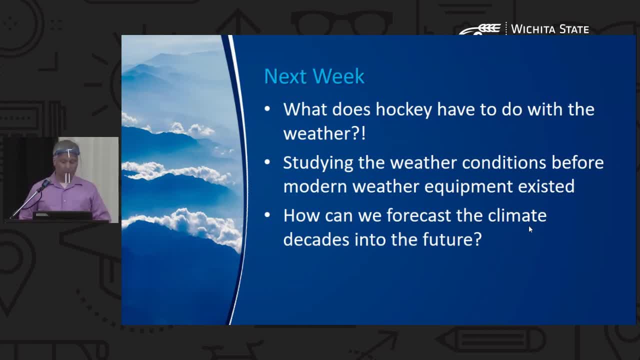 conditions around us is a fairly new thing relative to the existence of humanity. um, so how did we understand, and how do we try to understand, uh, what the weather was like before we could actually measure the weather? and then, how in the world can we forecast climate decades into the?